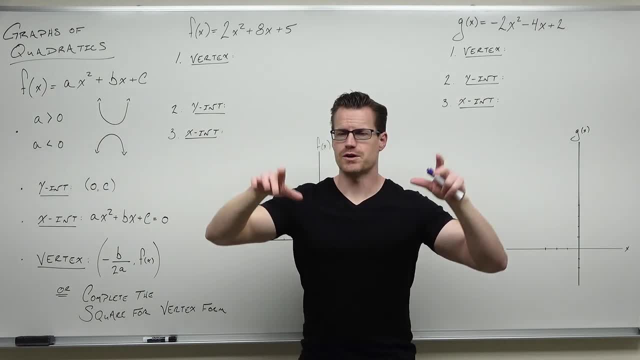 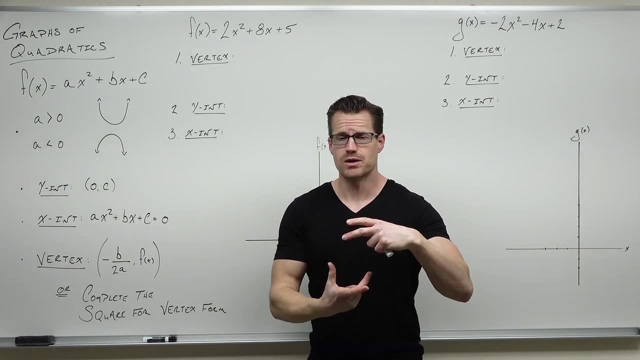 They're going to be what we call upward opening. And if your a, the first coefficient of your x squared term is negative, you're going to get a downward opening parabola. That's where they always look. If a is an absolute value larger than one, we get a vertical stretch. either way, 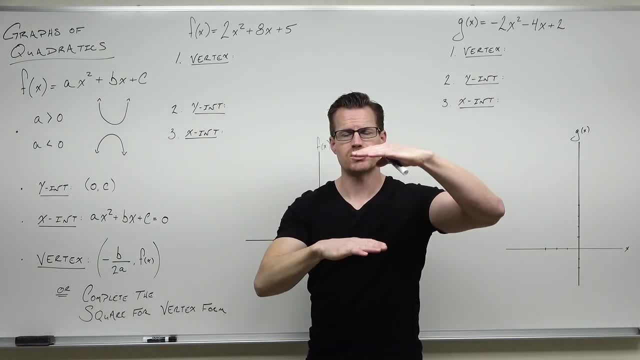 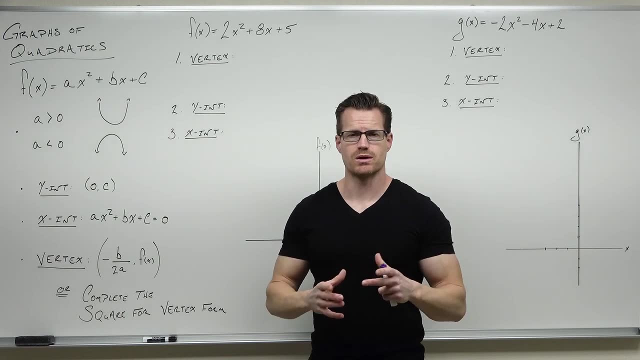 Or if it's absolute value less than one, we get a vertical compression. It'll make the graph look more narrow or more wide respectively, depending on whether your a in absolute value is greater than one or less than one. So we're going to be practicing that and just kind of looking through. 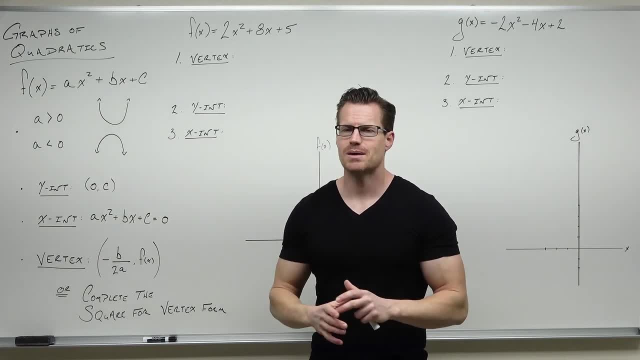 these, Then we need to know how to find the y-intercept and the x-intercepts, And if we want to put this in vertex form- or you're asked for it- how to do that with completing the square. So this is the. 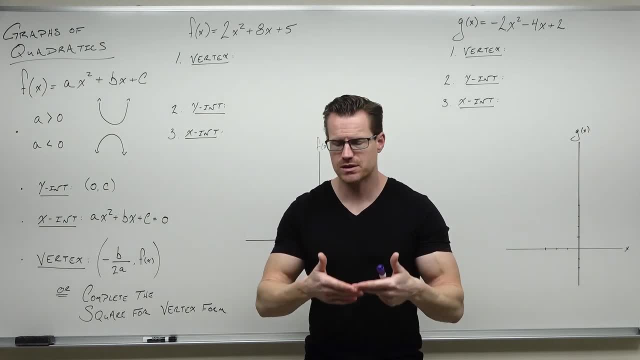 process of going through graph and quadratics. We first determine whether this is going to be an upward opening or downward opening parabola, just like what we talked about. Then we find the y-intercept And the reason why we do those two first: the upward opening or downward opening. 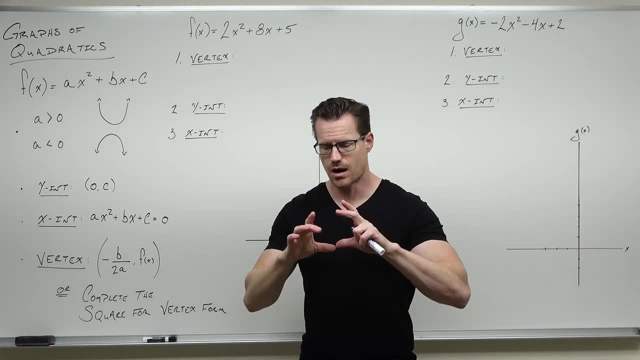 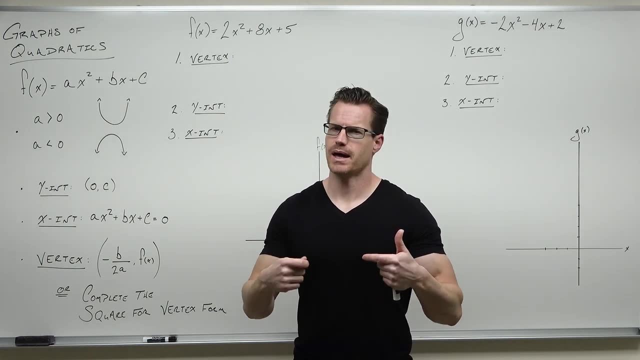 give us a great way to check our work later And in combination with the y-intercept which every parabola has, we can determine if we need x-intercepts. So let me make that very clear to you: Every parabola is going to open, either upward or downward. Every parabola is going to have a 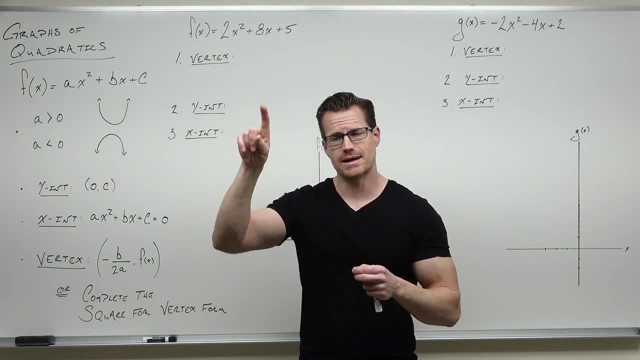 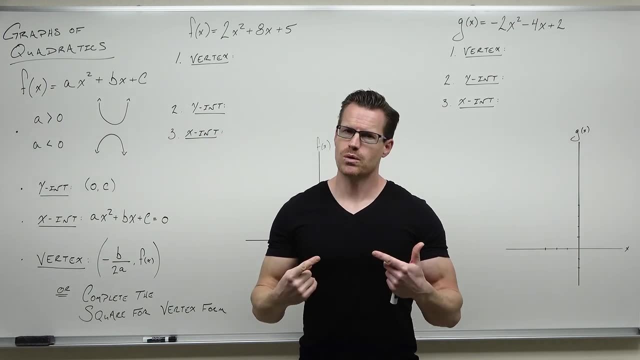 y-intercept. We're going to determine those two things. Every parabola has this vertex where you change from decreasing to increasing or increasing to decreasing. We're going to find that What they don't always have are x-intercepts. If you have an upward opening parabola with a vertex above the. 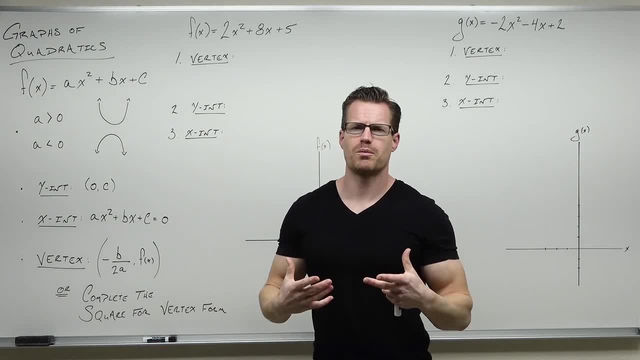 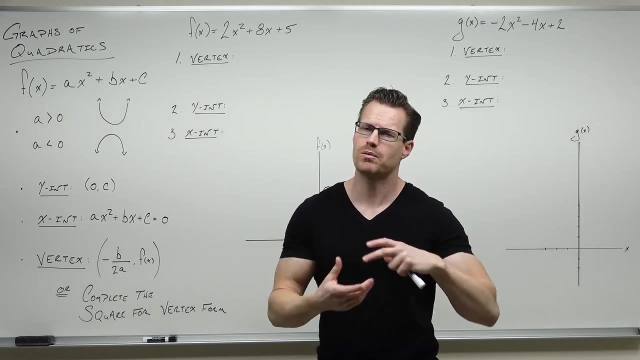 vertex below the x-axis, And so we always go through our parabolas in the following thought process. Number one is an upward or downward opening. Maybe we determine whether it's narrow or wide, depending on whether we have a vertical or a stretch or compression. Then we determine: 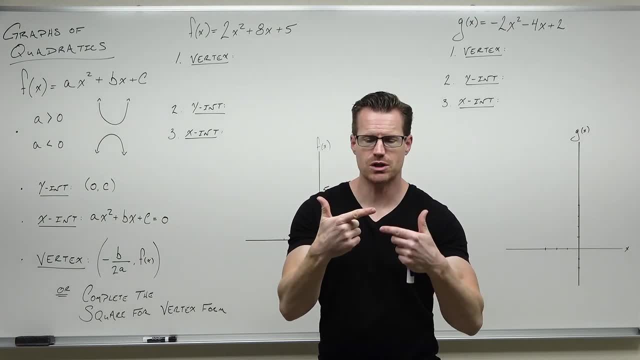 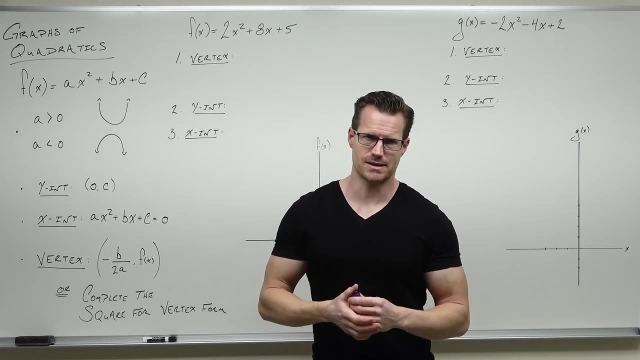 the vertex and the y-intercept. We're going to use the axis of symmetry, to use the y-intercept to give us maybe a free point And then, if we need to, we determine x-intercepts. If not, we're done, And so we're going to go through that. We're going to talk about these. 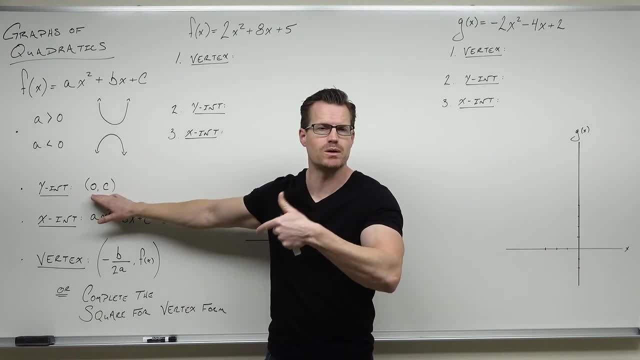 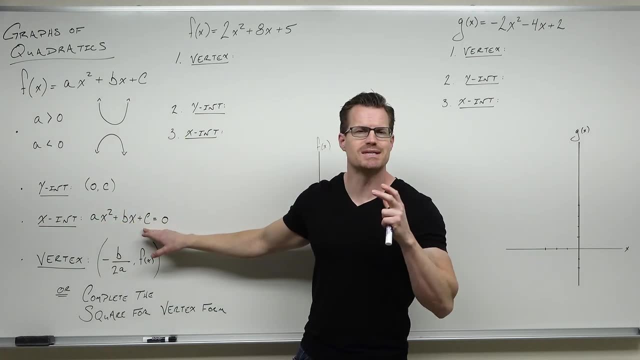 how we find the y-intercept by just plugging in zero to our x. evaluating the function for x equals zero. It's always going to be your c. We'll talk about that. We'll talk about how when you find x-intercepts. This is exactly why we've been practicing. the last few videos We set our 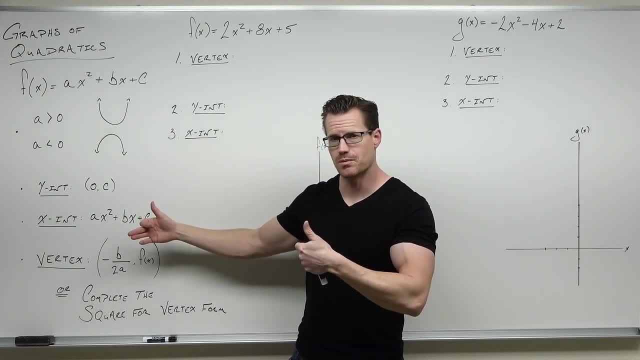 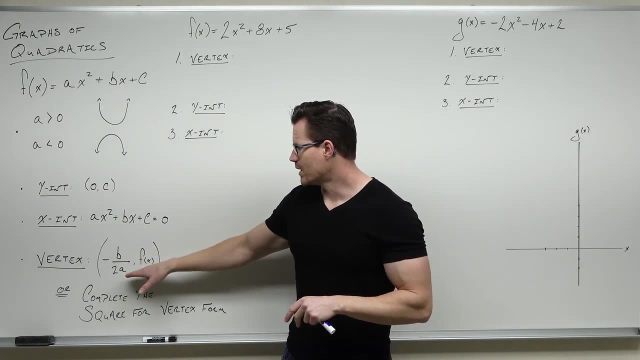 function equal to zero and we use factoring square method, completing the square or quadratic formula. Here it's pretty much all going to be quadratic formula if we need to. And then well, we find the vertex one of two ways: either by completing the square, which I'm going to show. 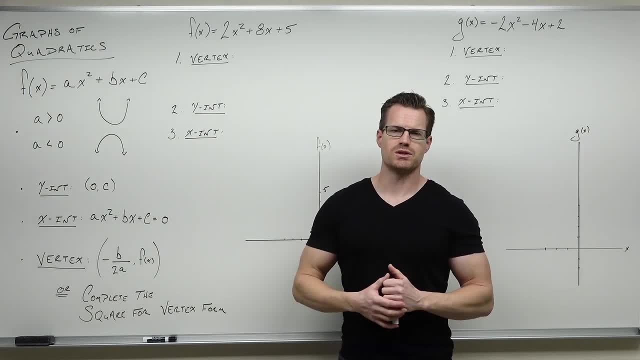 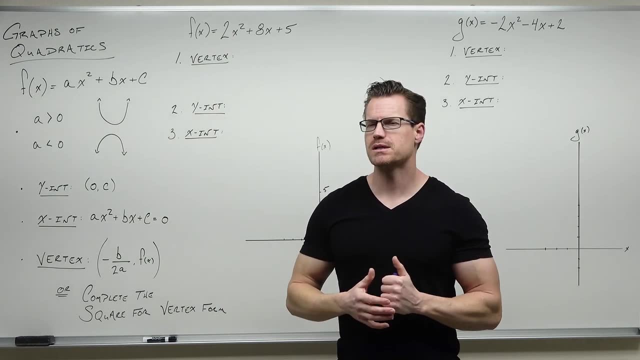 you, or by using this vertex formula, which is so much nicer to use. So this is pretty much what we're going to do. I'm going to show you the order in which we go through it and that's going to be just about it. We have maybe four examples. I'm going to show you going backwards, If I give you. 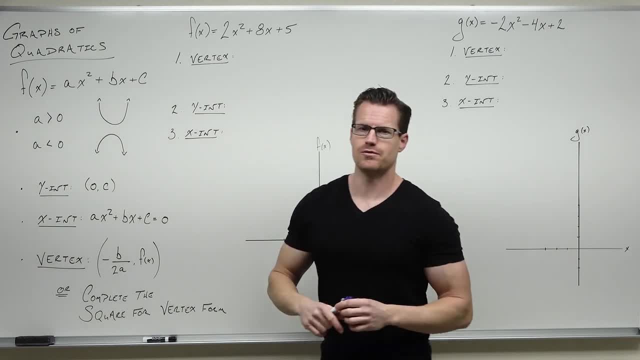 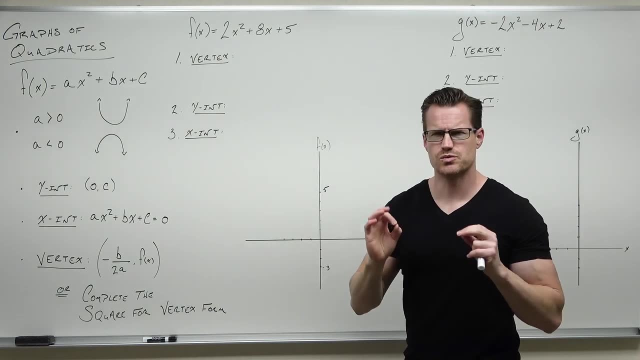 a vertex and a y-intercept how we make something in standard form. So let's take a look at our first function. It's clearly a quadratic. It's got that power. two: There's three terms. They're in order. It looks really nice. Here's the order in which we graph parabolas. Number one: you have. 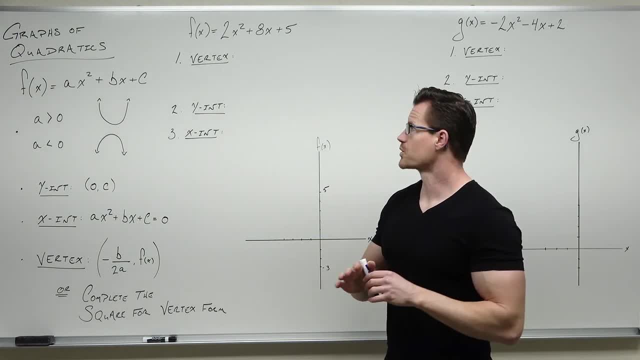 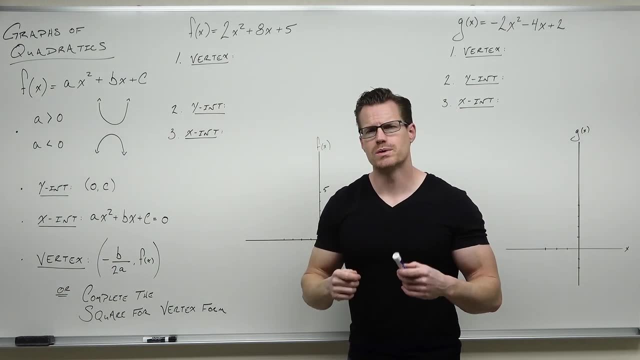 to make. Either you're going to do completing the square or you're going to find the vertex first, then the y-intercept, then the x-intercepts. In that order you graph them Again. the reason why? because I don't want to hold you in suspense. this order works because every parabola is going. 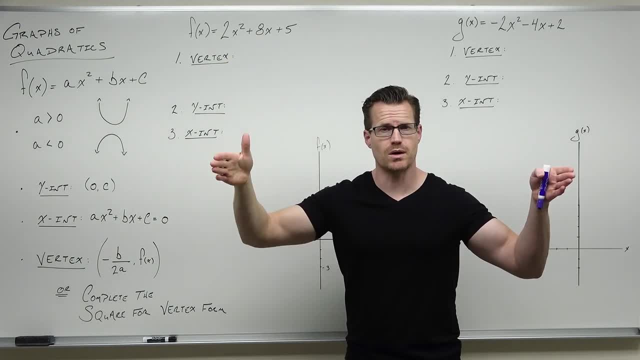 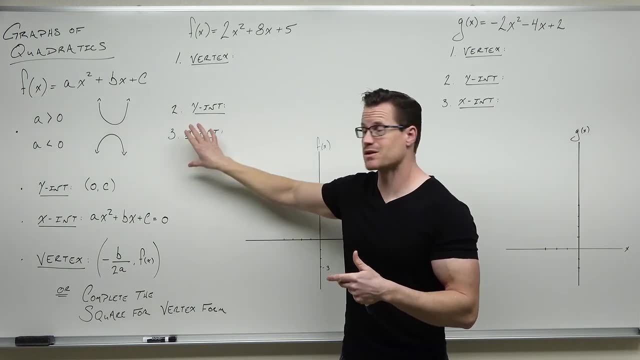 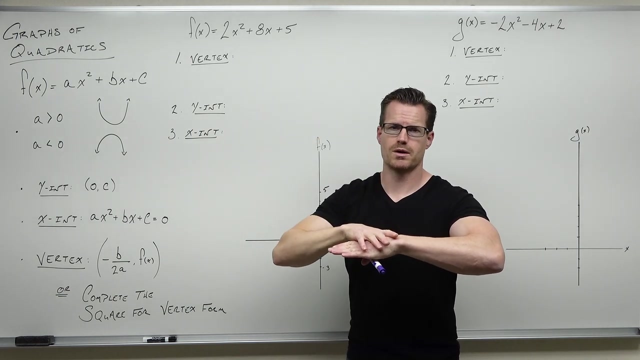 to have a vertex, and every parabola is going to eventually cross the y-axis, but not every parabola has to cross the x-axis, And so we do this in order to save ourselves some work. If we find a vertex above the x-axis and we know it's upward opening, we don't have to worry about the x-intercepts. 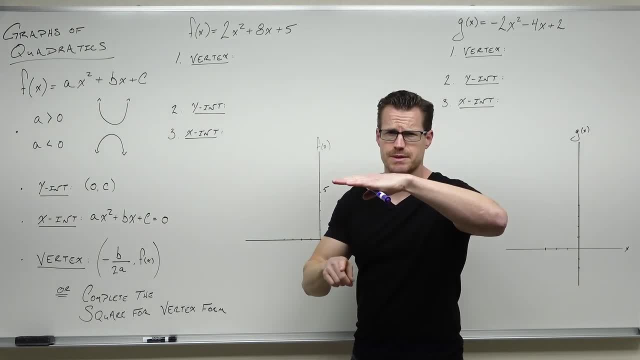 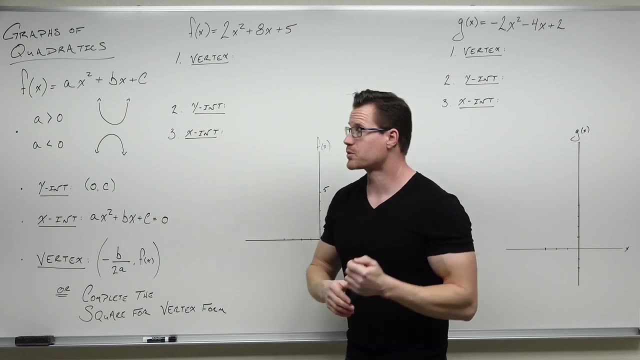 Or likewise, if we have one below, we don't have to worry about the x-intercepts, And so we go in that certain order to make certain we're not wasting our time finding x-intercepts that aren't even there. So let's go through it together. We know that's a parabola. We need to determine that. 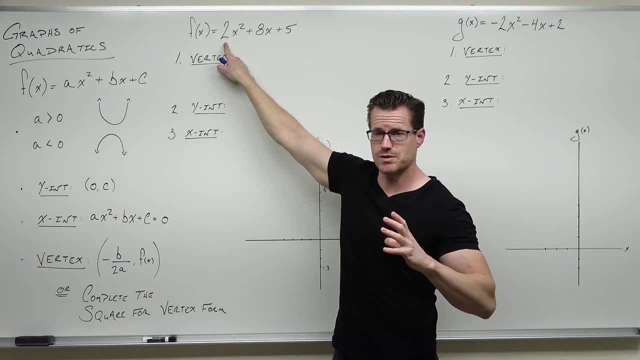 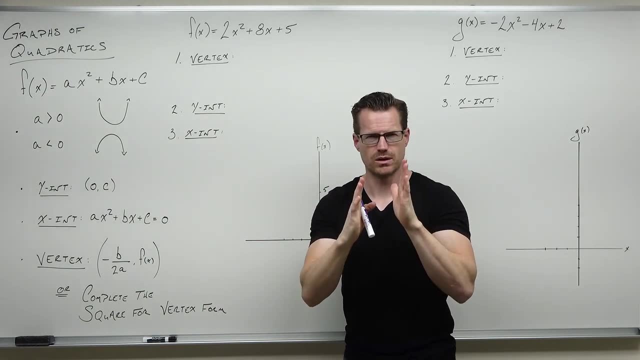 because that two is positive and because that two is an absolute value greater than one. this is going to be an upward opening parabola and it's going to be a little bit more vertically stretched, So a little narrower. What we're going to do first is find the vertex by this vertex formula. So 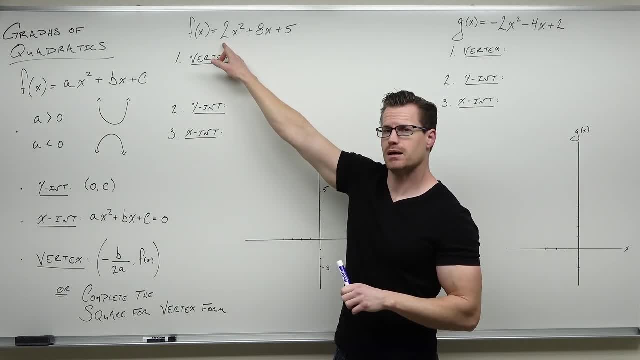 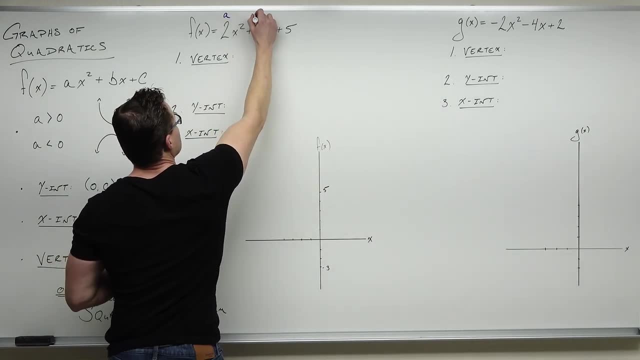 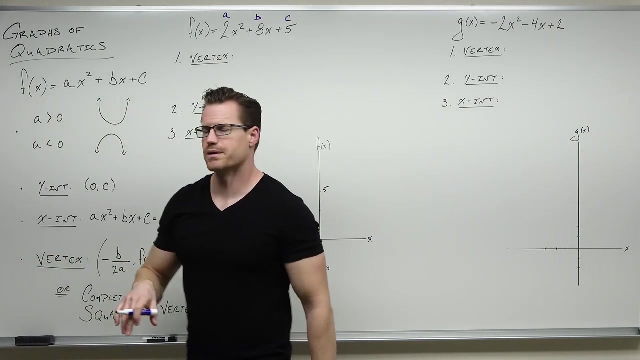 vertex formula says: if you can identify your a and your b and your c, which we should be really good at because of the quadratic formula, the vertex formula is going to give us that vertex. Now here's how to find it. It looks really familiar because from the quadratic formula. 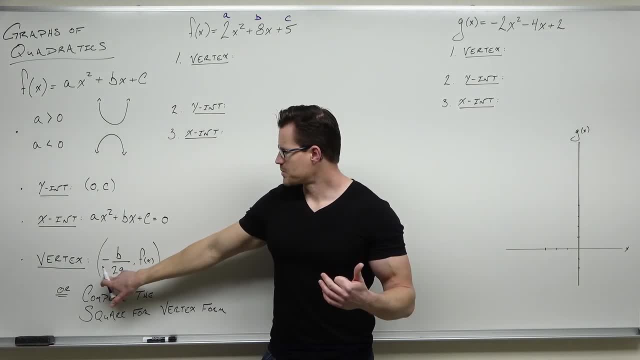 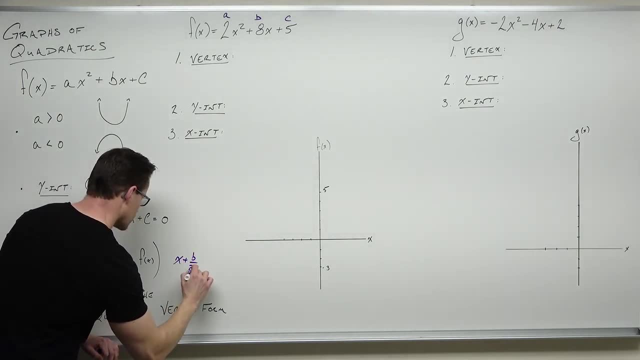 if you remember maybe, you maybe watched that proof video again, this part was the piece that we're going to look at later Before we take a square root. Now, why is that important? Because that's the only piece with an x in it, And this right here is in parentheses, And this means if 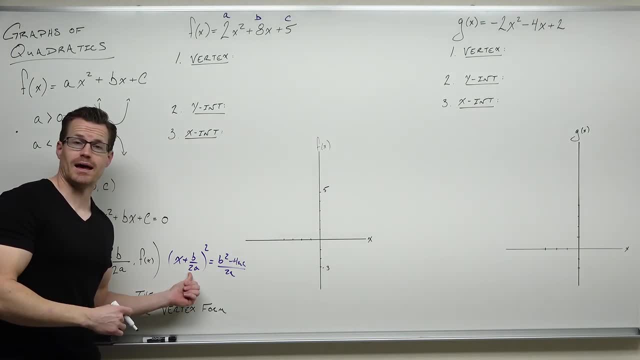 I looked at it like a function. this would be like a shift left. That's what that would be As far as our function is concerned, And this, if I move the other side, would be a shift up or down. That's what that's giving to you. So where the vertex formula comes from is this idea that 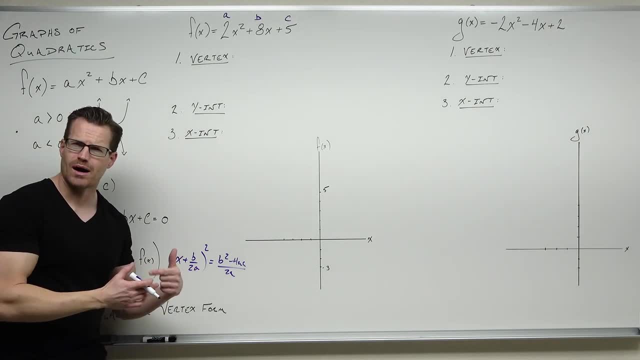 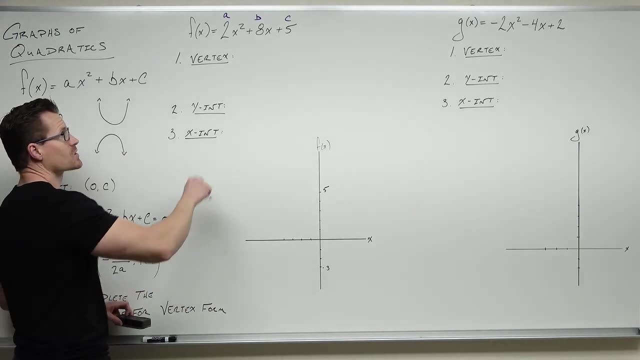 this is a shift left, hence the negative. And when we find out what that value is, that becomes the x coordinate of our vertex. How to find the y coordinate is: once you find this x coordinate- and we're about to do- we plug it into our function as what this stands for. So 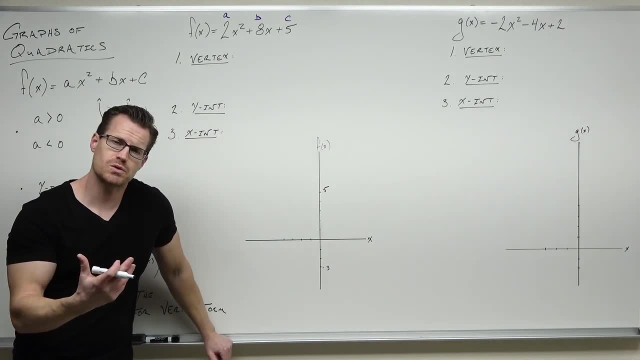 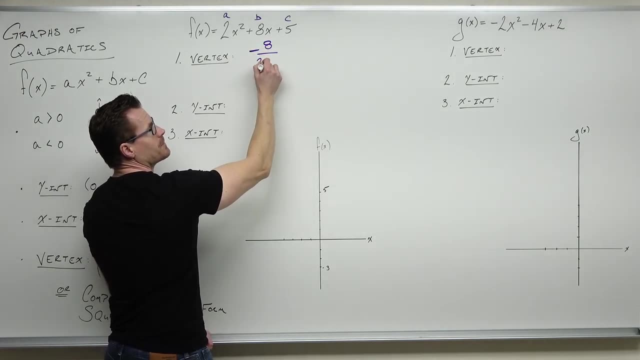 going to our vertex. it says: hey, identify your a, b and c. a is 2, and b is 8, and c is 5.. Our vertex formula says: take your negative b all over 2 times a, whatever your a is. In this case, our a is 2.. We're going to simplify that. 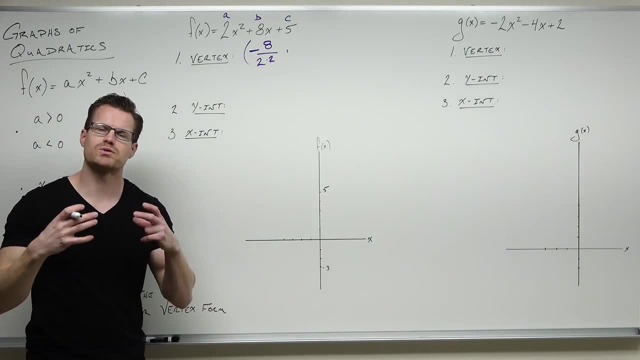 And then, whatever value we find, we're going to plug it into our function. That's how points work, including the vertex. Every parabola has a vertex. We use the formula to find the x coordinate And then, just like every ordered pair ever, we plug in the x or evaluate that x We get. 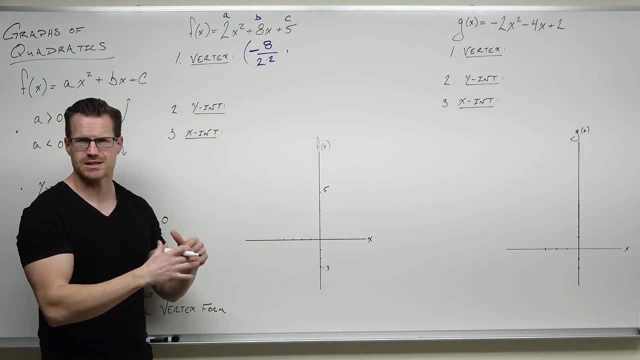 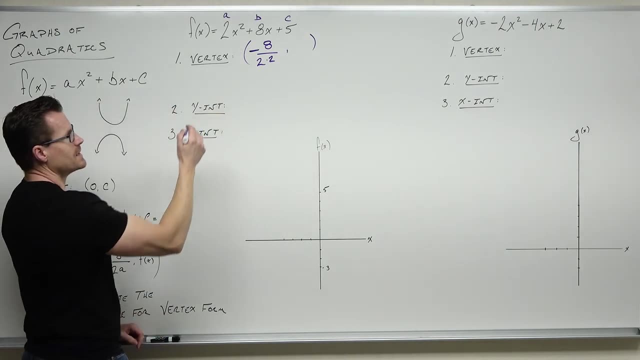 out the output. So we get out the y value, the y coordinate, the f of x, The same thing as calling a y. So this we're going to leave blank for just a second Negative 8 over 4 is negative 2.. 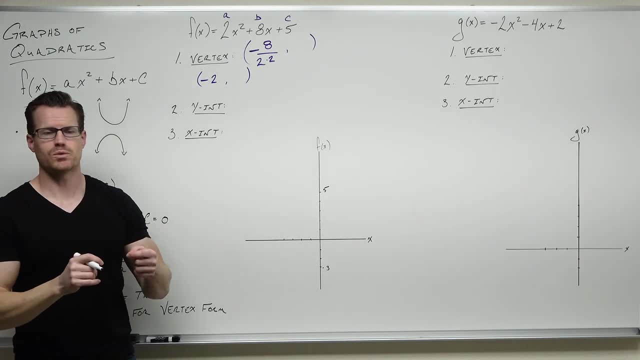 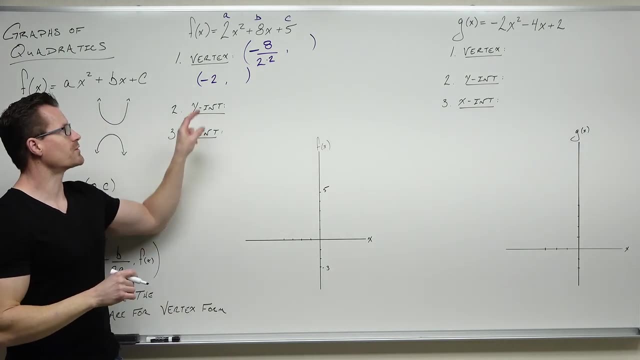 And then we evaluate negative 2 in our function. So we know right now that our vertex is going to be negative 2 comma, something along that negative 2 x value some output. We have to plug in that negative 2 in order to find the output. So negative 2 squared is 4. 4 times. 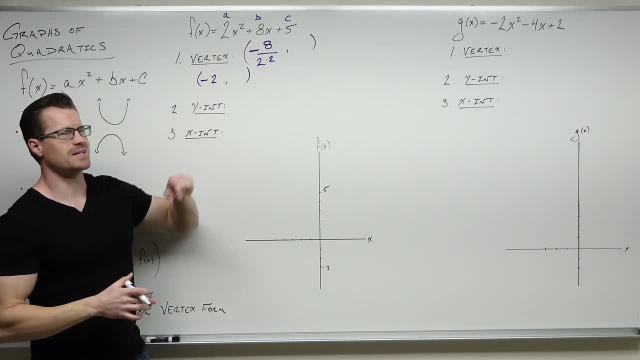 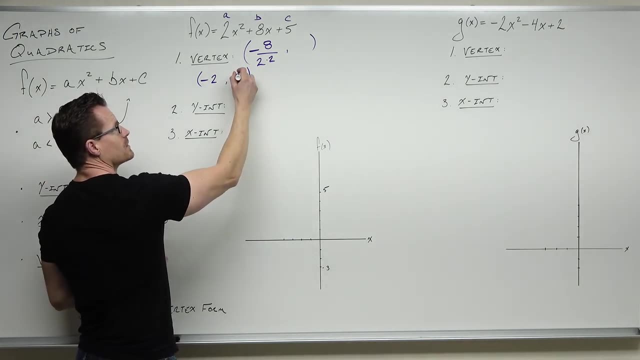 2,. well, that gives us 8.. 8 plus, let's see, 8 times negative, 2 is negative 16. That would be negative 8. And plus 5 would be negative 3. So we evaluate this as negative 2. And then we get out. 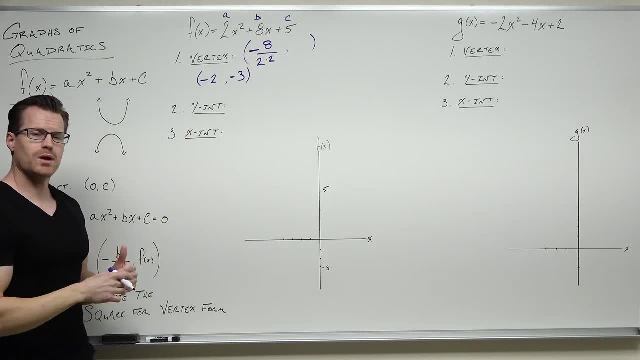 negative 3.. That is where our vertex is. Now we're going to plot that. We're going to plot that as we go. So negative 2 comma, negative 3 is this ordered pair: Negative 2,. negative 3,. 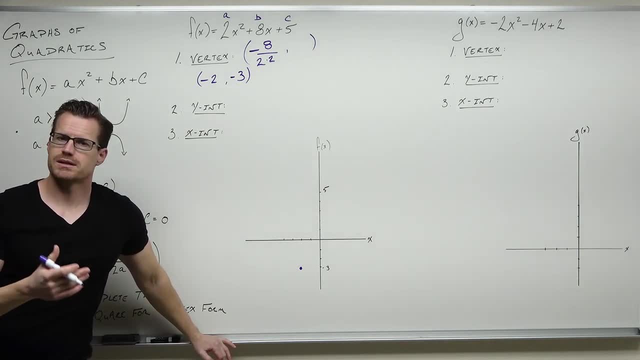 right about there. That's our vertex. Now think about this. This is an upward opening parabola. So if you are asked to find the minimum of this problem, which you're going to be asked to do on some of the word problems- you're going to get what's the minimum of this function. 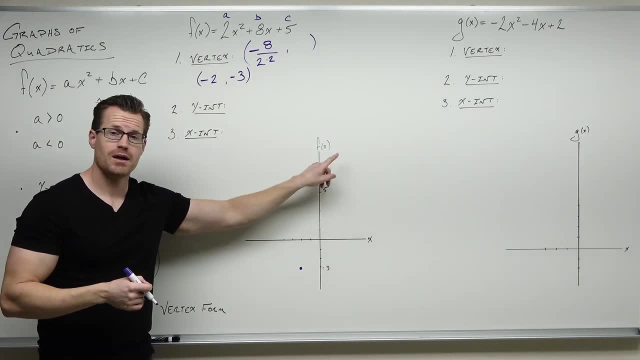 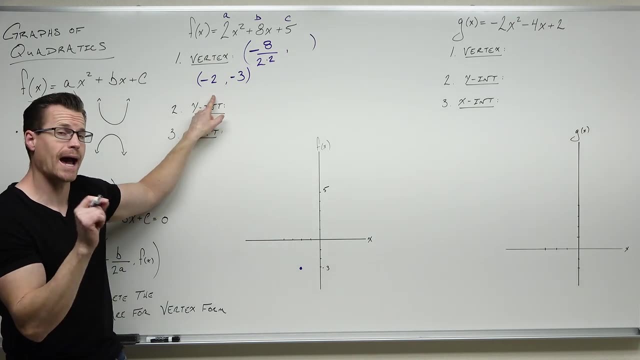 If this is an upward opening parabola and this is a vertex, then your minimum right now you're done. Your minimum value of this function is negative 3.. It's not negative 2. That's the x value where it happens. The negative 3 is the minimum height that this function attains. 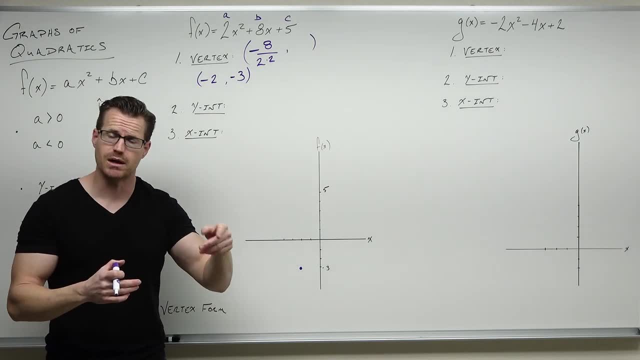 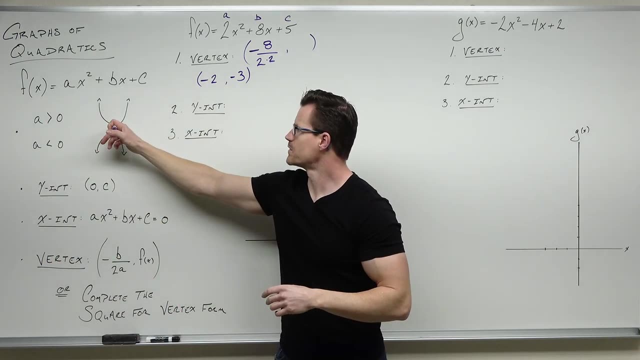 the idea of having a vertex being the maximum for a downward opening or minimum for an upper opening. So again, we've known, we said, hey, this is a parabola, We know it's going to be upward opening, Your vertex is going to be the minimum value on that function. on the graph of 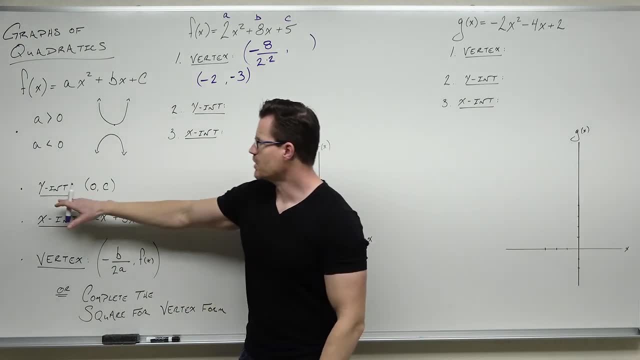 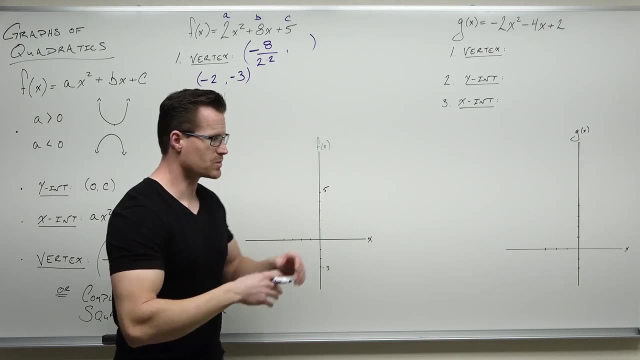 that function. the height that it sustains Minimum value is negative three. We know we can find a y-intercept, an x-intercept and a vertex by using some of these techniques we've learned already. Y-intercept is really easy. X-intercept we're using one of those techniques we learned about. 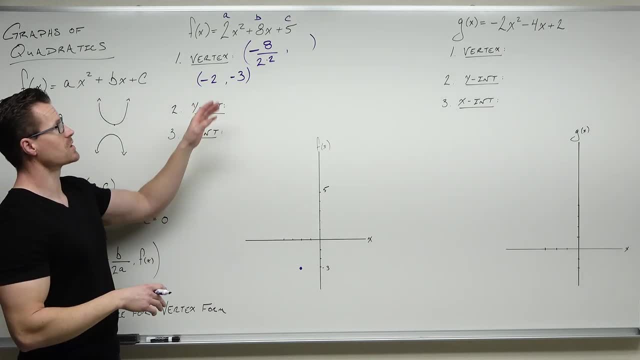 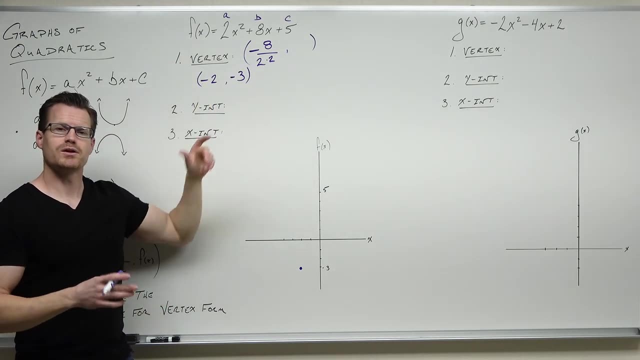 solving quadratics and the vertex has a formula. we just used Negative b divided by two a. We figure that out. We plug it into our function. We get an ordered pair that represents your vertex. Your y-intercept should be really quick. The y-intercept occurs where you plug in zero to your 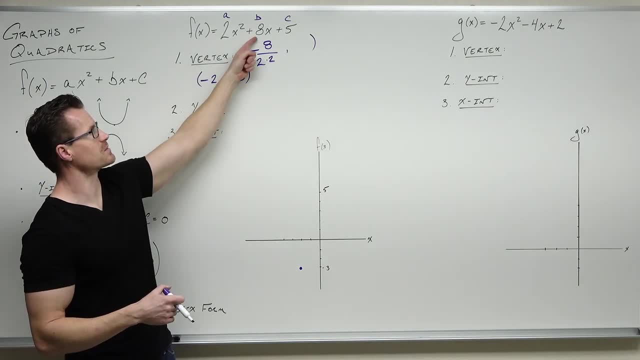 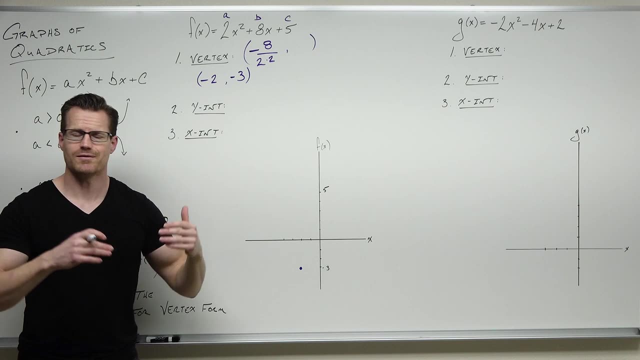 x. So if we plug in zero, hey, that's going to be zero and that's going to be zero. Can you see that if you evaluate your function for zero, you are only going to be left with the c value? If? 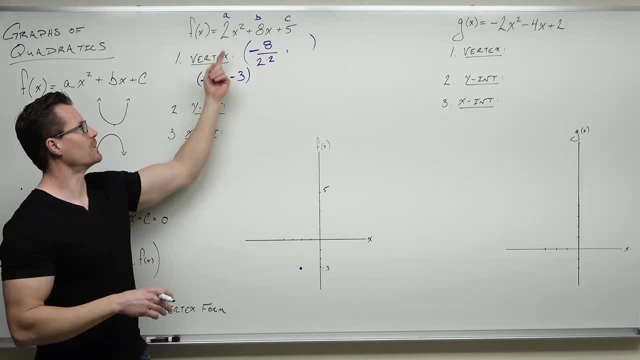 your function is a standard form. it means it looks like this: Then, if you plug in zero, these things are going to be zero. If you plug in zero, these things are going to be zero. If you plug in zero, these things are gone. You're just going to get your c value and that's. 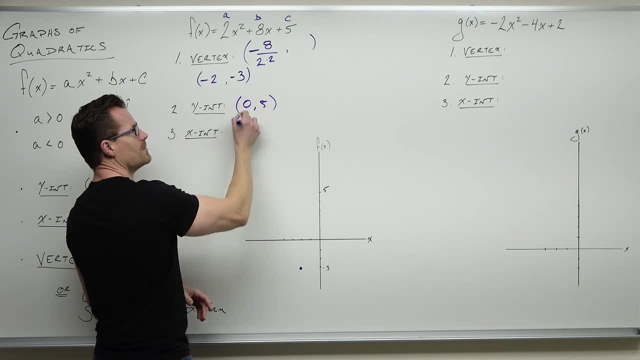 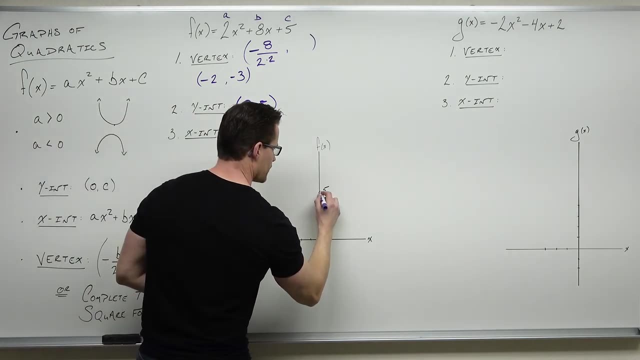 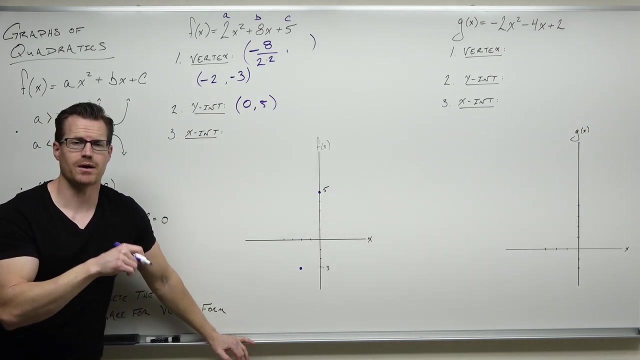 what happens. It should take about five seconds to find this at most. So we know that our y-intercept is zero comma five. We're going to plot that next, And now we're going to determine something. You see, I gave you an order of steps so that we could identify whether or not we need to find. 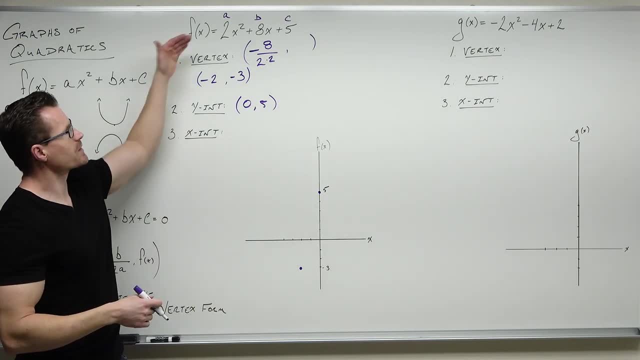 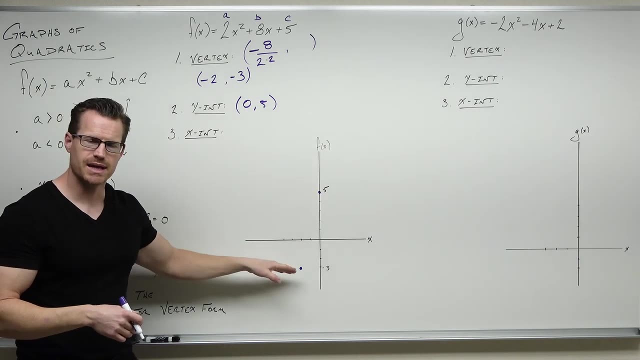 x-intercepts or not. So right here, because we know it's upward opening, because we have a x-intercept, we're going to have to cross this x-axis in this parabola. So here's our vertex. We know it's upward opening, Yeah, we're going to have to cross this somewhere, probably somewhere. 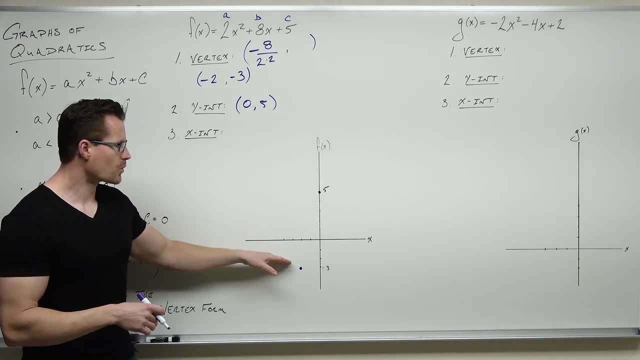 between here and here, of course, because it's got to be symmetrical, We're going to have to cross that. That, right there, tells you whether you need to continue to find x-intercepts or not. Had our vertex been above the x-axis and we were still upward opening. we don't have to do this. 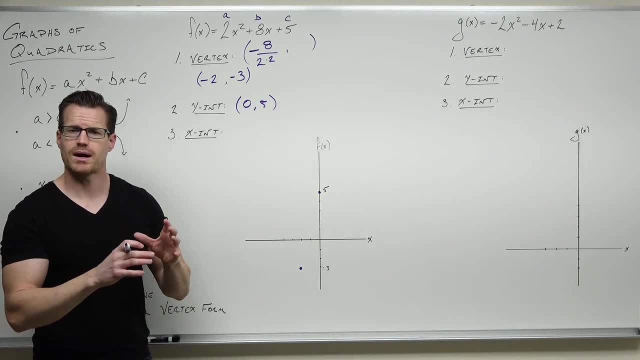 next step. So to make it very clear, when you're graphing parabolas, we always find the vertex, no matter what. We always find the y-intercept, no matter what. We always use the y-intercept for a free point. I'm going to show you in just a second. But then sometimes, 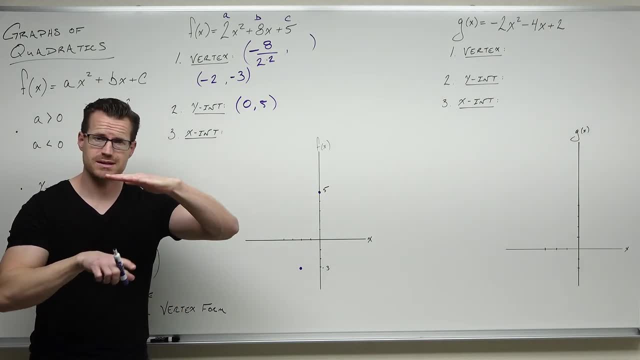 we find x-intercepts if we have to. Vertex below the x and upward opening: yes. Vertex above the x and downward opening: yes, But not if we're above and upward or below and downward. I hope that makes sense to you. So here we're going to find in just a minute, But before we do that I need you. 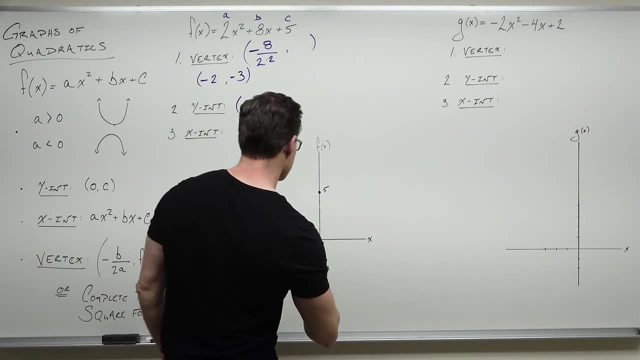 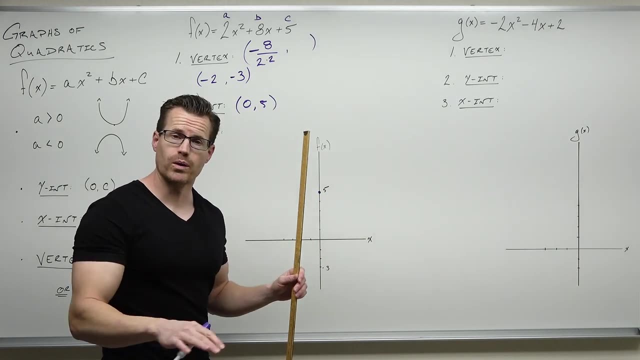 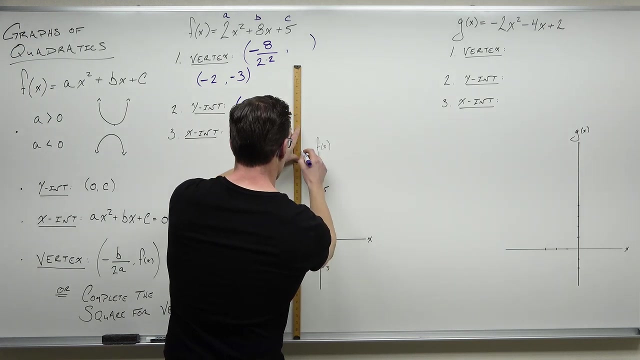 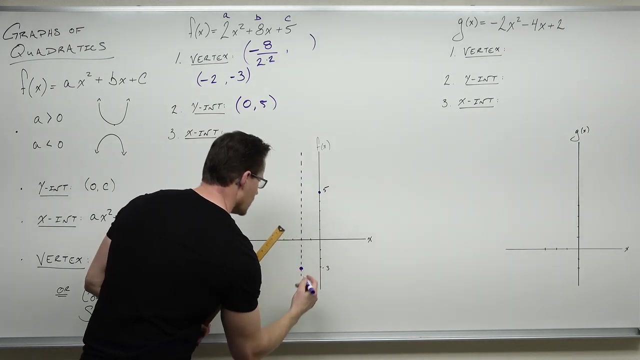 to make sure that our parabola is symmetrical, And because it's symmetrical, we have this thing called an axis of symmetry And it's always going to go through your vertex. So our graph is going to be this mirror image across that dotted line. 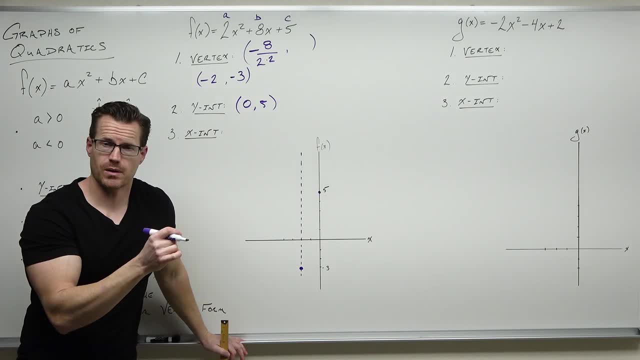 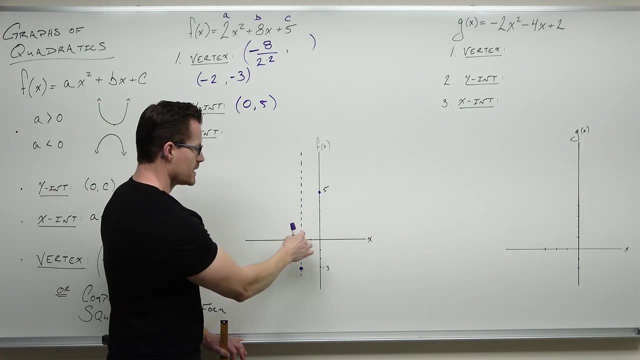 What that means is this: If you have any point on one side of that axis of symmetry, you can mirror that image on the other side being equal, this in front of it. So because this 5 is, let's say, 2 units away from 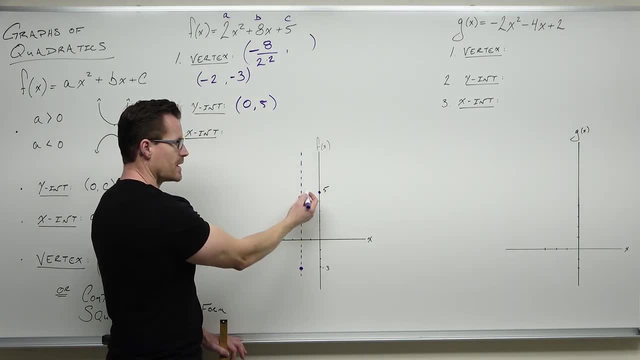 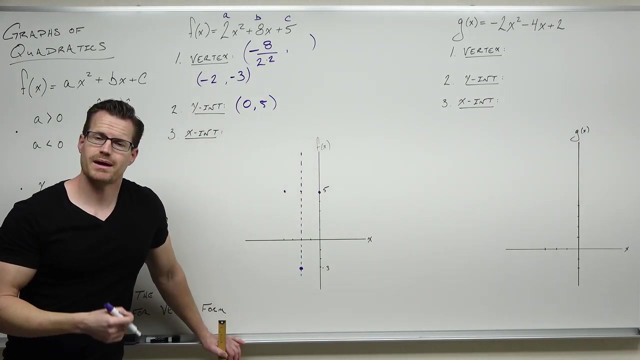 the axis of symmetry. this is negative 2 comma 5, is where that would. this point right here is Because this y-intercept is 2 units away. we can go 2 units away on the other side at negative 4, 5.. 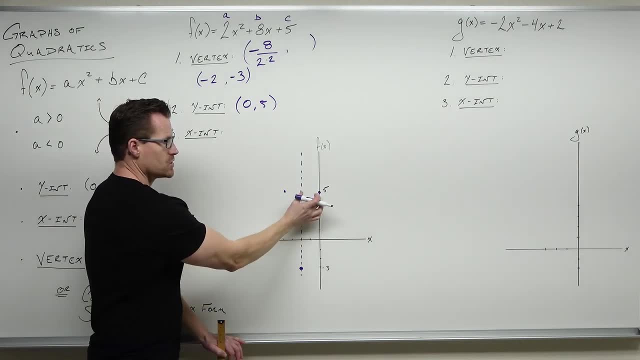 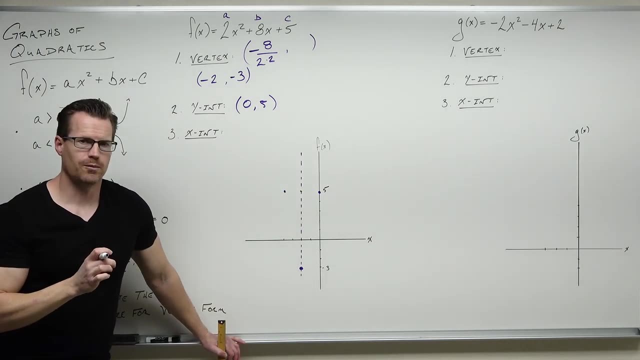 And put a point. So we know that that's symmetrical. Here's two units away from the axis of symmetry. The other side of that axis of symmetry is going to create for us another point. This is very, very helpful in your graphing. 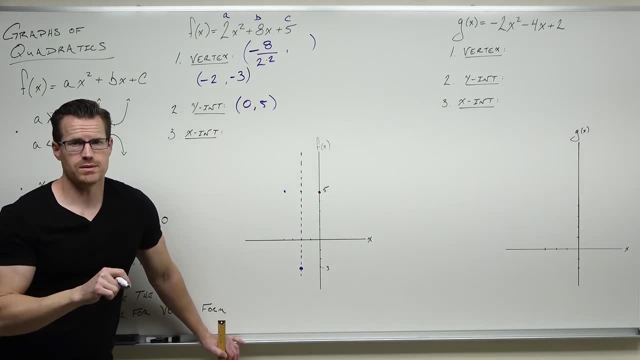 You get a point for free. That's really nice. We can always do that with our y-intercept, provided the axis of symmetry is not on the y-axis. So we're always going to. we're always going to graph a vertex, No problem. 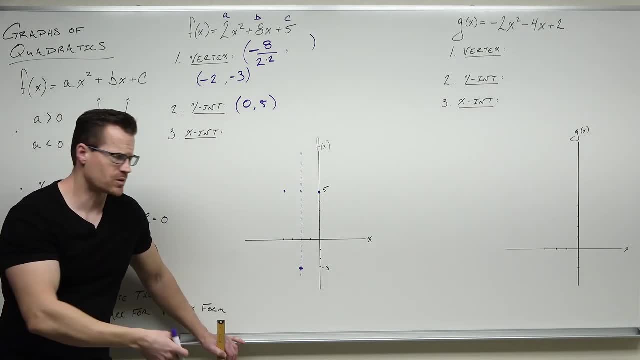 We're going to graph the y-intercept Great. We're going to use the axis of symmetry that always goes through your vertex to give ourselves a mirror image from the. We're going to use the axis of symmetry that always goes through your vertex to give ourselves a mirror image from where we're at. 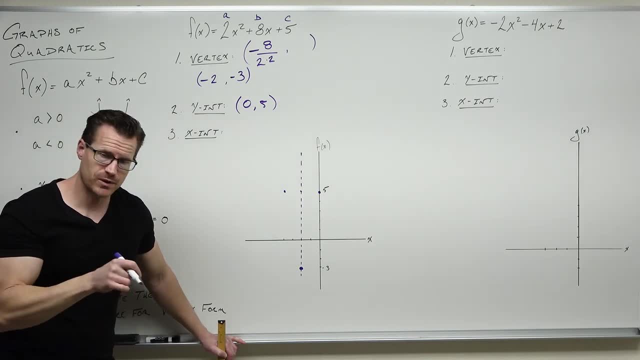 group, you're expect to be in the right match where that y-intercept is, And then, if we need to, we're going to find x-intercepts. So how we find x-intercept is always setting your function equal to zero. 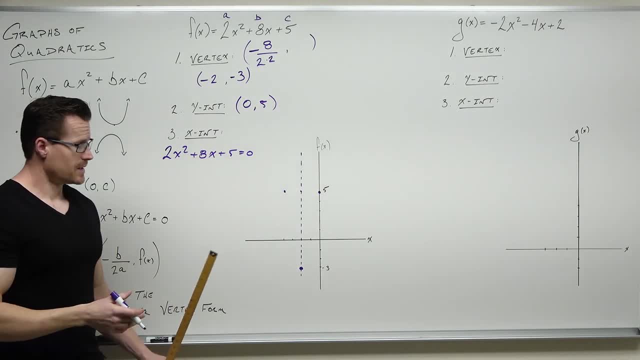 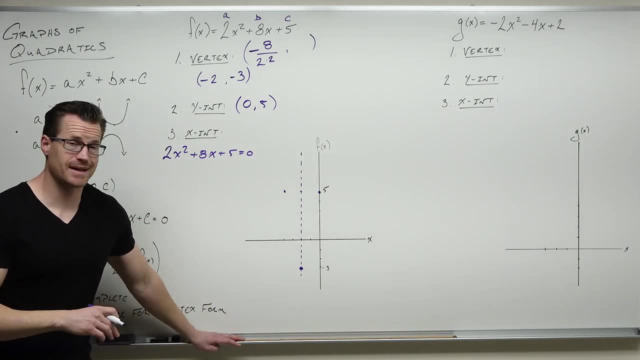 And then trying to factor or trying the square root method, trying something Hearing the square root method is not going to work. We can't get a power 2 by itself that contains all of our x's and have a constant on the other side. That's not happening. 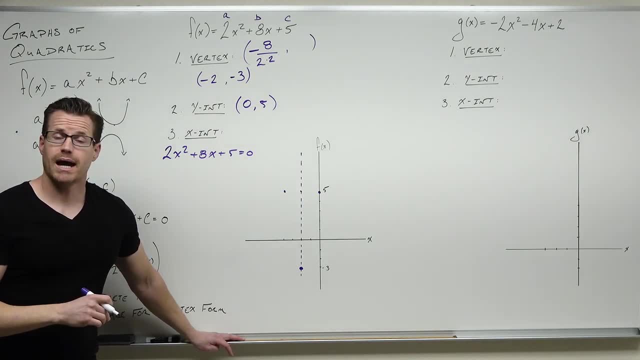 And could we do the completing the square? Yeah, we can, And I'm going to do that in a minute to show you that we can solve it that way. People generally think it's a little bit more work and unnecessary, but I want to practice it to show you that it does work, If you're asked to. 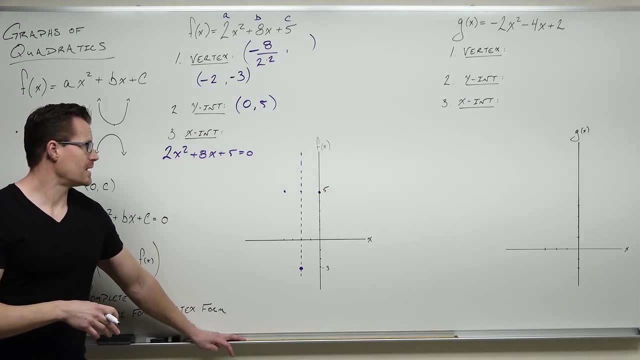 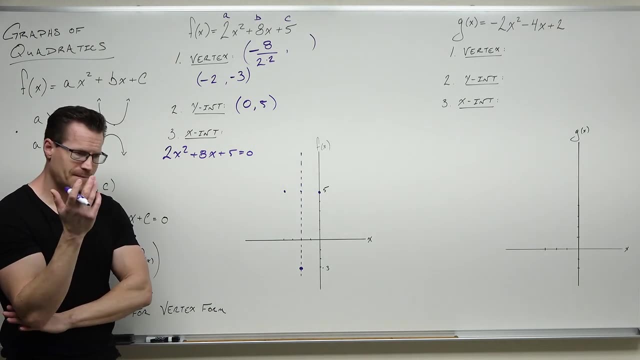 do vertex form. that's what you have to do Instead, if we can't factor, let's see 8, add to 8, multiply to 10, that's not going to happen. So, man, the only thing we've got. 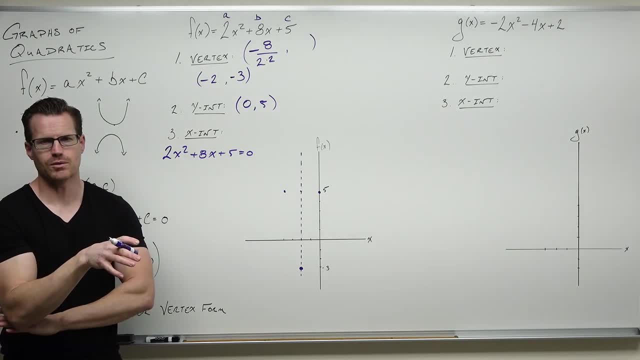 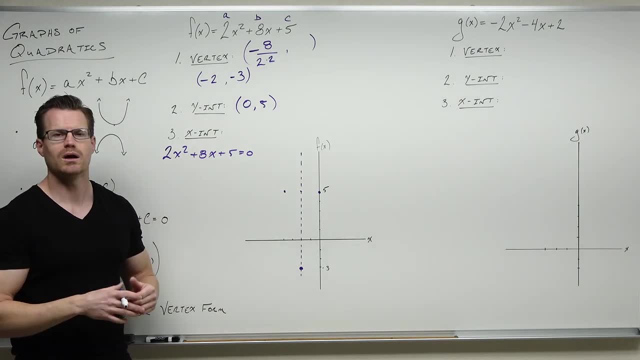 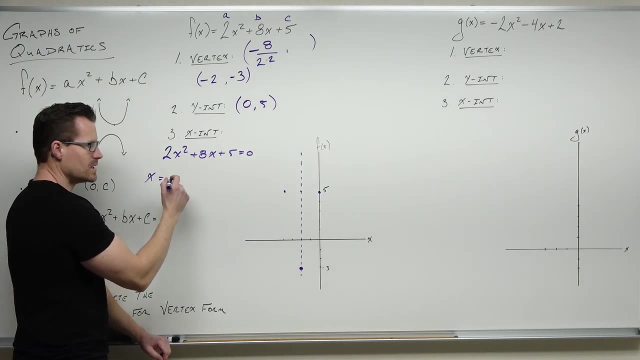 set this function equal to 0 and nothing else works and we don't want to complete the square. do the quadratic formula So identify your a and your b and your c, which you've already done, And we understand that our x would be equal to negative b plus or minus. 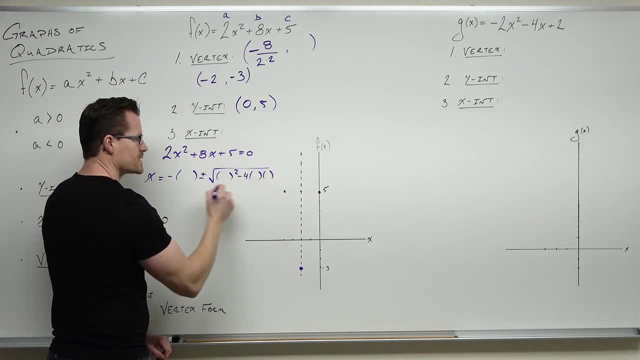 this whole b squared minus 4 times a, times c- And we've done this before, all over 2 times a- And say, hey, our 8 is b, our a is 2, and our c is 5. And we end up getting this. I'm going pretty quickly here, but we want to make sure. 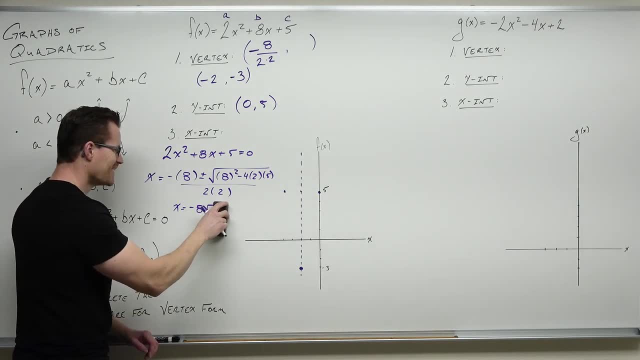 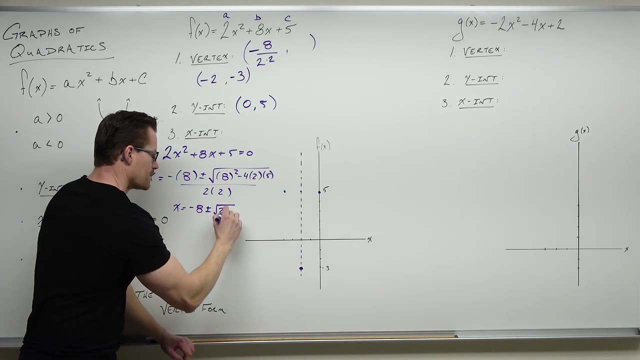 that we're not making any mistakes. Ironic, because I forgot something. And it's 64 minus 40, that's 24, all over 4.. So negative 8, we've got a 64.. We have minus 40,. 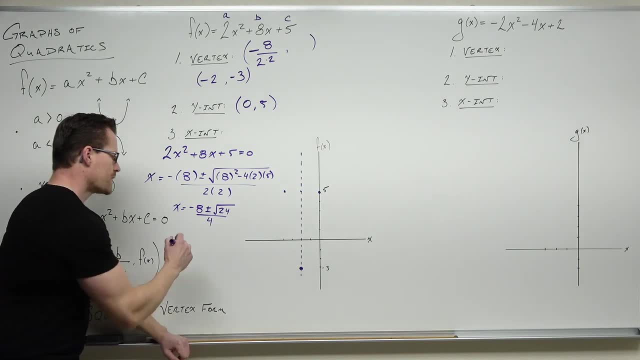 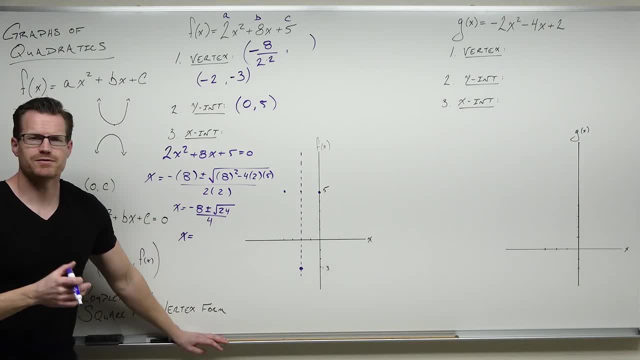 solution. I mean, we know we have x intercepts. There's no, i's here. We know we're crossing the x, but it's very hard to graph And so we're going to approximate it And we're going to say, all right. 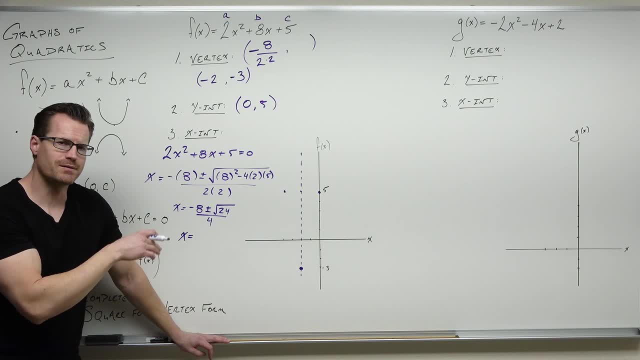 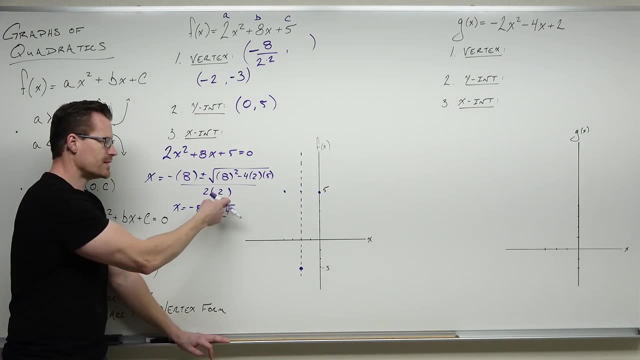 once we take this: negative 8 plus the square root of 24 over 4, negative 8 minus the square root of 24 over 4.. Notice what I'm not doing. I'm not spending a whole lot of time simplifying this. 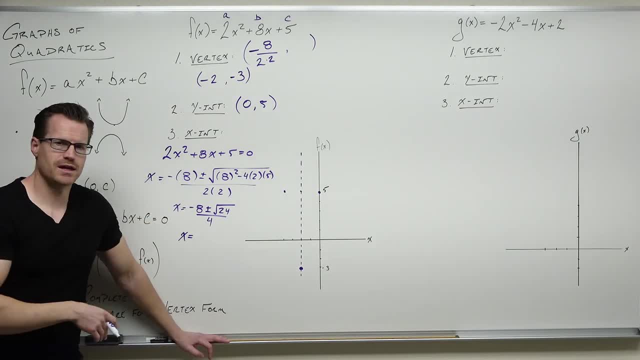 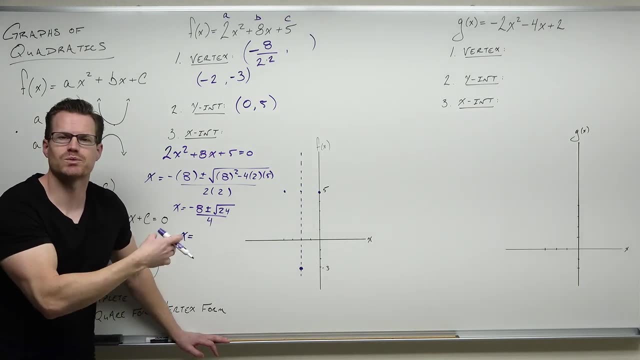 by factoring out that square root of 4 and simplifying with 8 to 4.. I don't care, Because all I'm trying to do here is approximate my x-intercepts. I'm trying to get a number that I can actually graph, And so that's what we're going to do here. So I'm going to do this. I'm 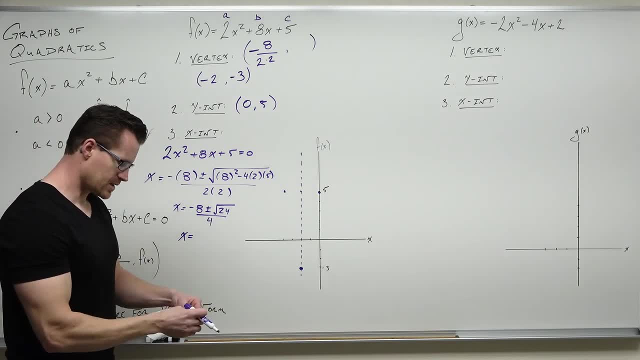 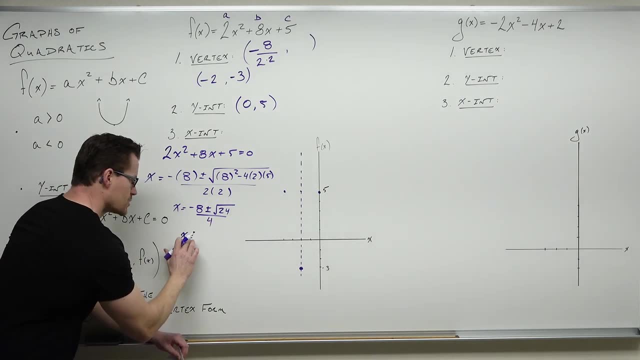 going to do this, And so that's what we're going to do. So, after taking a break and work on this under calculator or whatever I got that our x-intercepts are about, So I'm going to change this to: about equal to negative 3.22 and negative 0.77.. Let's see if that kind of copes with what. 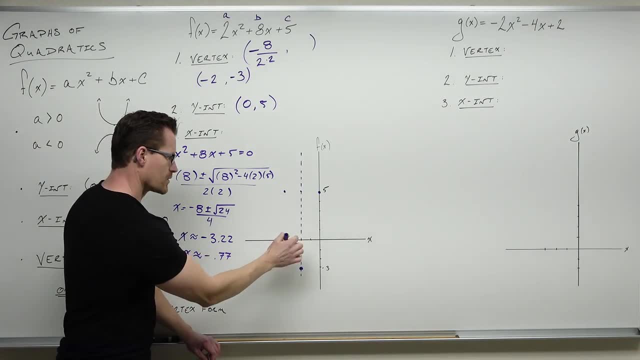 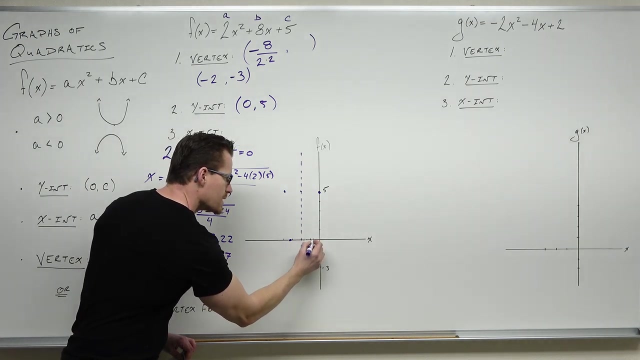 we got here: Negative 3.22.. Negative 1, negative 2, negative 3.22.. And then negative 0.77.. Negative 0.77.. Here's what we want to check, Because we have this nature of symmetry for. 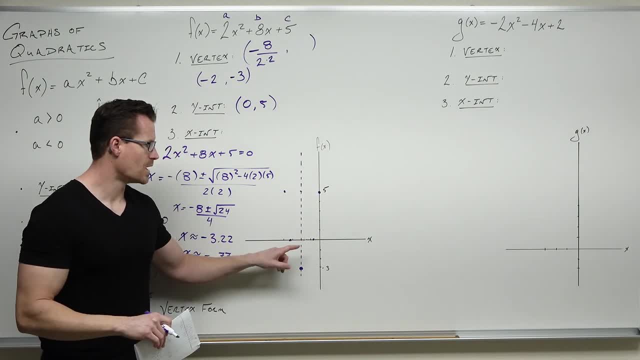 every parabola. in fact, we use it to get a free point for a y-intercept. we want to make sure that our x-values, our x-intercepts, are also symmetrical on this graph, So they're the same distance from the axis of symmetry on both sides, And this is the only reason why this is a little. 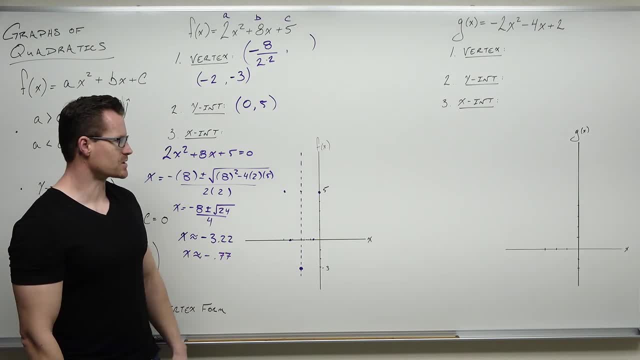 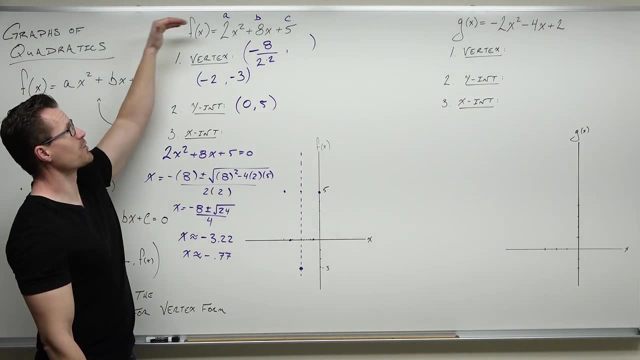 bit off is because this is the same distance from the axis of symmetry on both sides, And this is because of a rounding error. That's, that's the idea. So, man, once we have that, those five points are what we need to make a really solid graph for a parabola. We have determined that. 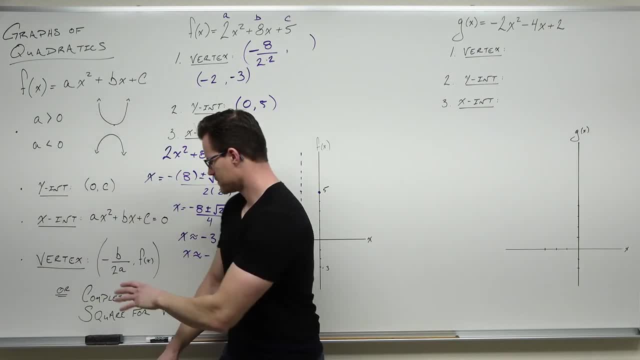 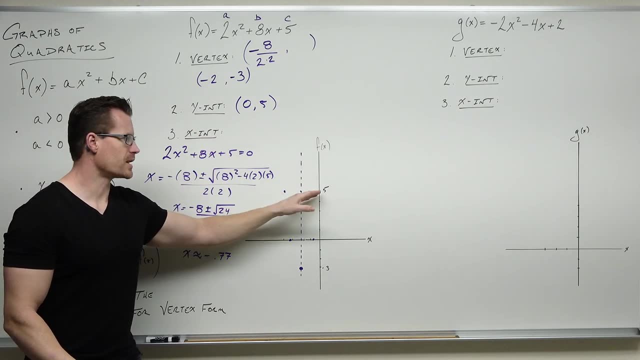 every parabola has a vertex. Find it first. Use the formula. Use the formula I've given you. Find the x-value, plug it in for the y-value, Plot it. Then find your y-intercept: Plot it. Use the. 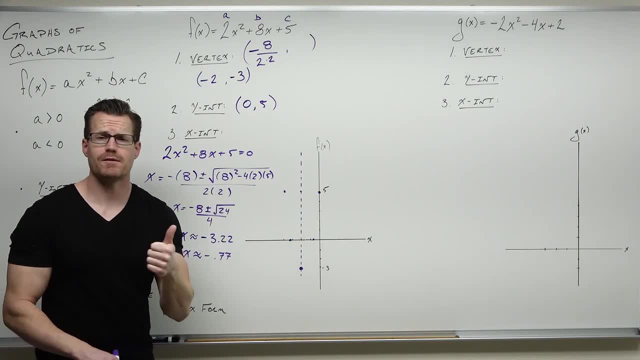 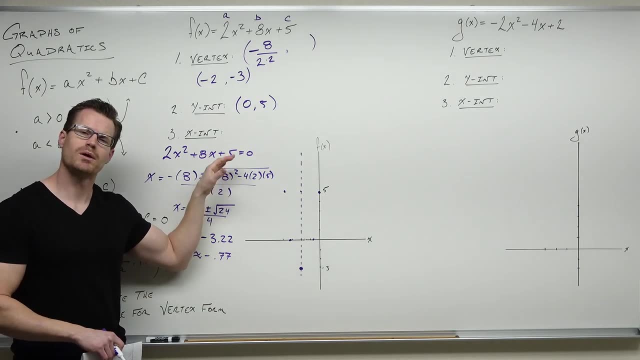 axis of symmetry. to give you a free point, Plot it, Determine if you need x-intercepts. If you're going to be crossing the x-axis, you've got to find them. Sometimes that means when we set the sequence equal to zero- and it's not factable- we're using the quadratic formula, plugging this. 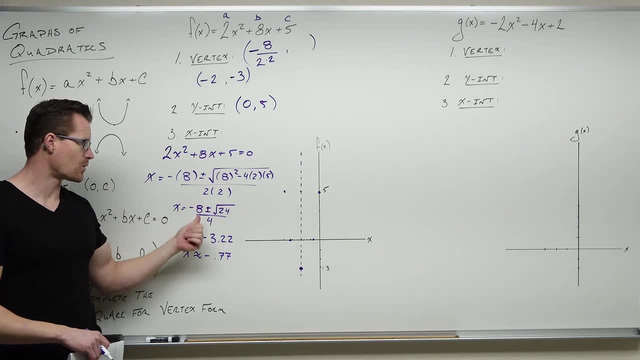 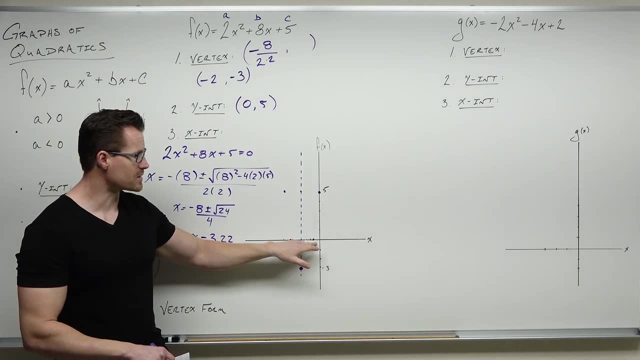 into our calculator: negative 8 plus square root of 24, and then divide by 4, negative 8 minus square root of 24, then divide by 4, getting two values, plotting them on our x-axis and double checking. they're the same distance from the axis of symmetry. After that we have something that 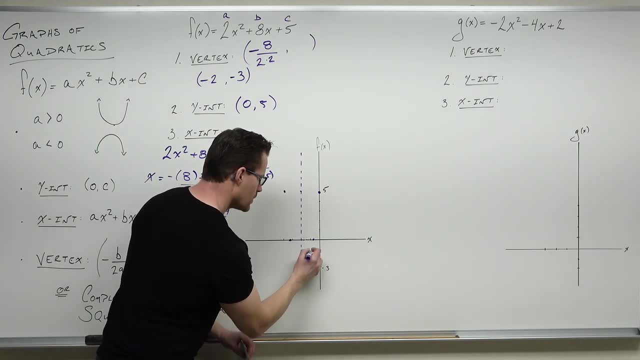 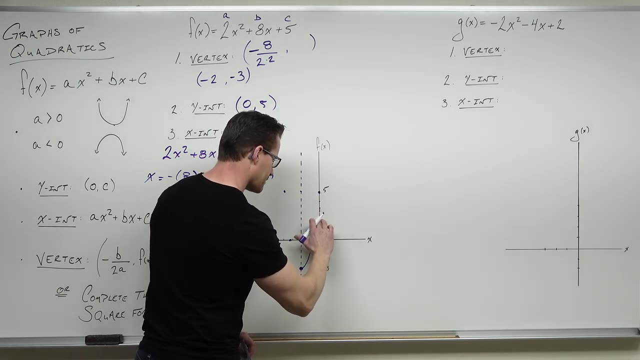 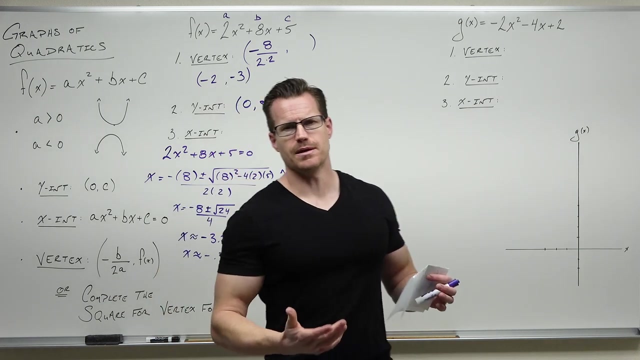 we can graph with a nice smooth, flowing curve. We can make it as symmetric as possible And that's about as good as I can do by hand, to be honest with you. I hope that makes sense. the idea that parabolas are these shapes we get for quadratics They're all going to make. 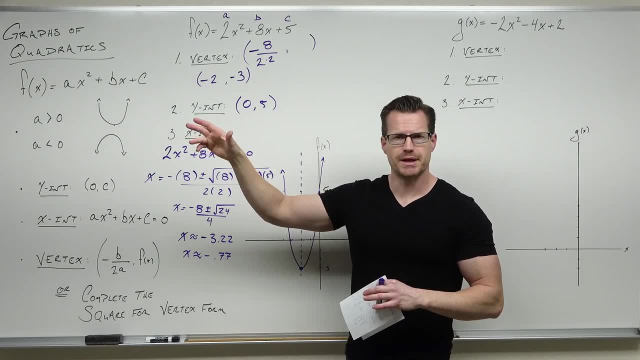 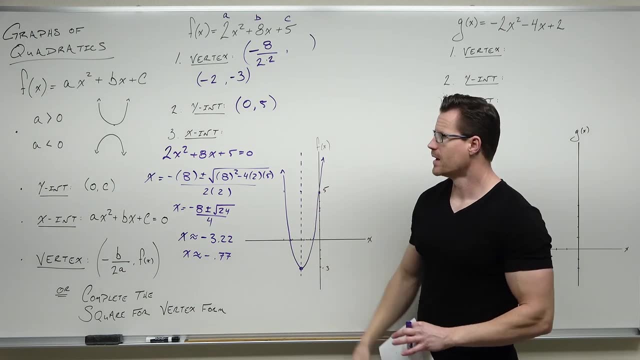 that. I hope it makes sense that if your a is positive, we're upward opening and negative, we're downward opening And then we have a vertical stretch of compression. This one is stretched a little bit, You can see. it's a little more narrow than normal. I hope you understand. 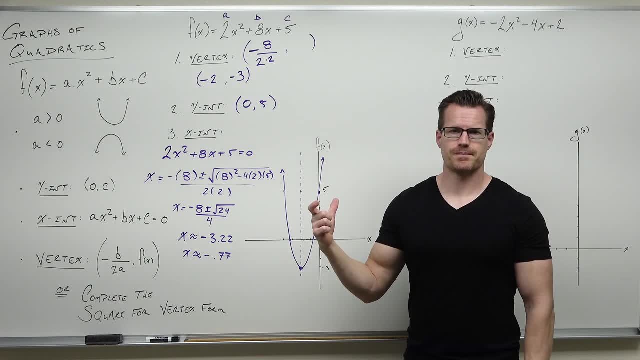 that every parabola has a vertical stretch of compression. and if we have a vertical stretch of compression, every parabola has a vertex. We're going to find it first. If it's below the x-axis and upward opening you're also going to have x-intercepts. so we've got to keep that in mind. 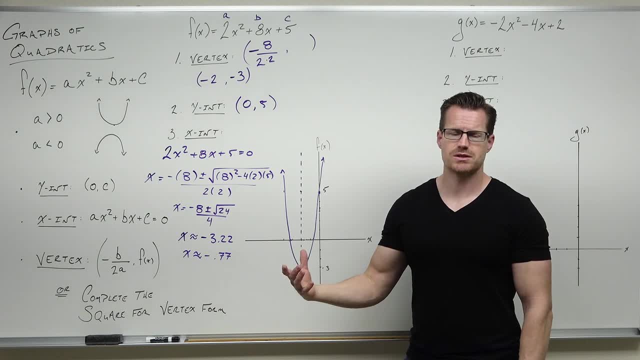 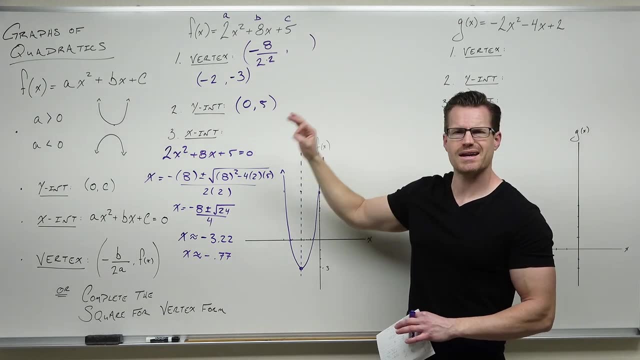 If it's above the x and downward opening, again you're going to have x-intercepts. so we've got to keep that in mind. Every parabola has a y-intercept. They're easy to find. We just plug in zero. we get our zero comma c. X-intercepts might take some work here. 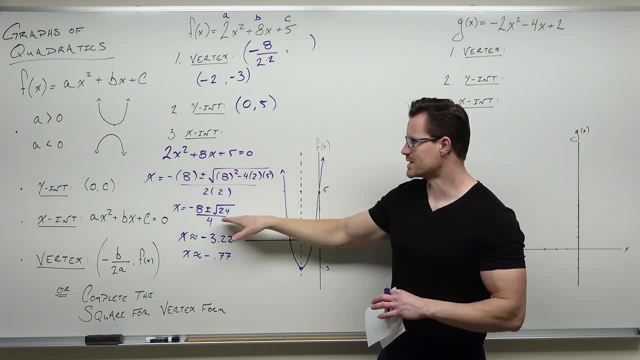 because they're not always factorable. Quadratic form is going to give us an exact representation for x-intercepts, but to graph them we might have to approximate it. So we're going to have a vertical stretch of compression and then we're going to have a 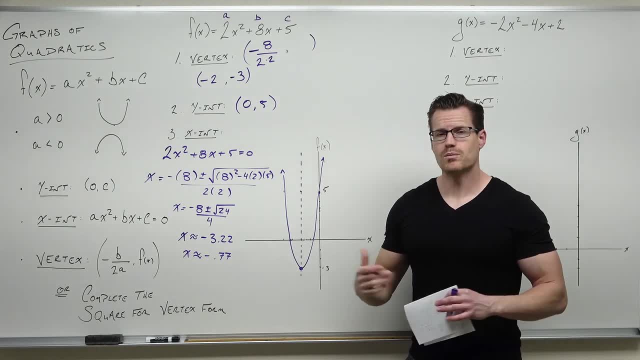 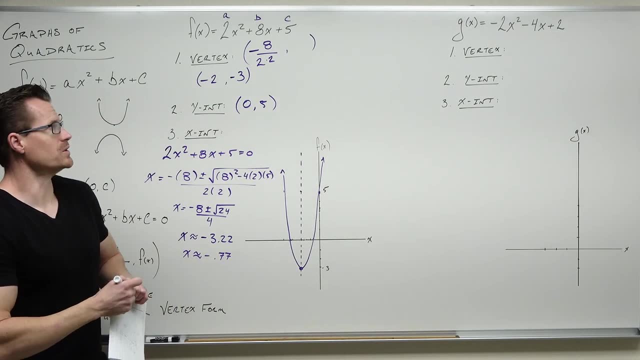 x-intercept. That's got to be there before we go any further. Now one more thing that we can do If you're asked to put this in vertex form, or if you just want to double-check to make sure that you got this right. I mean, I wouldn't I would trust this, But if you have to, 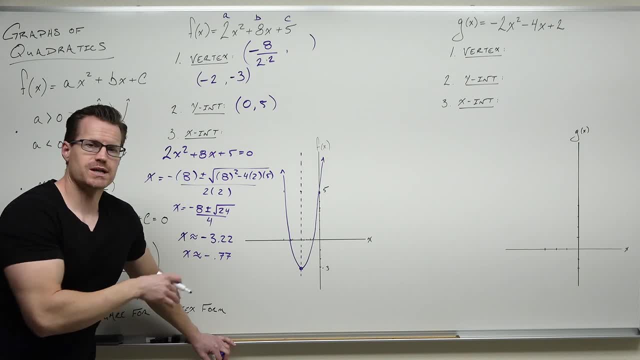 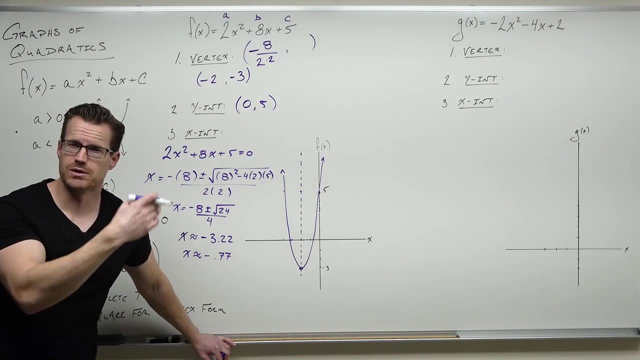 we can always complete the square to verify our vertex. This is called vertex form because of the nature of completing the square, putting this in the form of being able to use transformations, the shifting up down, left right. This is also the reason why I taught completing. 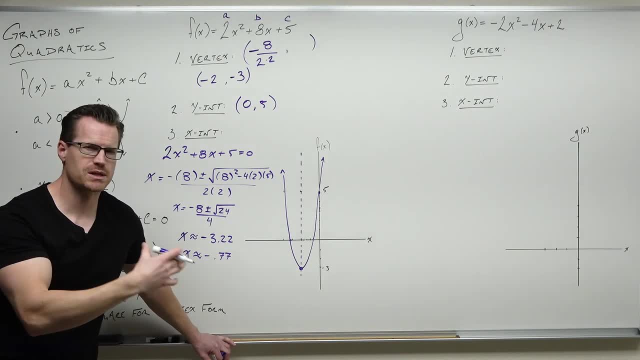 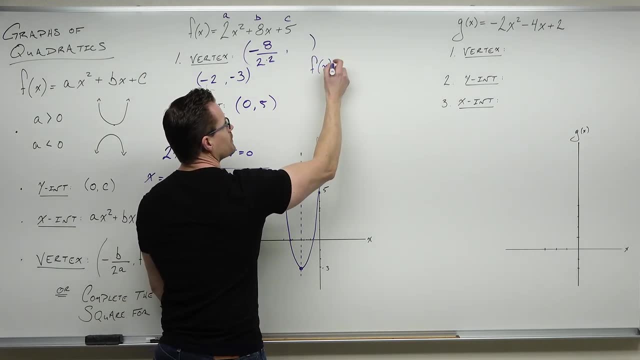 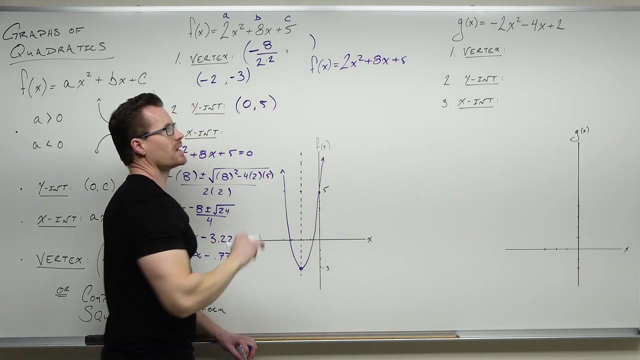 the square the way that I did, the way that we didn't work on both sides of our equation. So I want you to understand that when you complete the square on a function like this, what you're doing is putting this in what's called vertex form. 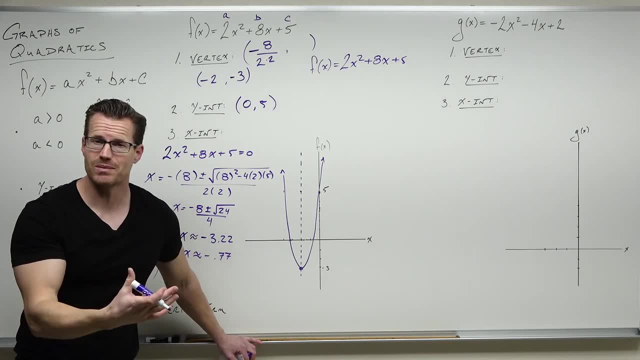 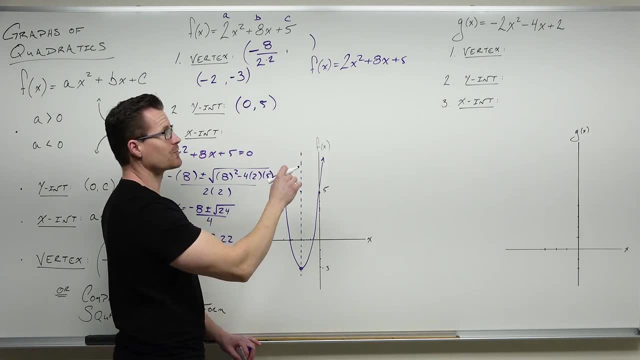 So we're going to do it. We don't need to set this equal to zero, because I taught you the way we did. So let's go through it one time on this example and one time on that example, to make sure that we have this down and we're not going to touch it again for a real long time. 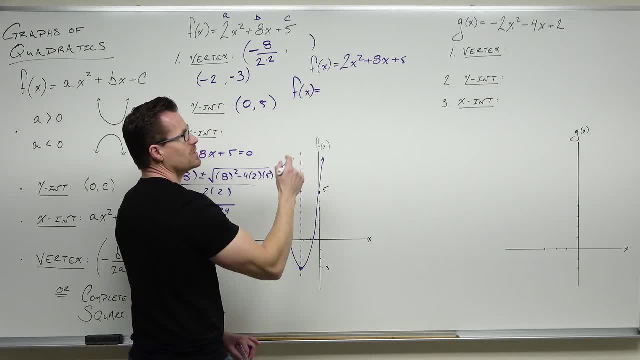 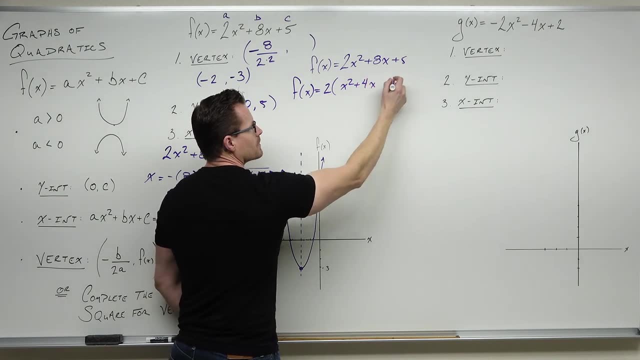 So what completing the square does? it says, hey, I need my a to be 1.. I'm going to factor out my a from these two terms. I'm not going to touch the last term. In fact, I'm going to kind. 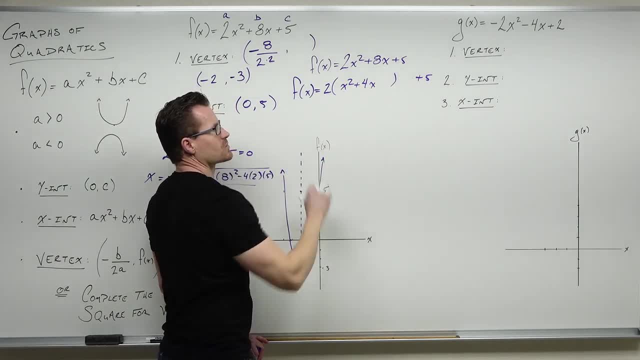 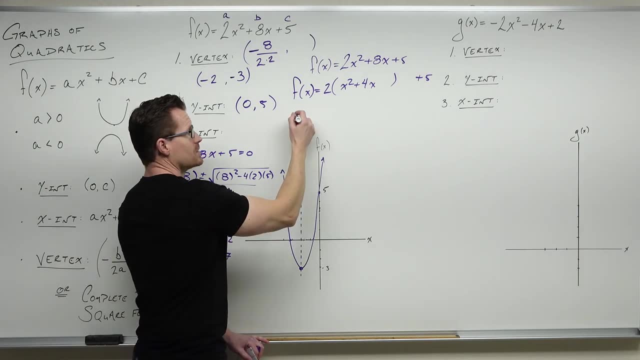 of ignore it. Not forget it, but ignore it. I'm going to leave myself a space right here And I'm going to complete this. I'm going to add something here that makes this a perfect square. What we're doing, basically, is understanding that. 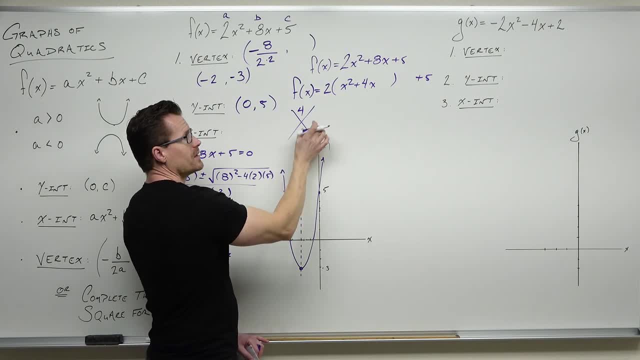 when we complete this square. we need a. we have a missing number. we need a number that two numbers add to this middle one and two numbers multiply to this last number. We're going to be adding this number in here, but we also want it to be a perfect square, so we want these two numbers to be the. 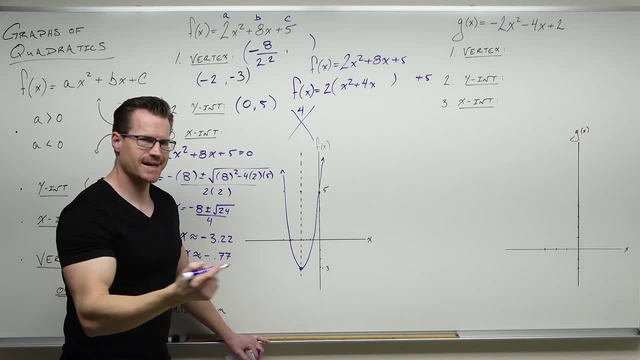 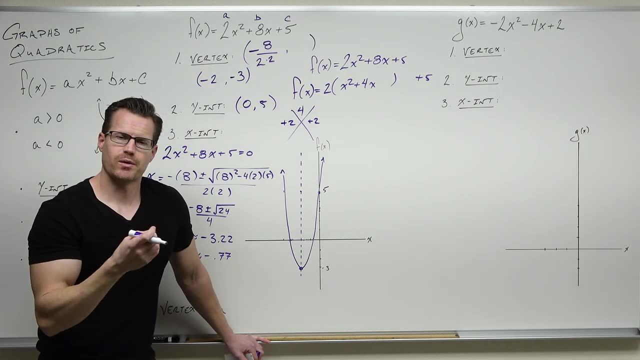 same. So we think: what two numbers are the same that add to four? It's got to be two and two. Those are the only two numbers in the world that add up to four and are the same number. So what number are we missing? Well, we're missing the number that these two would have to multiply. 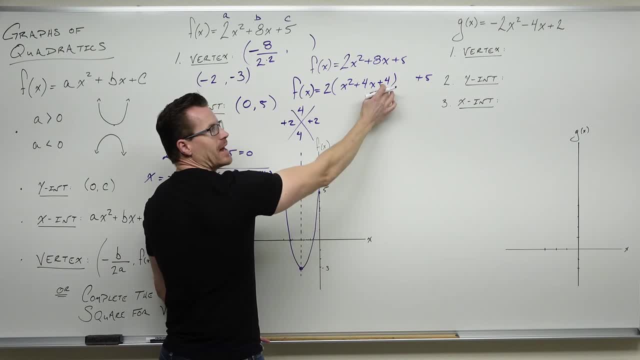 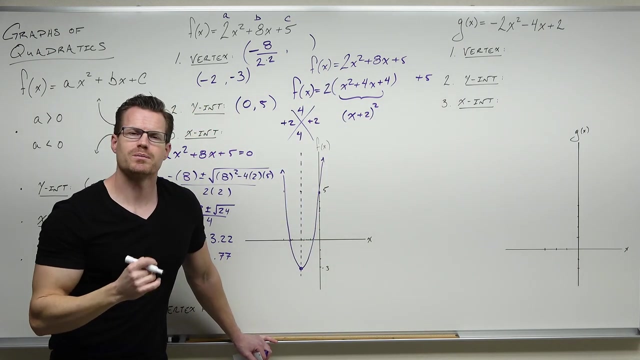 by. We're missing a four. If I add that four, it completes this factoring and it says this will eventually factor as x plus two times x plus two or x plus two squared. That's what's going to happen there. That completes this factoring. The only problem is what we've done is we've added. 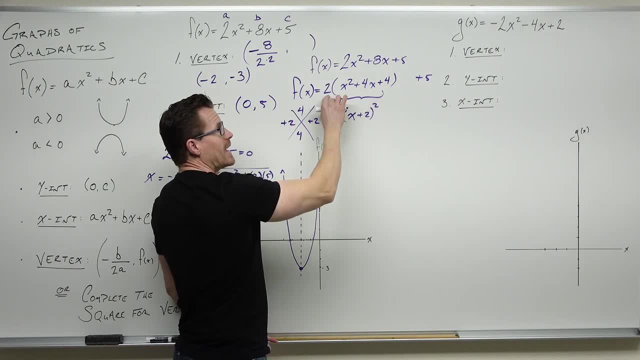 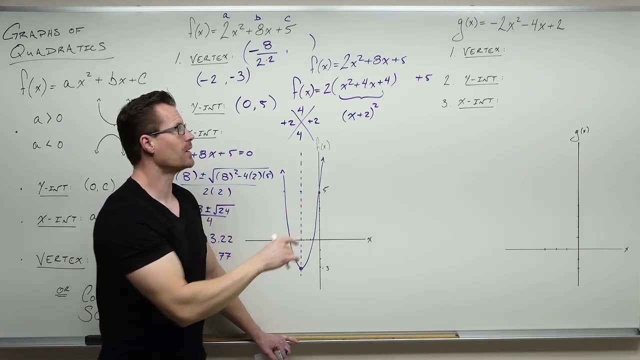 four inside of a parentheses, but more than that, something that has a two as a factor that's being multiplied by it. So in adding that four, it wasn't there before, We added it on there. In adding that four, we really increased this function by eight. 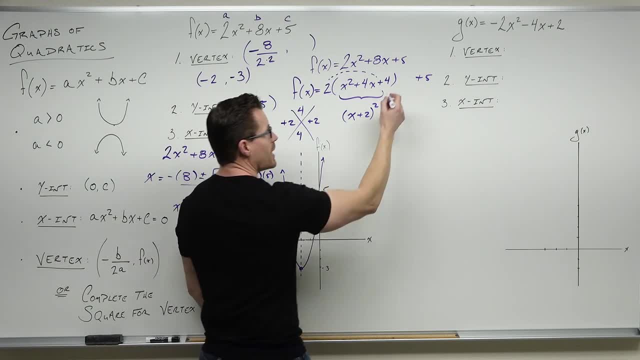 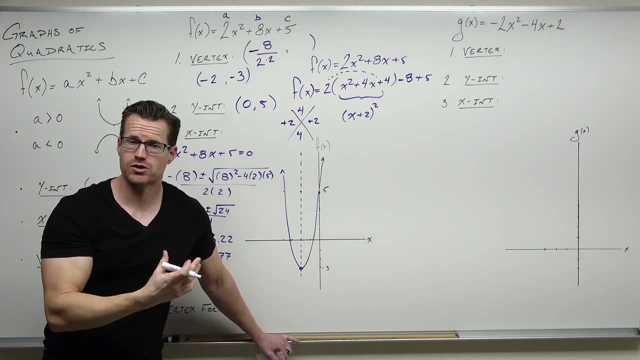 Distribute the two, You're increasing the function by eight. We have to undo that. We added eight and then we subtracted eight to make up for it on the same side of our function. That's why I taught this to you- the completing the square to you this way. 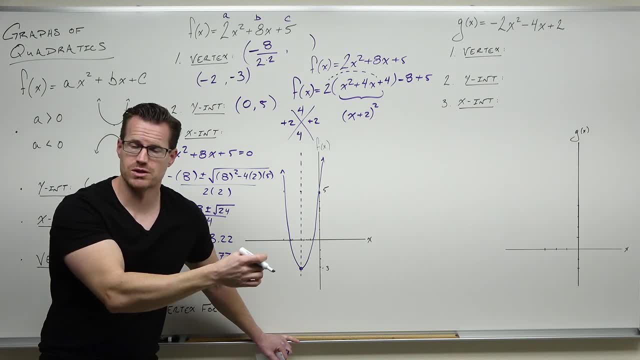 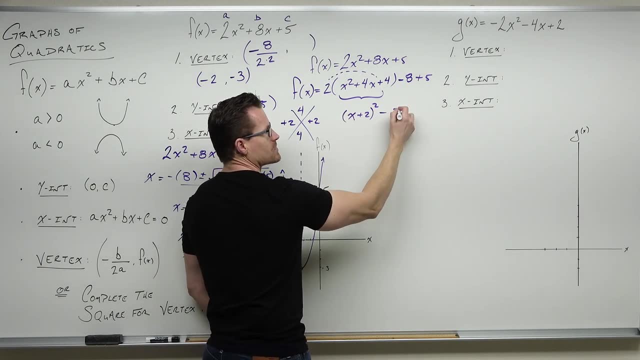 because we don't have a zero. We don't have another side of your equation to compensate for that. We're all working on one side of the function here. If we combine some like terms, this is minus three. The two stays right up front, and so our function says hey. 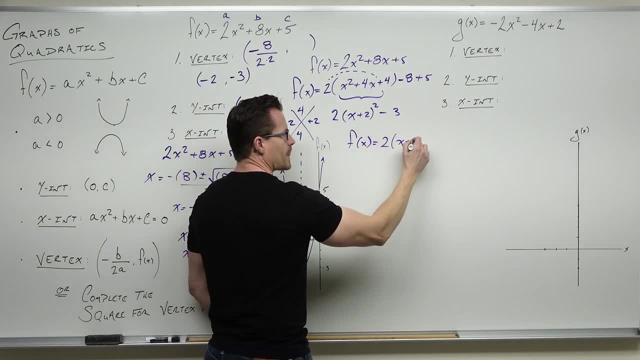 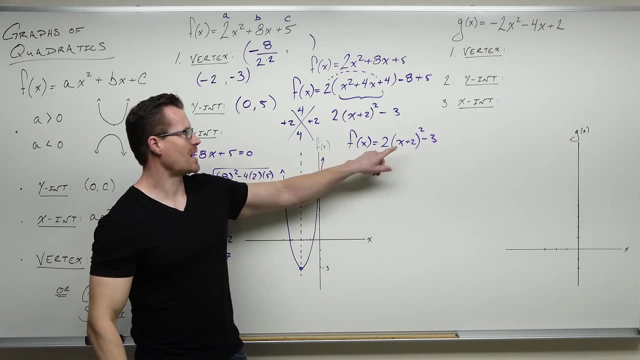 if you wanted to put this in vertex form, here's what this says: Oh man, I hope you remember our transition. This is pretty cool. This says: this is a parabola. How can you tell? Oh, it's a power. 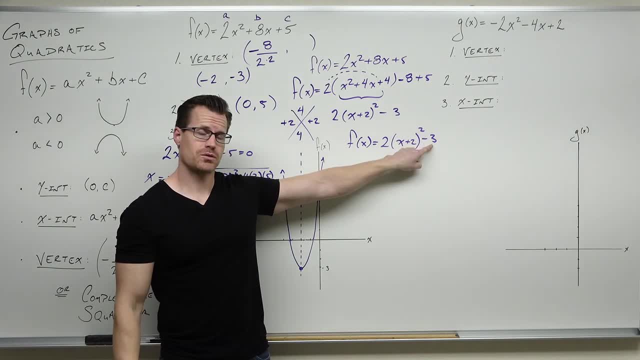 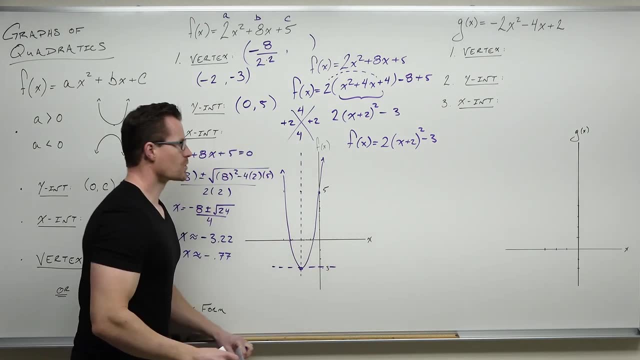 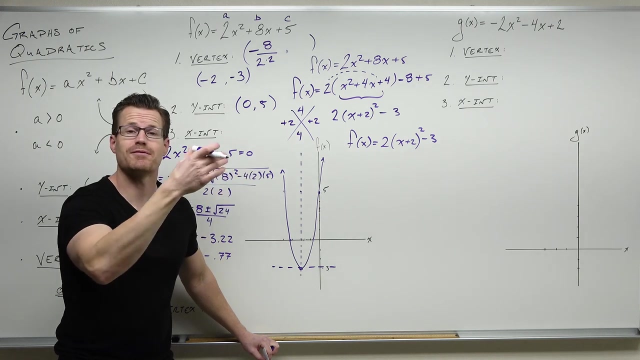 two. What's going to happen here? You're going to shift down three- Wait a minute- Down three. one, two, three. You're going to shift left. two. Remember how everything's out of your. this is opposite what we want. So the inside says left or right, but plus two would be left. 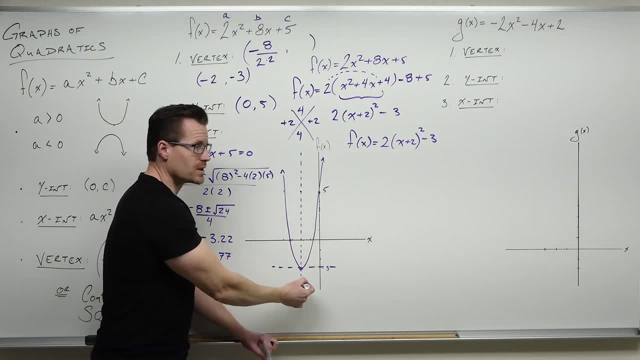 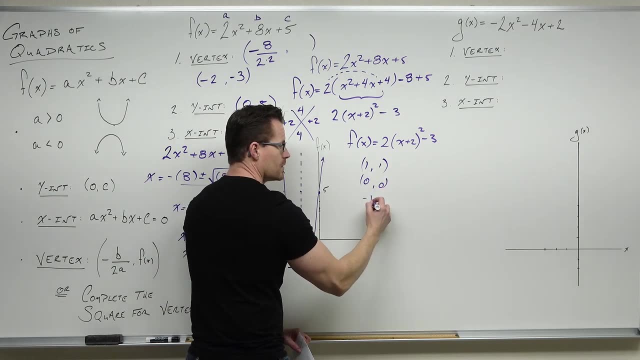 two, Left two. Oh wait, we see our axis of symmetry. That's pretty neat. We know that this is going to be narrow. In fact, if we use our key points, these are things we've covered already and we understand that. I take these key points and multiply the outputs, the outputs of them, by two. 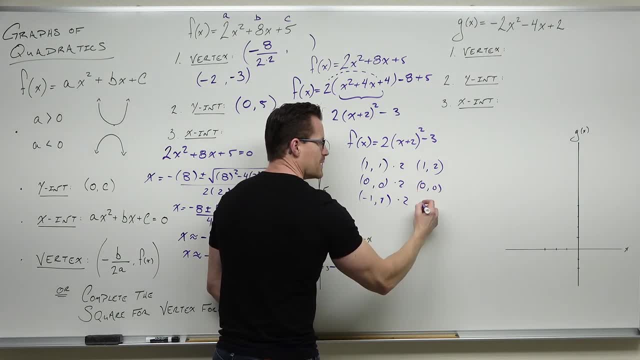 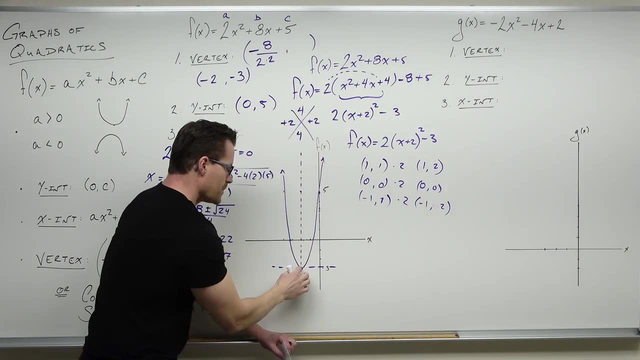 That's one comma two. That's zero comma zero. That's negative one comma negative two. I'm sorry, negative one comma positive two. So from here this would be one comma two. There should be a point there. Hey, there is. 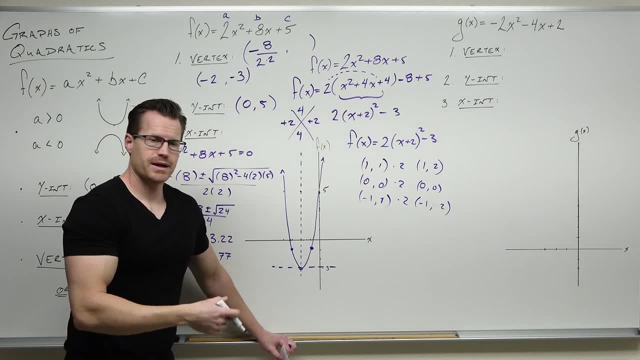 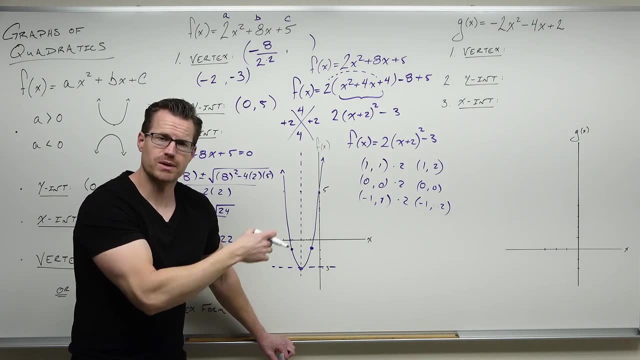 Negative one comma two. There should be a point there. There is. Oh my gosh, that's symmetrical. That's what our key points would have done by doing this whole transformations idea, doing the vertex form, If we wanted to find x-intercepts, you could set this equal to zero. 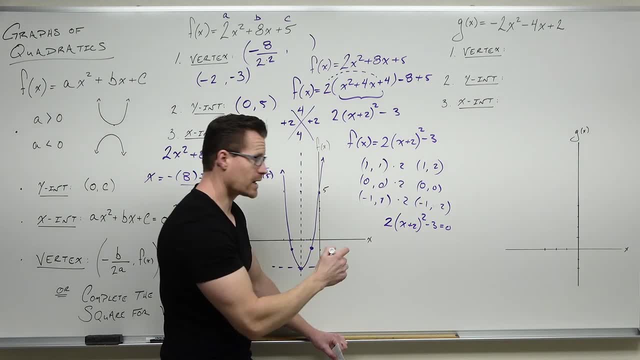 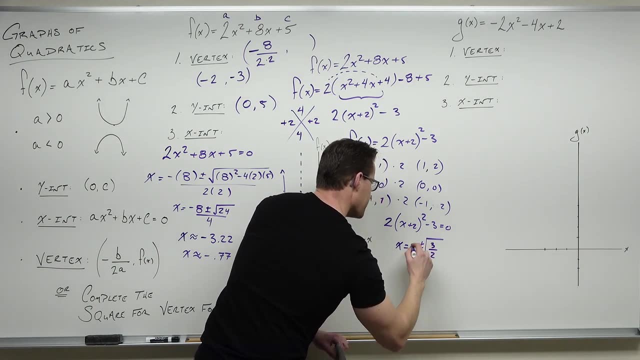 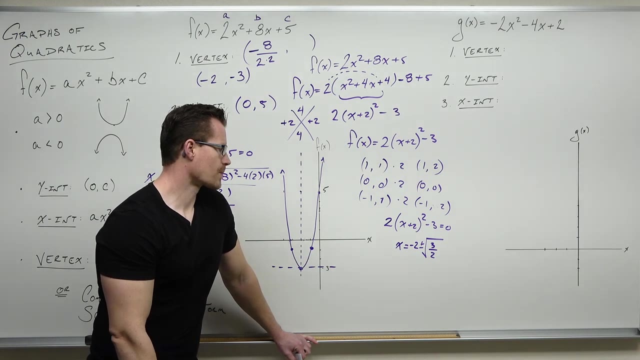 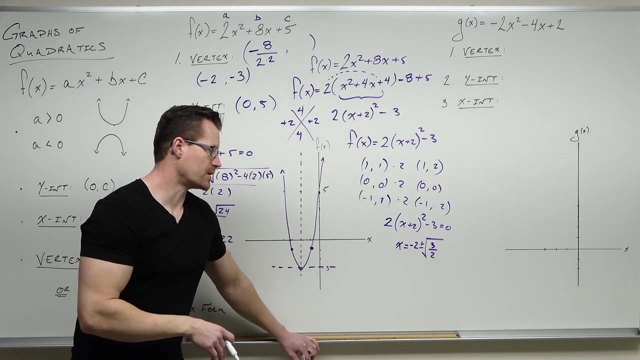 You can add three, divide by two, take a square root and then subtract two. And if we look at that as well, if let's see we add two, yeah, divide by two, sure, take a square root plus minus and subtract two. If you evaluate that on your calculator, 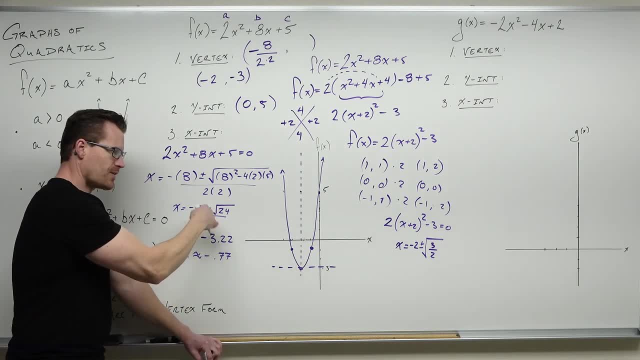 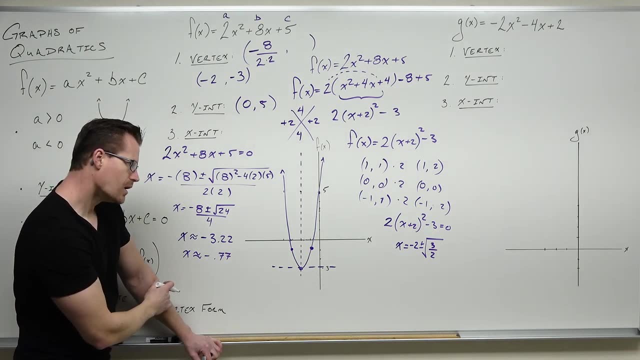 you're going to get the same exact x-intercepts as this. If we wanted to simplify this a little bit, uh, we'd have to find a common denominator. It's going to not be great, but we could certainly have done it. Uh, this would be. 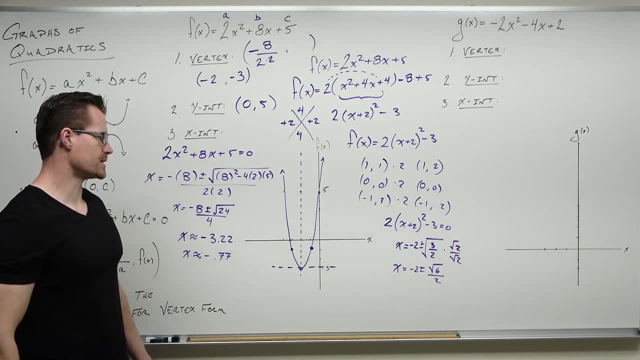 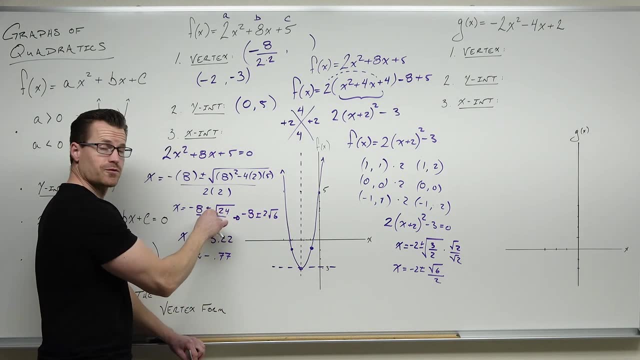 negative two plus or minus the square root of six over two. if we rationalize the denominator This right here, if we simplify negative eight plus or minus two root six, hey, that's a square root of four times six all over four. 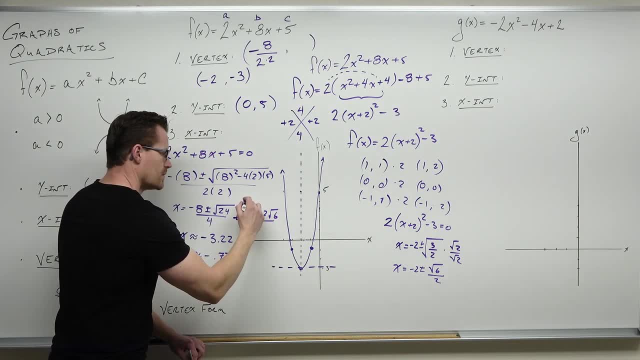 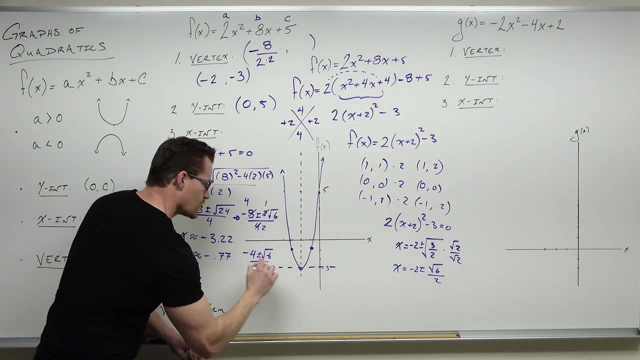 And we simplify: two goes into eight, four times into two, one time into four, two times and that's negative four plus or minus square root of six over two. So why do they look different? This is written as two fractions, So if I separate this negative four over two plus or minus square, 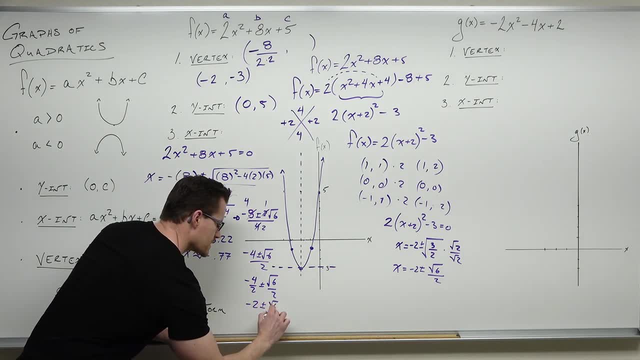 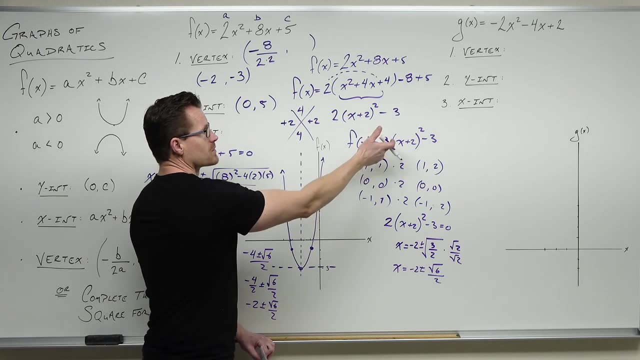 root of six over two. this is negative. two plus or minus square root of six over two. It's the same exact thing. It's representing the same exact x-intercepts. If you want to find the y-intercept, you'd have to plug in zero or go back to your original and say it's still going to be zero. 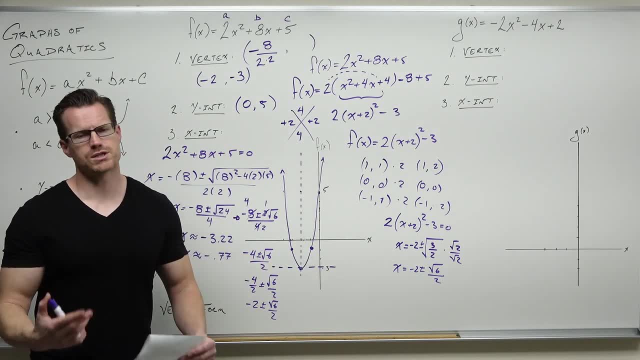 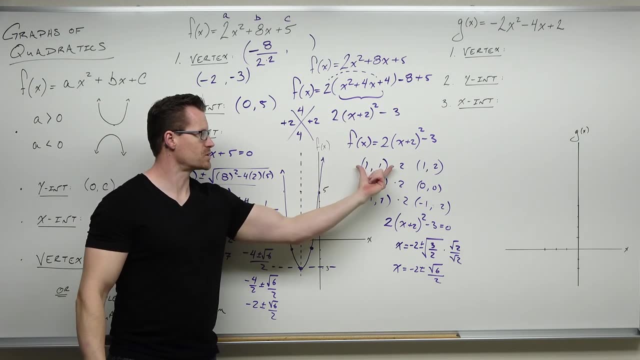 My idea here is just to tell you that this stuff all works together. So whether you want to do the vertex form and complete the square, no problem, You can still use key points. You can find x-intercepts, You can find y-intercept, You can find the vertex. Very easy. This is down. three, left two. 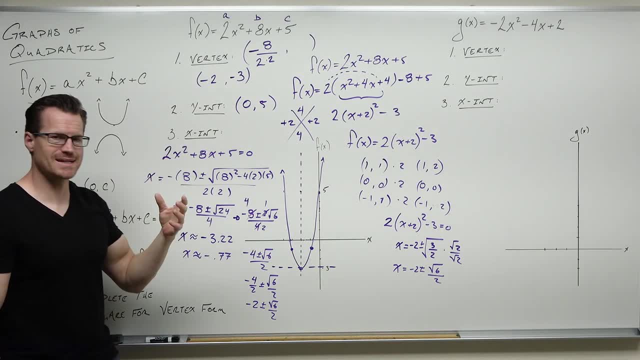 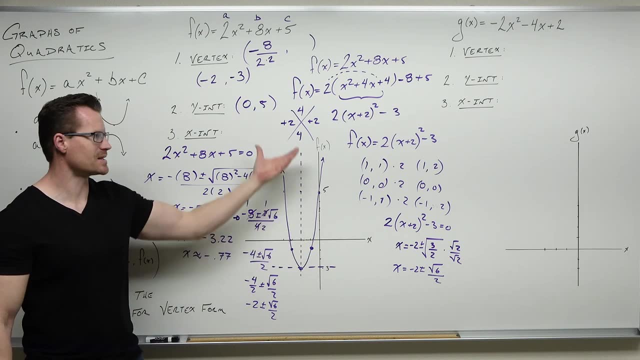 This says down three: left two: That's exactly the same thing. You're talking about the same vertex. The minimum height is still negative. three: The maximum height is infinity. This goes on forever. We can find x-intercepts either way. We can find y-intercepts either way. 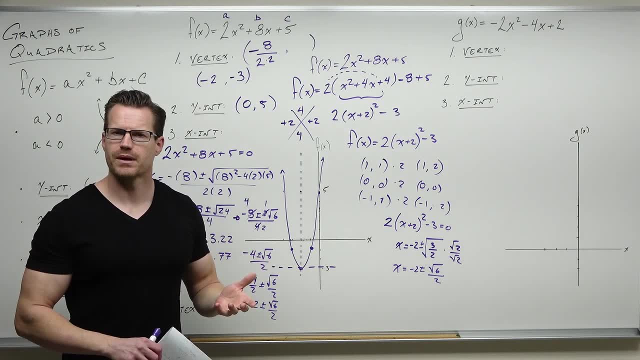 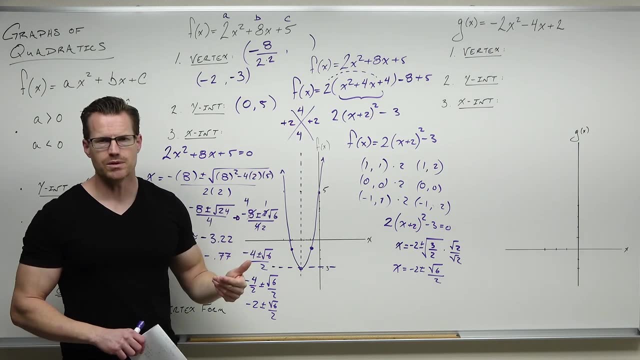 It's really up to you. Now. which way do most people prefer? Most people prefer this one, because you don't have to touch completing the square, Because this gets really difficult. if I didn't give you easy numbers, I gave you easy ones here. I gave you eight, which was divisible by two. 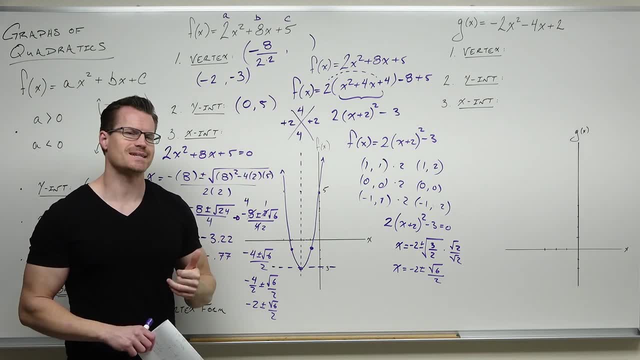 and then created a four which you can separate and divide that by two very nicely. So if that's not the case, this becomes fairly challenging. We saw that when I taught you how to complete the square. So, anyway, I hope that I've made sense of it. If you have any questions, please feel free to. 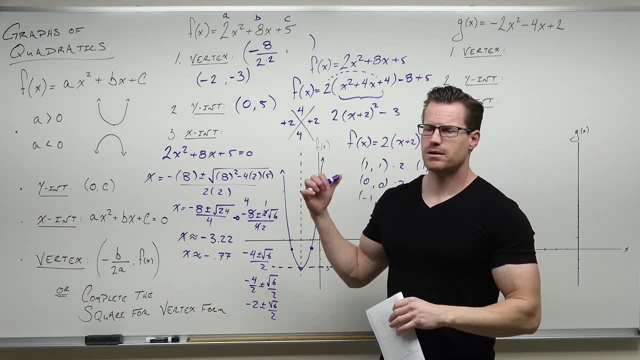 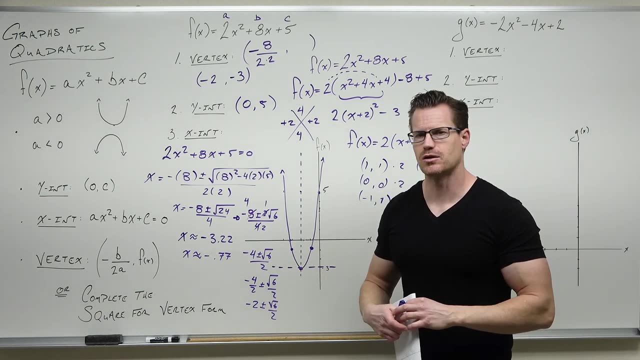 to you on this example. This is the longest one we're going to go through. Later on the rest of them, we're going to do basically this: I'm going to very quickly complete the square to verify the vertex and just to practice that a little bit, and then that's it. So at this point we need to. 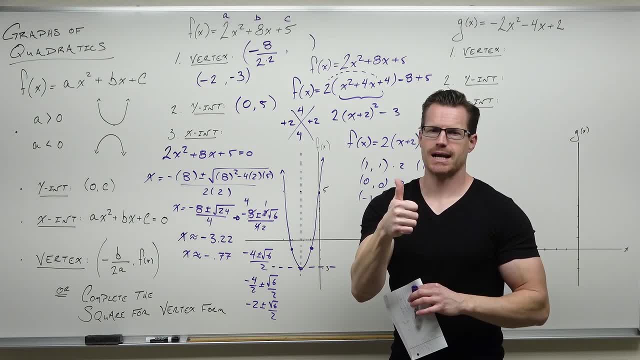 understand. the vertex comes first. Every parabola's got it, We got to find it. The y-intercept comes second. Every parabola's got it, We got to find it. and we have to use it across from the axis. 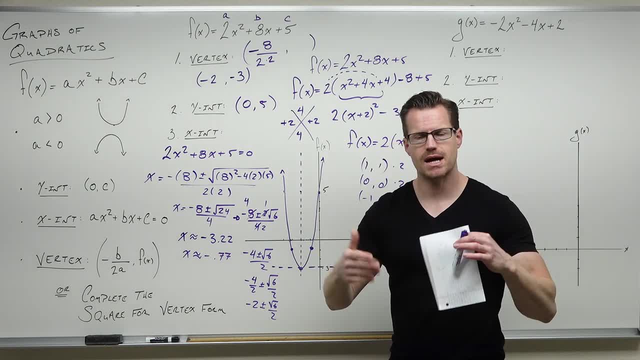 of symmetry to find our symmetrical point. Then if we're going to cross the x, then we find x-intercepts. So we're going to come back and we're going to do this. So we're going to do this, We're going to. 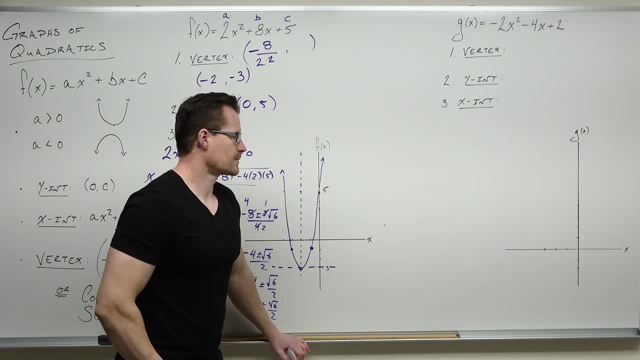 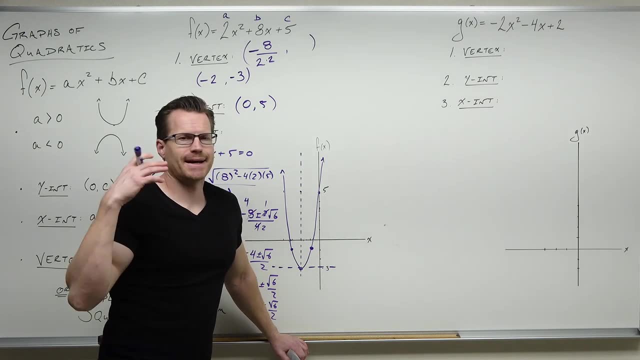 go on another example in just a second. Okay, let's continue. So we're looking at g of x. We have negative 2x squared minus 4x plus 2.. The first thing we got to notice is: well, what's? 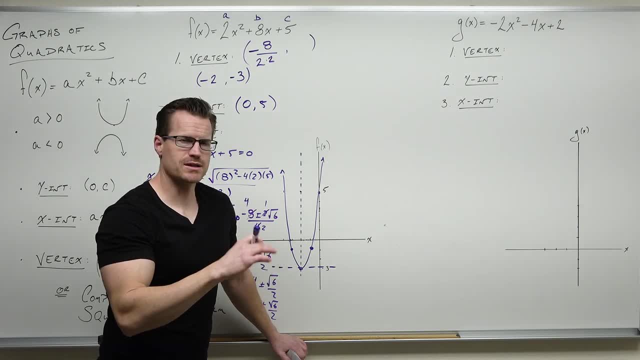 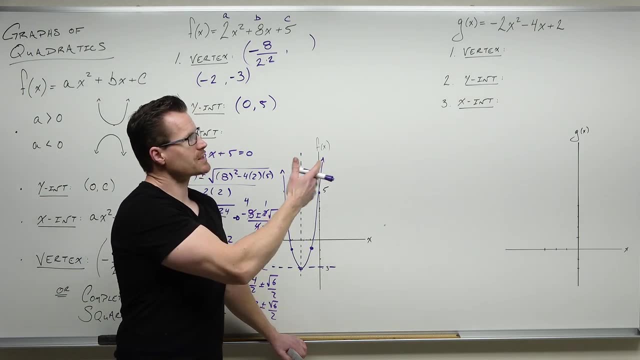 its shape. Its shape is it's got a power 2. That's the largest power. It's a polynomial-type function. This is going to be a parabola Now. is it going to be upward opening or downward opening? Because that's in order. it's really easy to identify that this negative 2 in front. 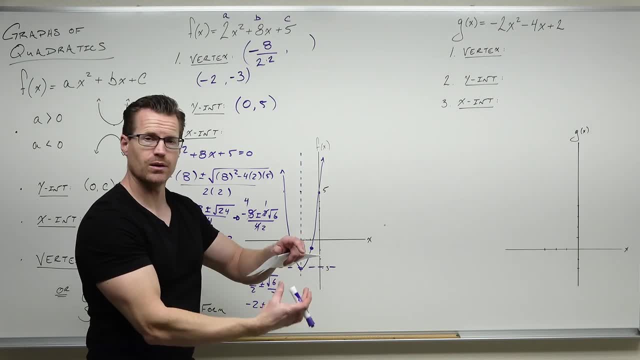 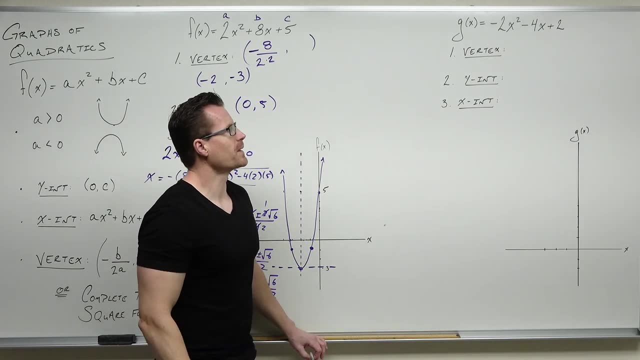 of x squared, It's going to make it a downward opening and fairly narrow. So we're going to draw a parabola. It's going to be this vertical stretch because the absolute value of our a is more than 1. So that's a little bit stretched out. Here's what we're going to practice. 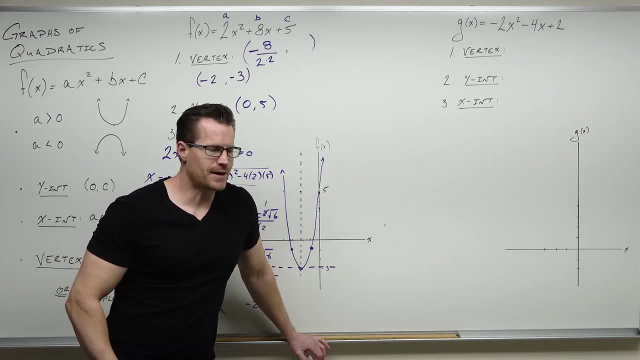 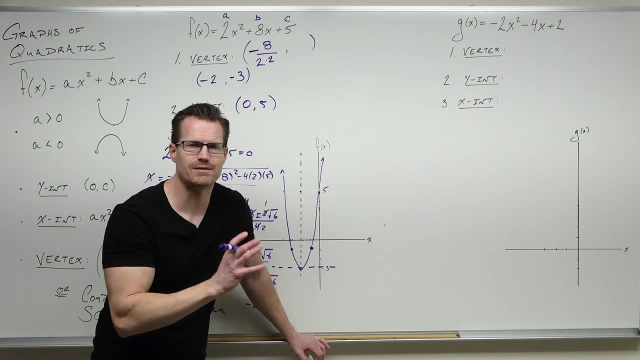 We're going to go through and find the vertex first, then our y-intercept, then our x-intercepts. if we have to, Then I'll show you the vertex form if you need to find that, and we'll just make sure that they're giving us the same thing. So let's start with vertex, Because 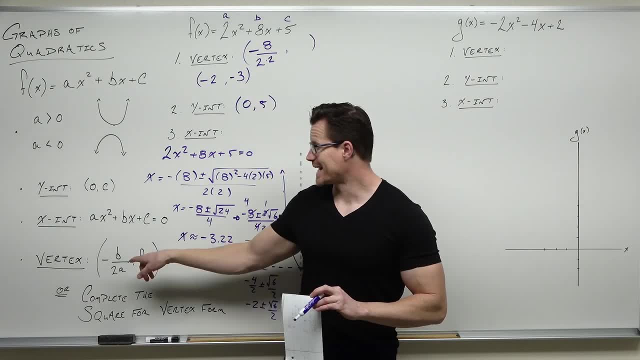 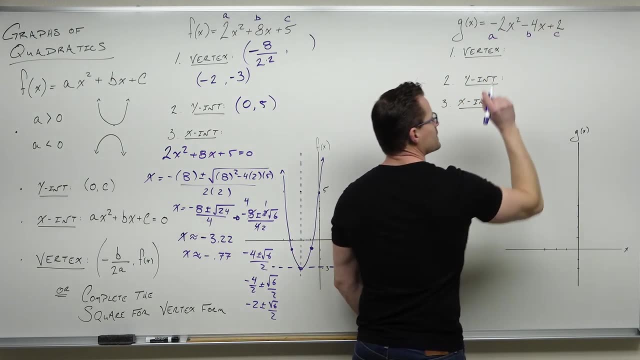 every parabola in the world has a vertex. this formula comes in really handy. Our formula for the vertex is: we're going to find the x-intercept. So we're going to find the x-intercept Based on our a, b, c, a being negative, 2 and b being negative, 4 and c being positive. 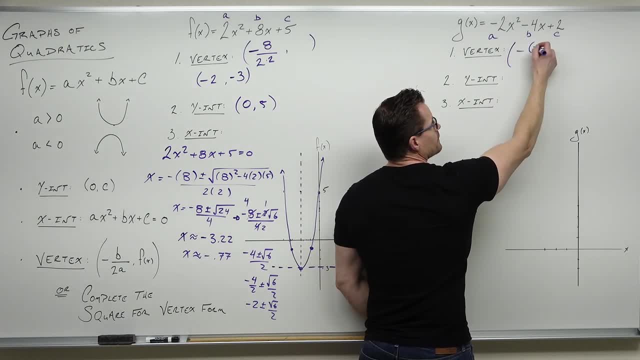 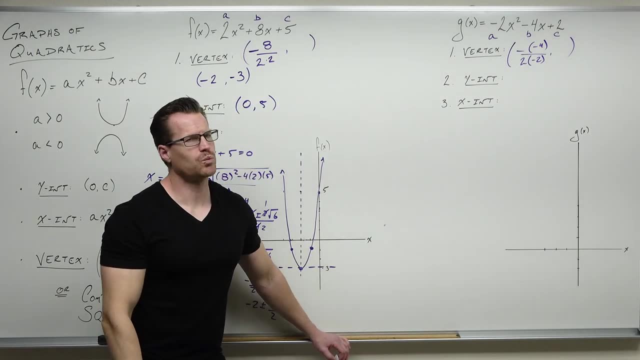 2, we're going to find negative b all over 2 times a. We've got to be real careful with signs. I oftentimes will use parentheses here to represent the sign, to represent the fact that we need to have that negative and it maintains operation. 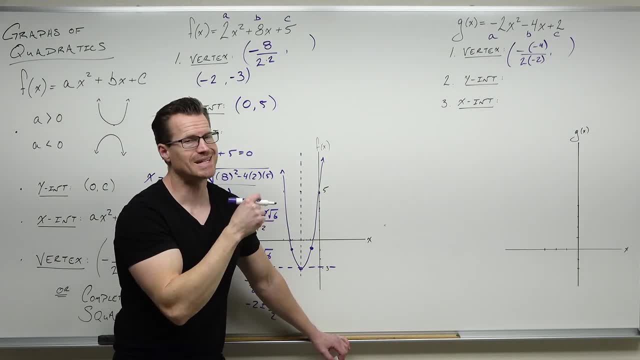 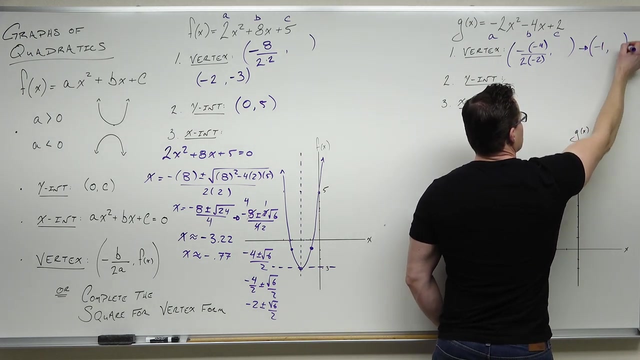 It's negative, negative 4.. All over 2 times a, that's 2 times negative 2.. We can't forget those negatives. We're going to simplify it. So: negative, negative 4, the opposite of negative 4, that's positive 4, but we're divided by negative 4.. That's negative 1.. Now to find. 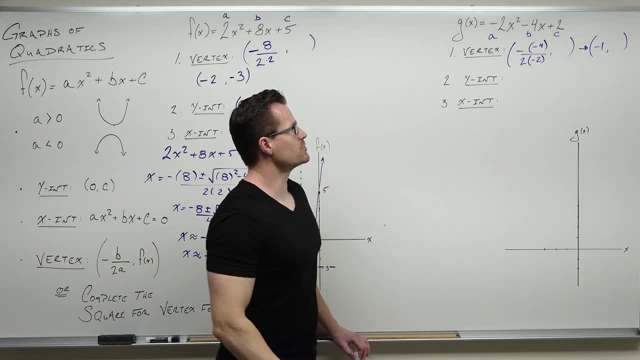 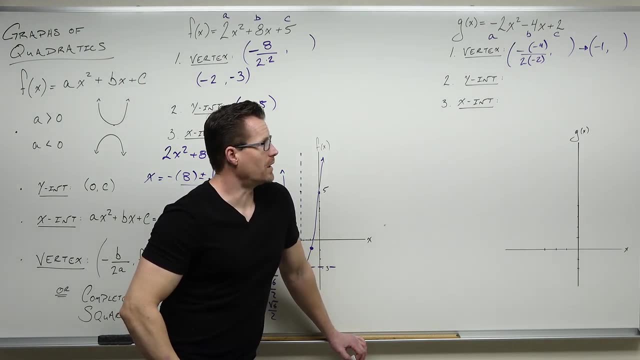 the y-value. we're going to take that negative 1, we're going to evaluate it. Put it right back in g of x to find the y-coordinate. So when we plug in negative 1, let's see: Negative 1 squared is 1 times negative 1.. Negative 1 squared is 1.. Negative 1 squared is 1. Negative. 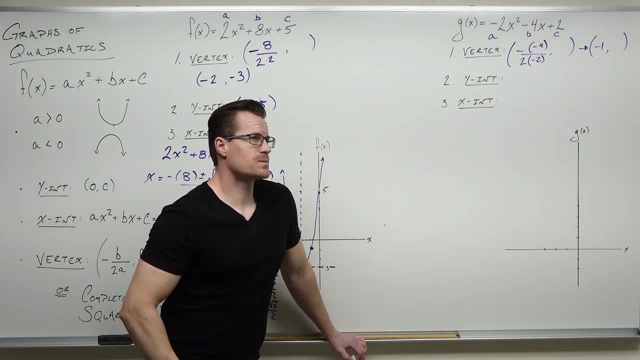 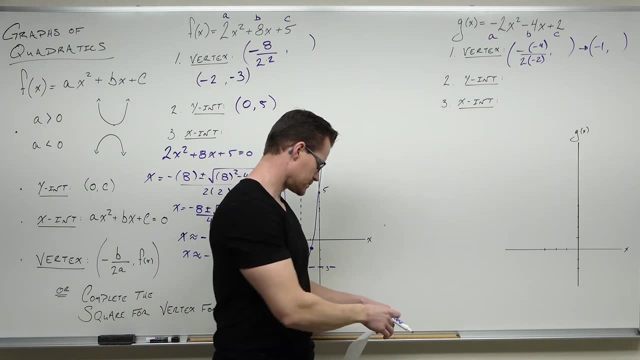 2, that's negative. 2. Minus 4 times negative: 1. So negative: 2 plus 4, well, that's, 2 plus 2 is 4. And we're going to take that vertex and we're going to plot it right now. So negative. 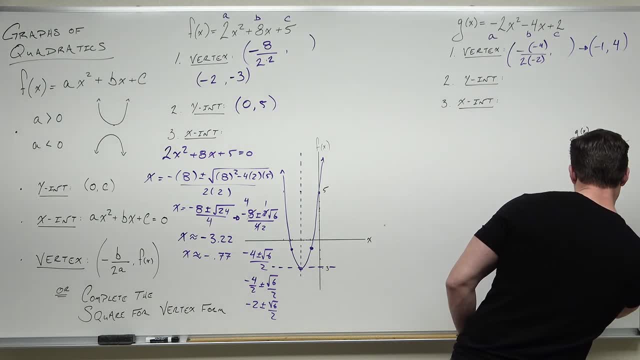 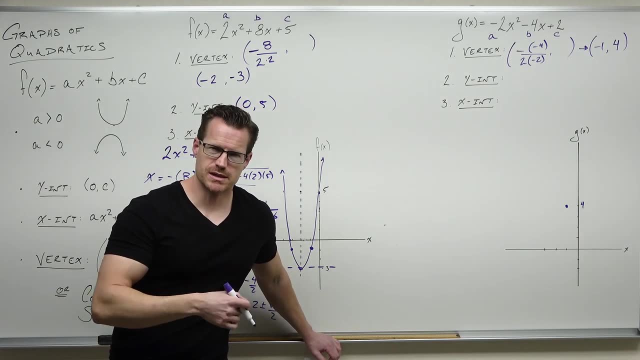 1 comma 4.. Negative, 1 comma 4, right about there. And we're going to determine something right now. Because this vertex is above the x-axis and because it's downward, it's going opening In our heads. right now we're thinking I'm going to have to find x-intercepts or at 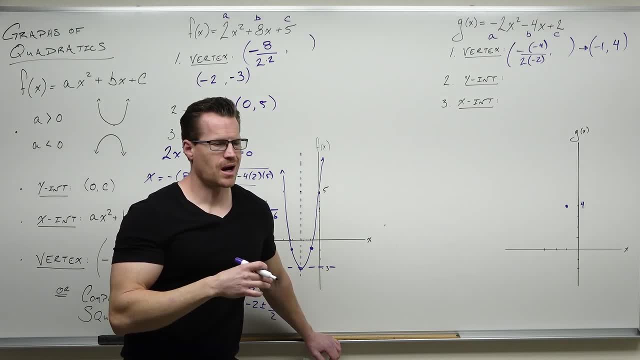 least an approximation for them. So I'm probably going to be factoring, I'm probably going to do in quadratic form, because my vertex is above the x-axis and it's downward opening. The parabola is going to cross it. We've got to find that The only time we don't is: what if this had been? 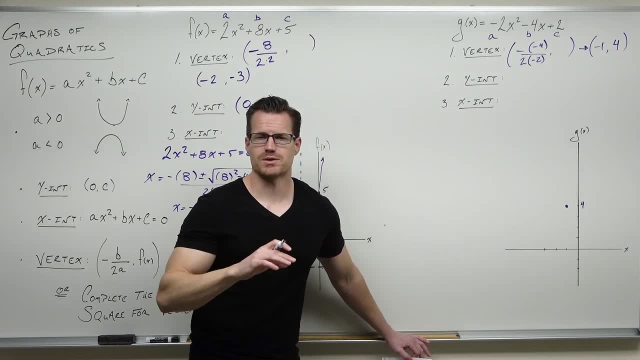 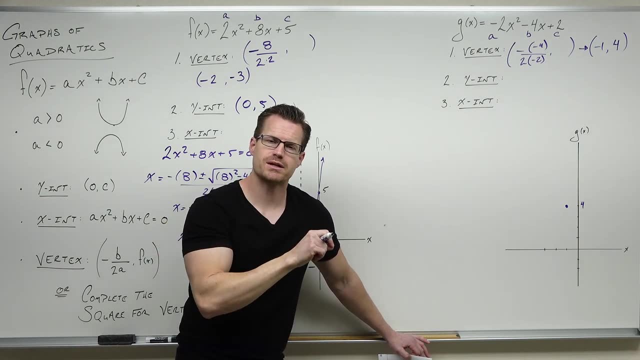 upward opening Man, we're golden. We don't have to find x-intercepts at all. The other thing we're going to talk about right now is the maximum, Because this is a downward opening parabola. that vertex represents the maximum height of your parabola, of this function. So if you were 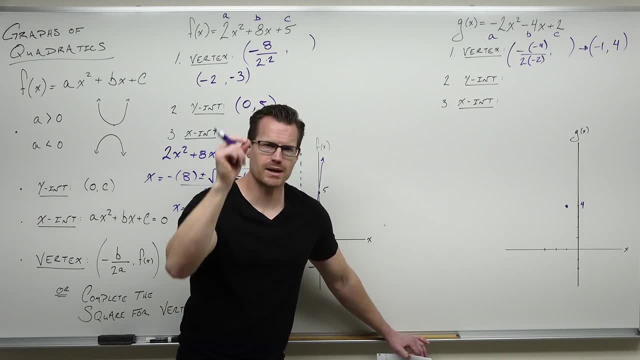 asked: hey, this is a picture of a ball going up and coming down, which it's not. How would you find the maximum height? Well, you'd find the vertex, So you wouldn't even do any of this if that was your question. Just find the vertex, The maximum height of a downward opening parabola. 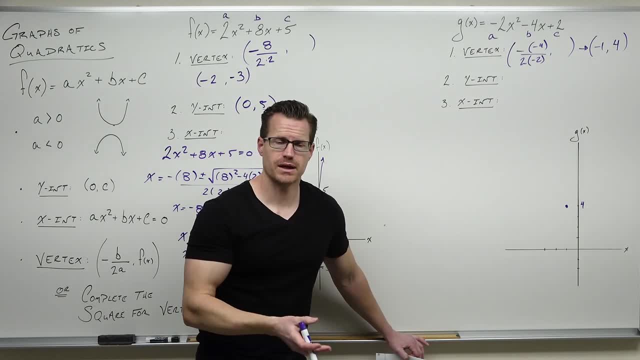 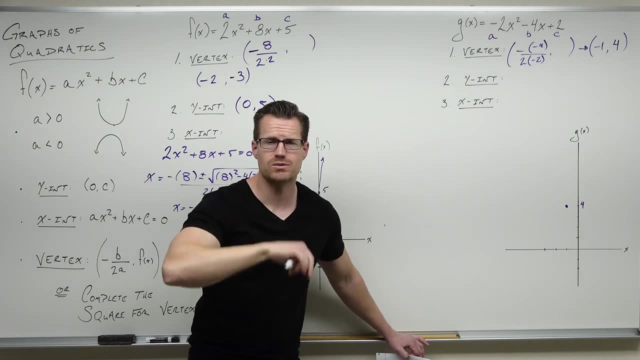 happens at your vertex, So your maximum height would be four. It occurs at: x equals negative one, but your maximum height would be four. That's the highest value. This function contains the highest y value that you get. It's four on us. All right, So we know. 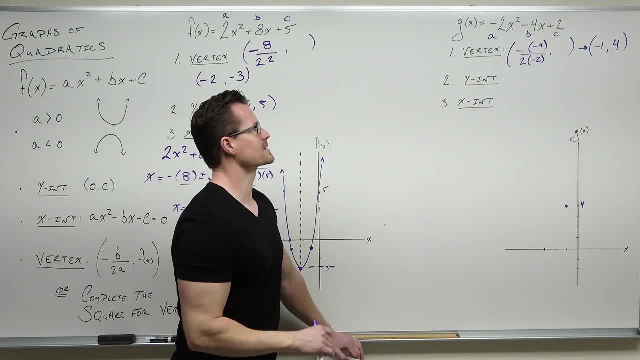 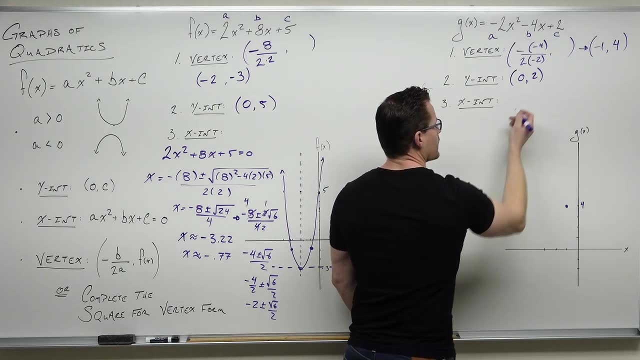 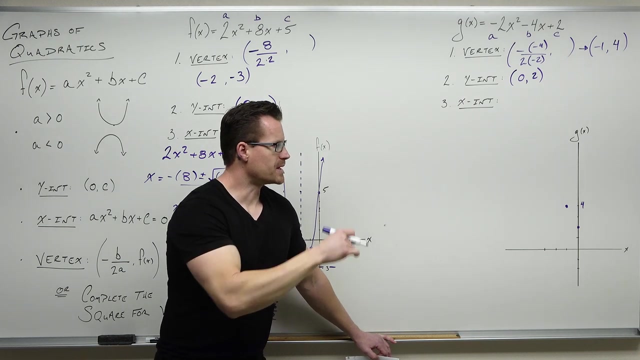 that We know that every problem is going to y-intercept. So we take like two seconds to say: if I evaluated for x equals zero, my y value is going to be two. And I'm going to pull up that Right now before I forget. I'm going to make sure that because I have that axis of symmetry. 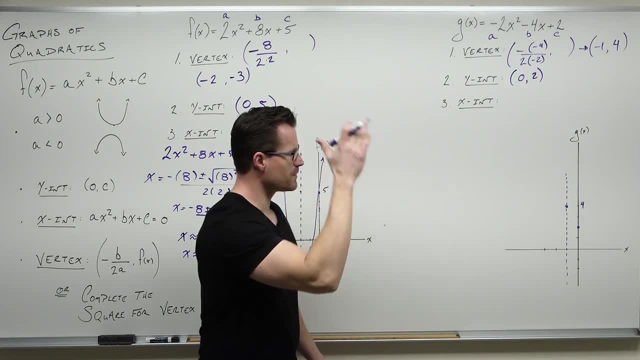 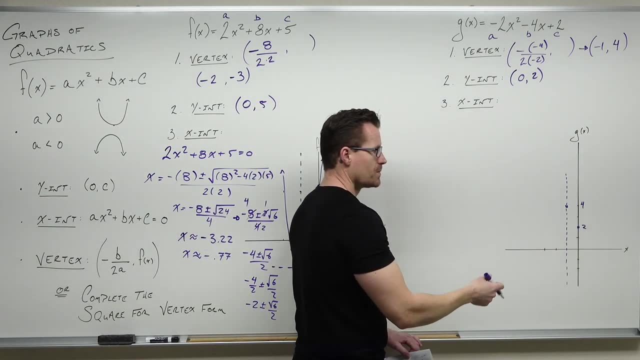 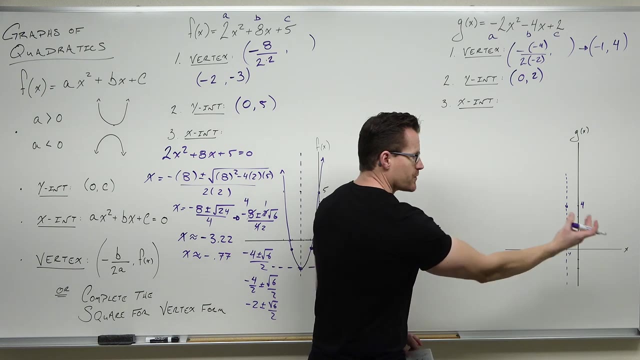 that always goes right through my vertex. I'm going to use that y-intercept to give myself a symmetrical point. So I know that at this two, this value of two, I'm at zero comma two. there I know that's one unit. This is negative one, One unit away from the axis of symmetry If I go one. 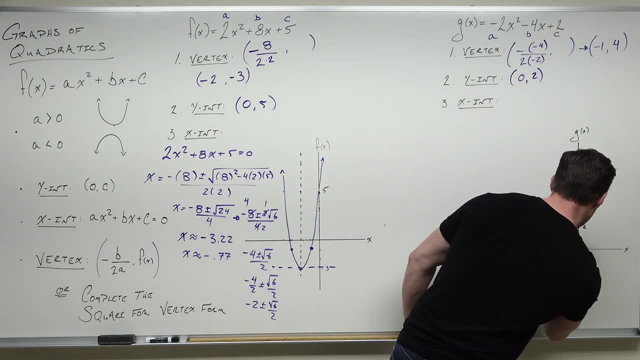 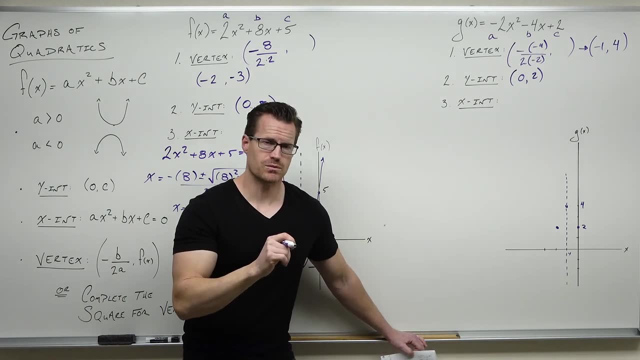 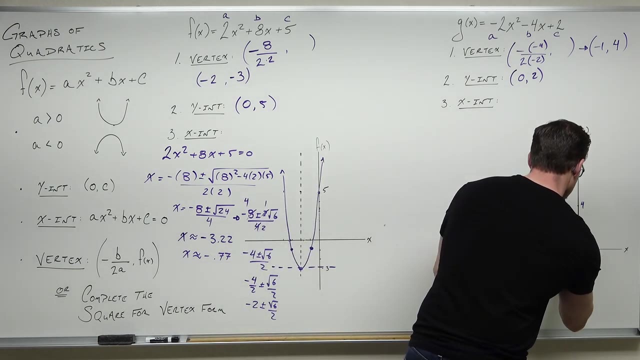 more unit at the same height. well, on the opposite side of the axis of symmetry. I'm going to have another point, due to the fact that this is an even function. well, based on the axis of symmetry, It's a symmetric function, about that. So we found the vertex. No problem, We know we're. 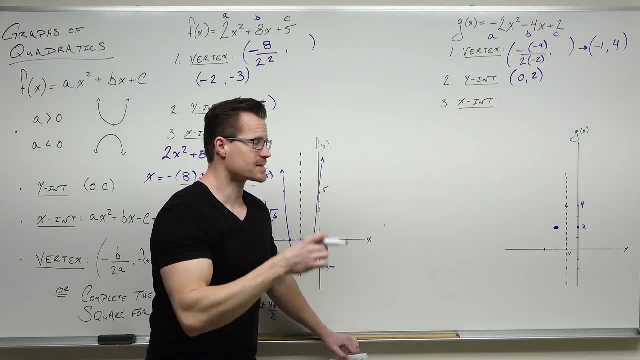 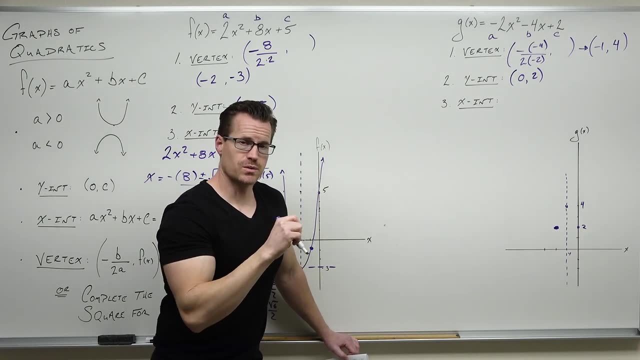 going to have x-intercepts. We're going to find them. right now We find our y-intercept. We use axis of symmetry. We know it's downward opening And now, because of that, we know this is going to cross the x-axis. So we're going to do two things: We're going to use, we're going to set. 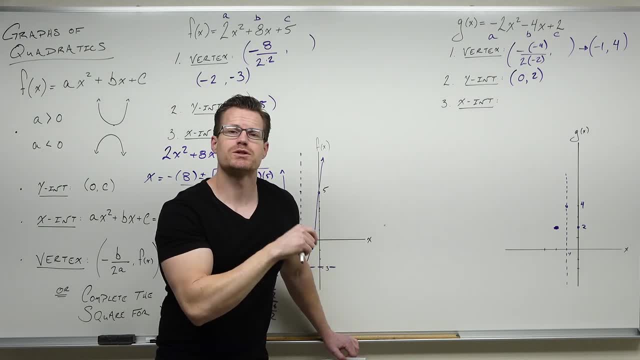 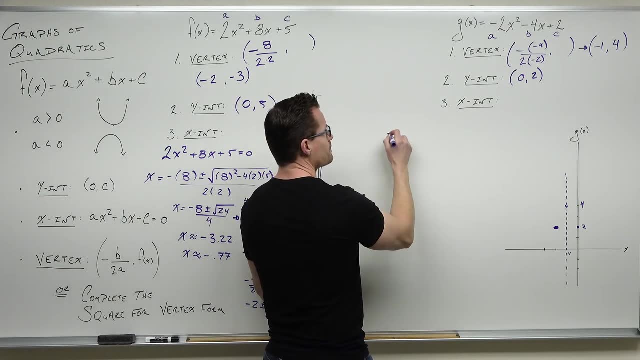 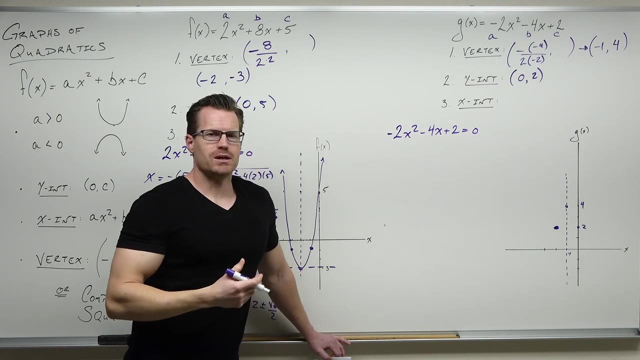 this function equal to zero and find the x-intercepts, And then we're going to determine whether our approximation is accurate in equal distance from that axis of symmetry. So we set this equal to zero. You know, we can't forget that we can do nice things, Like, if that's. 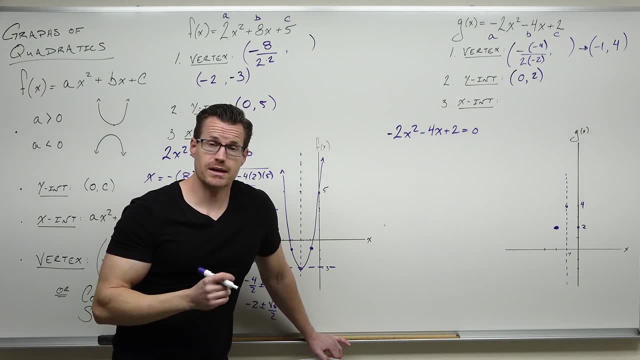 set equal to zero, we can try to factor, at least set it up for factoring, because it also helps our quadratic formula by having smaller numbers or at least less negative numbers. So what I mean by that is: don't forget that when you're, when you're finding x-intercepts, it doesn't care if your 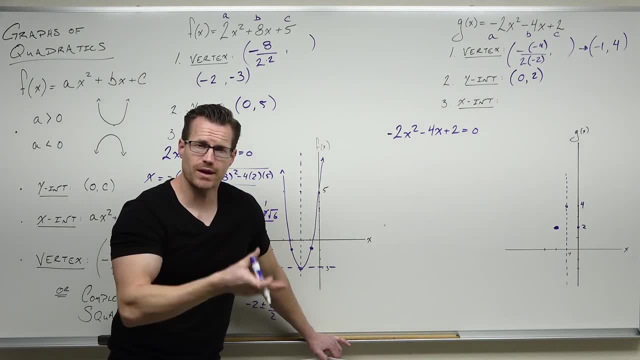 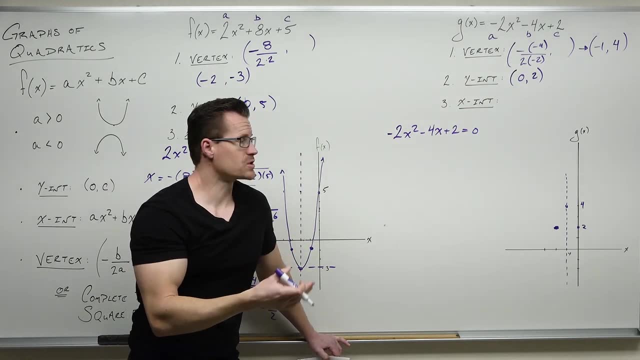 first term is positive or negative. It doesn't care about the signs of it. If you reflect this function, don't do it now or don't do it over here like before, But if you do it now, your x-intercepts won't change, And so what we would do is we'd factor this, Let's factor out negative two. 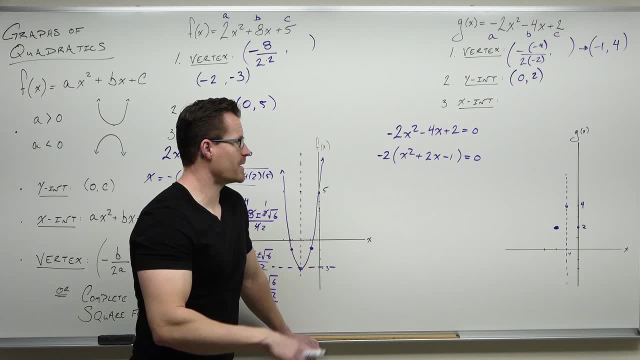 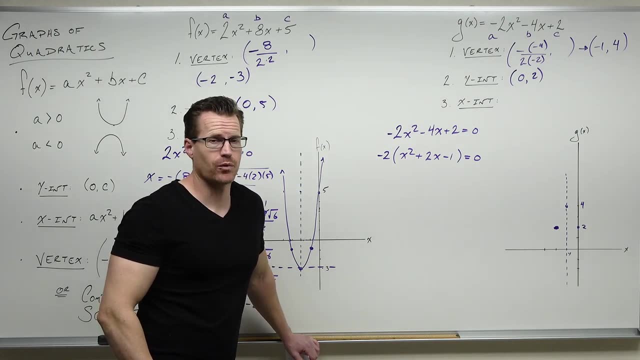 That at least gives us something nicer to look at for factoring. Now, when we think about it, man, it looks like it should be factorable, but we can't add the positive two and multiply the negative one. That's that's not going to happen for us. 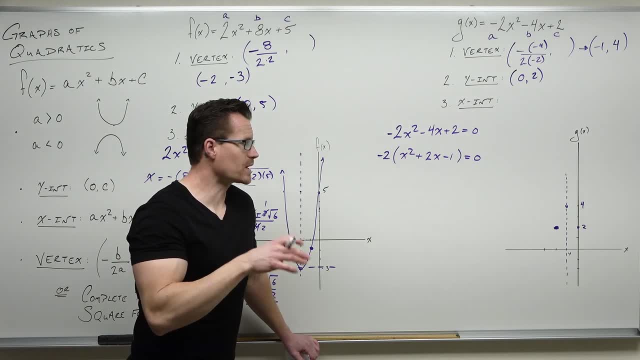 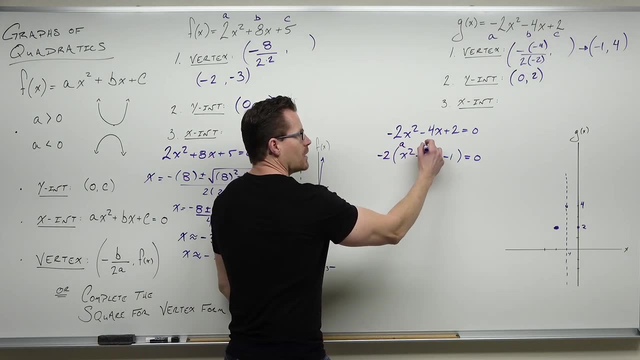 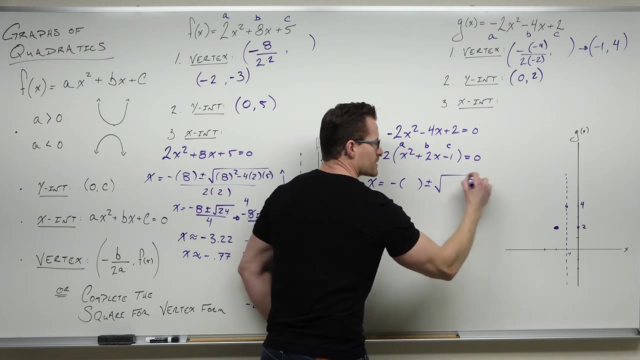 And so our best choice here, because factoring is not going to work, I really don't want to do completing the square right now. The quadratic formula is pretty much it: Our a would be one, our b is two and our c is negative one. So x equals negative b, plus or minus. we got a square. 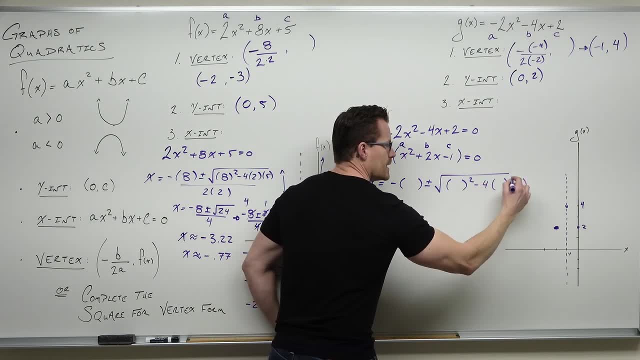 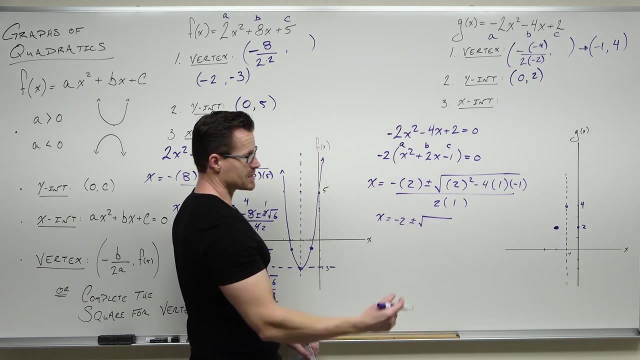 root b squared minus four, a, c all over two, a. then we fill it out: B comes first, a comes second, c comes last. I know that we have x equals negative, two plus or minus square root of eight all over two. 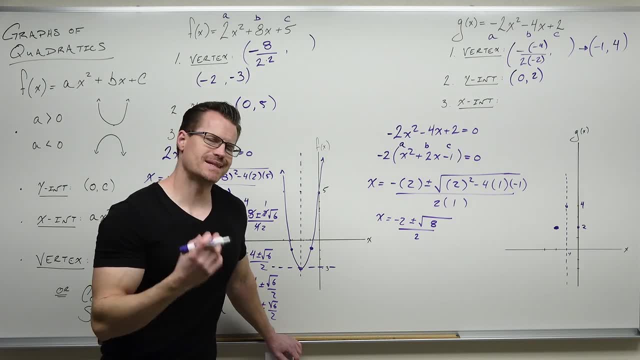 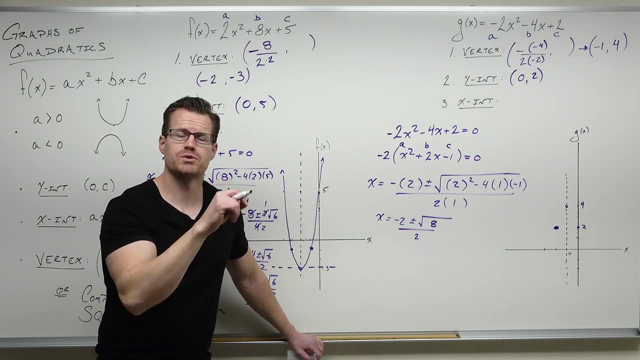 Can you simplify it? Yeah, you sure can Do you have to. It depends. If you're asked for an exact answer, then yes, You'd want to simplify this as the square root of four times two, so two root two. 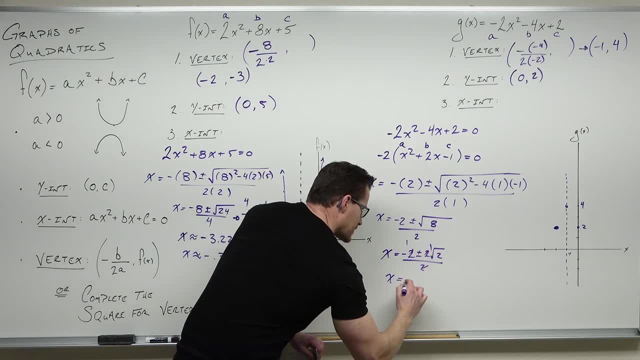 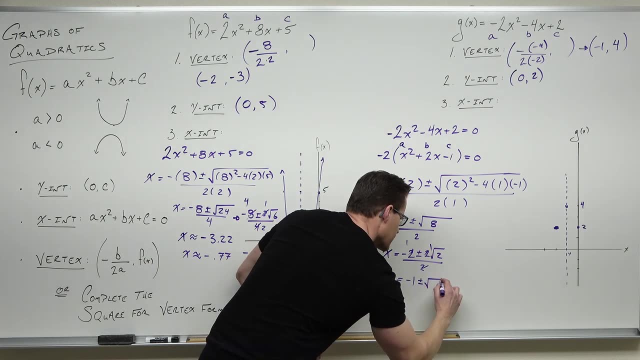 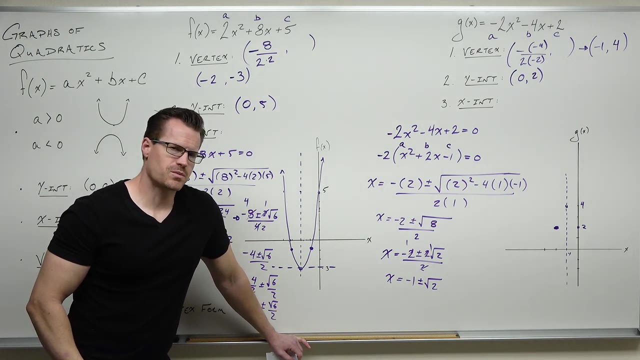 And then we can simplify By factoring, or understanding the reason why factoring works, and simplifying all three of these coefficients or constants, as the case may be, And you get negative one plus square root two and negative one minus square root two. That's almost easy enough for us to approximate our 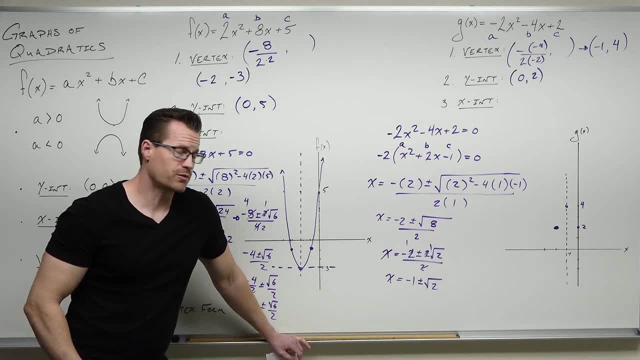 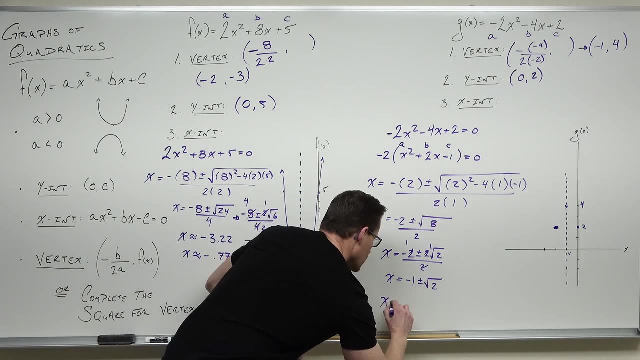 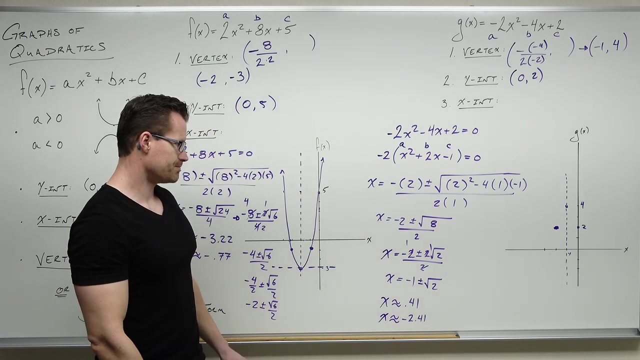 head. if you know, the square root of two is one point four one. So if we do that well we go okay. negative one plus one point four one is approximately point one minus one point four. Forty four nine zero minus one point four one is negative two point four one. That's what we're gonna put on our x axis is as close as we can. 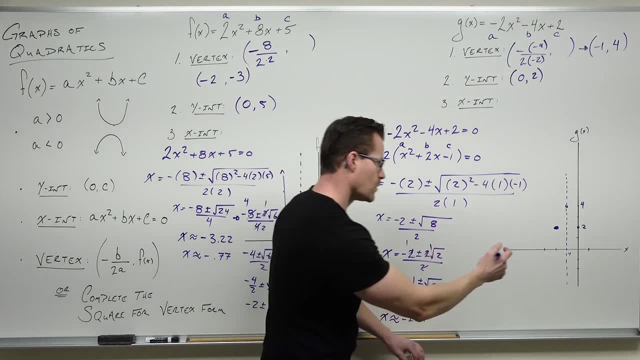 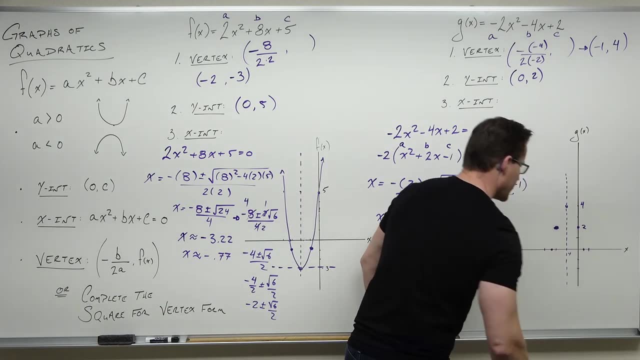 So let's see Negative One, negative two, point four, one negative one, negative, 2.41, and then point for one that's positive. Man, that looks about right, That's 1.41.. 1.41 on each side of the axis, symmetry. so I know that we're symmetrical. 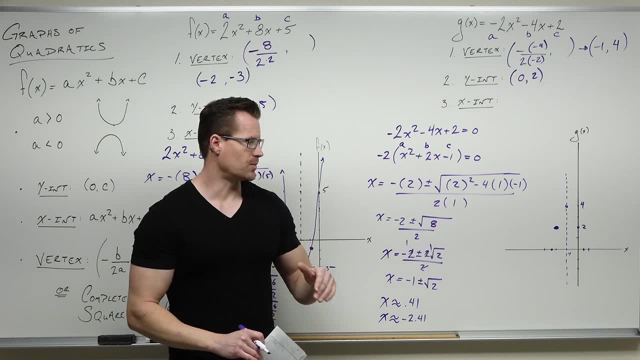 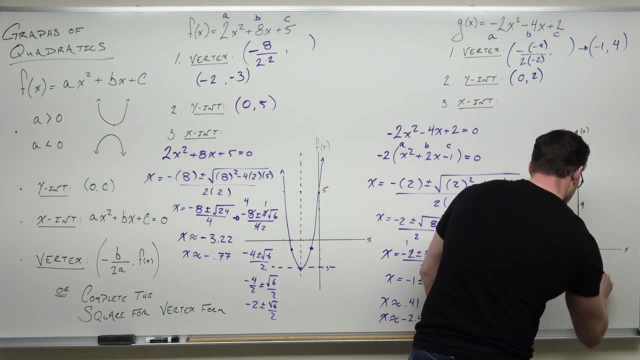 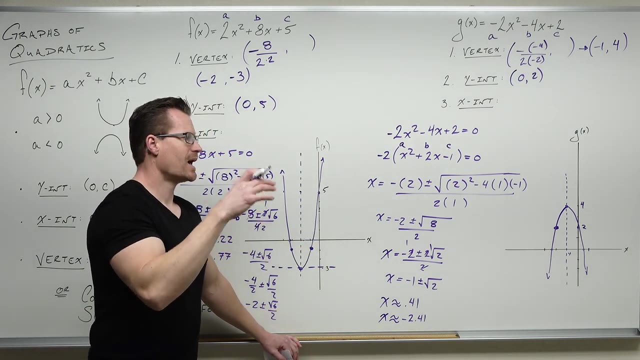 That's probably a really good indication. we got this right, And now we're going to graph our parabola using those five points As symmetric as possible, using the vertex y-intercept, second with axis symmetry free point, and then your x-intercepts, if you have them. 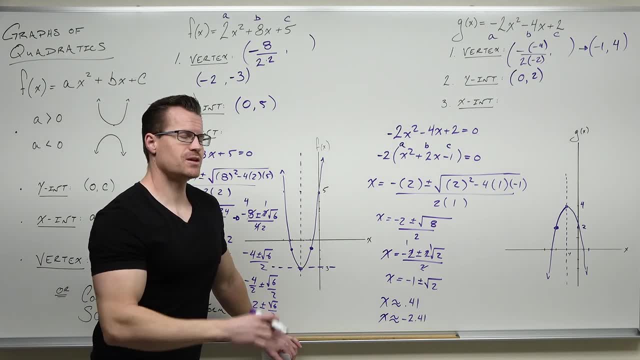 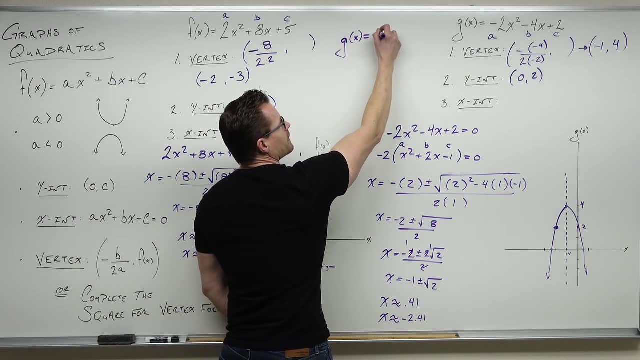 Now, I did promise you that I was going to do completing the square. Just to make sure that we have that right. if you have to do vertex formula, here's what we would do. So for our g of x, remember we don't have two sides to work on. 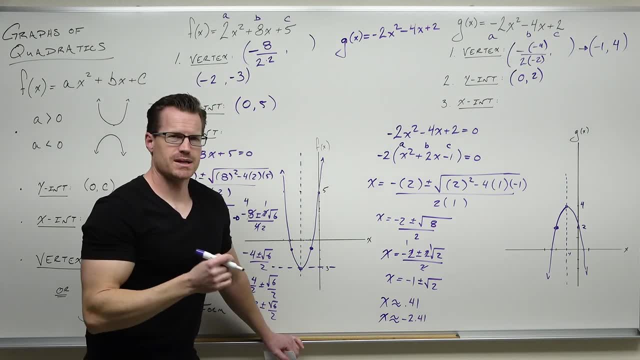 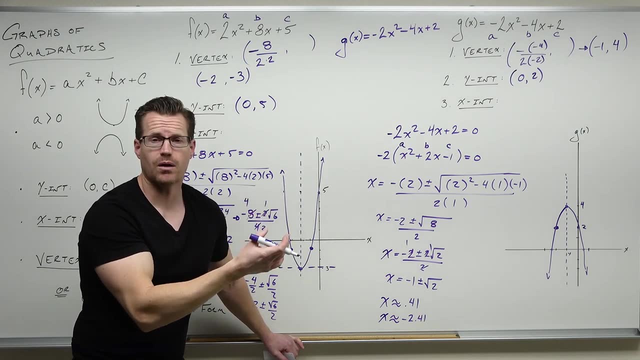 and so that's why I showed you how to complete the square the way that I did, Because if you don't have that other side, you can't compensate for what you're adding for or subtracting on another side of the equation. There's not one. You have to do it on the same side. 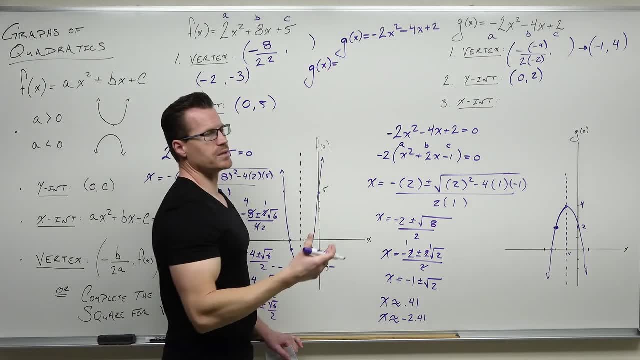 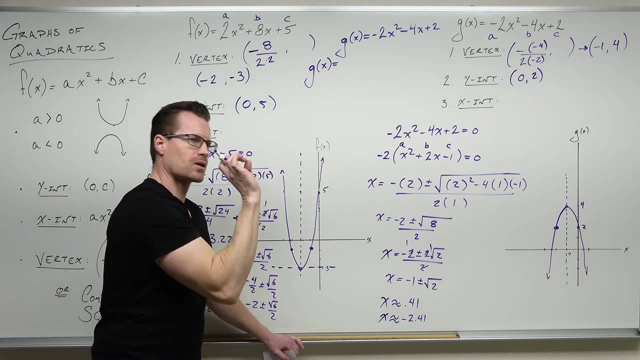 So, rather than teach two different ways, I choose to teach it the way that I do. That way, you have one way that works all the time. What we have to do here is separate our first two terms and our constant at the very far back. 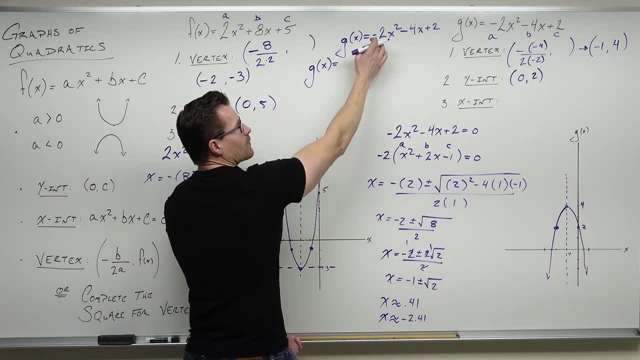 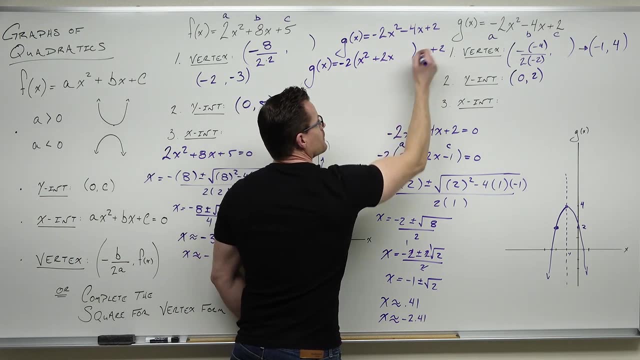 We don't want to lose it, but we want to ignore it for a second And we're going to divide out or factor out a negative two. It's going to change your signs. We're going to complete this so that it's factorable. 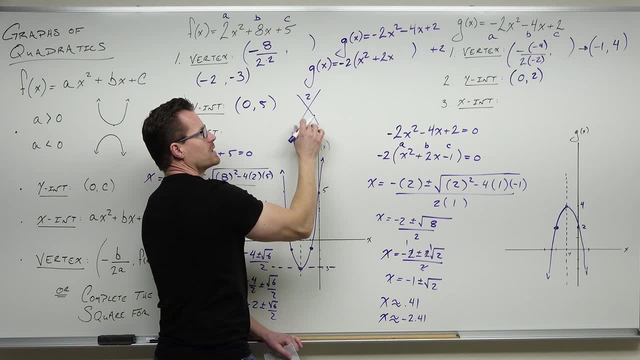 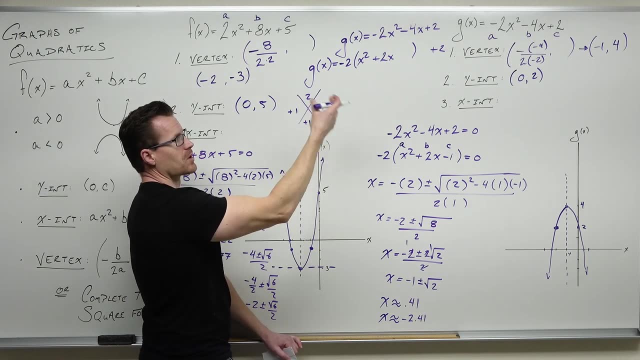 We're missing a number right now. Just think about what you would have to put here to make the factoring actually work. It's got to be a factor, It's got to be a one, So I want this to work as far as being a perfect square trinomial. 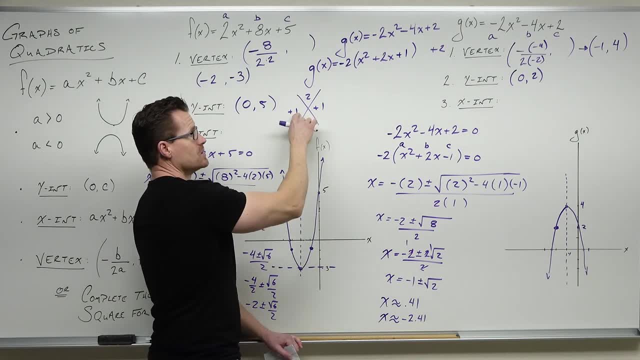 It would be missing a one. It would make that happen. I'm thinking, hey, I got to add a two. What numbers add a two that are the same One? What does this have to be for those to multiply to it? 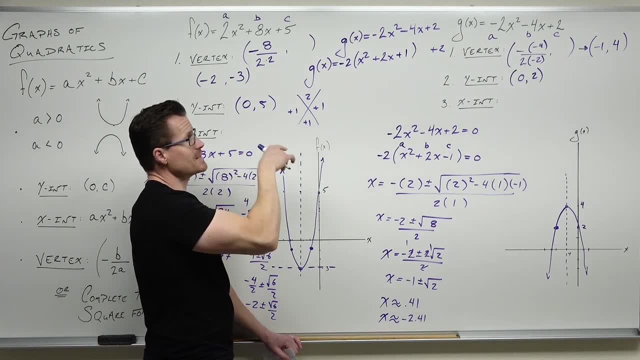 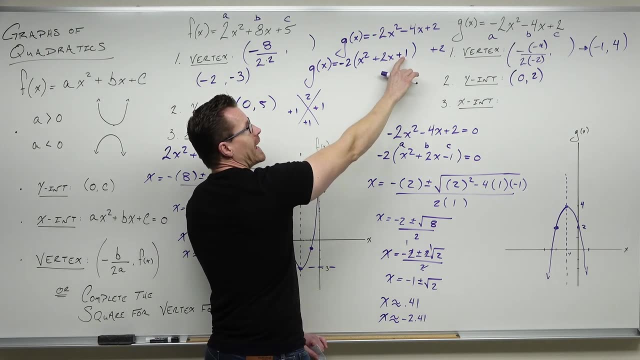 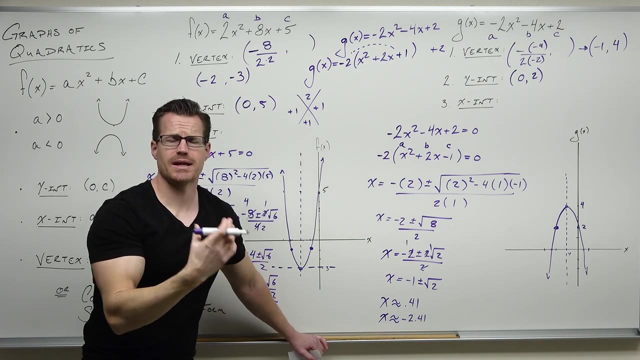 It would have to be one. That's the value I'm missing. The problem is this: By adding that one, you are Distribute this. by adding that one inside of something that has a factor in front of it, You're technically subtracting two. 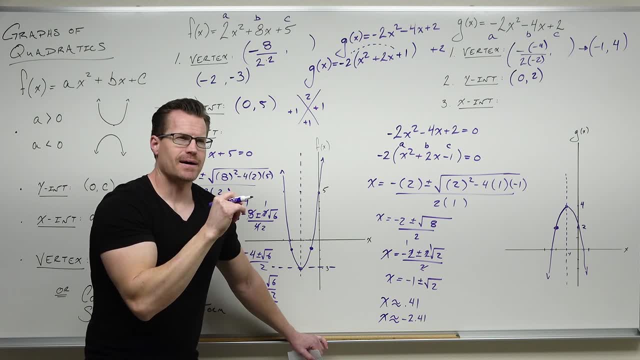 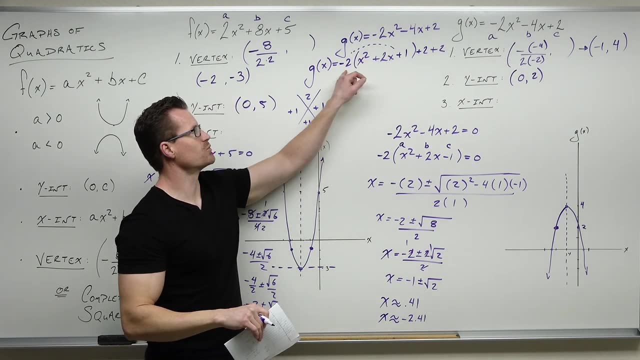 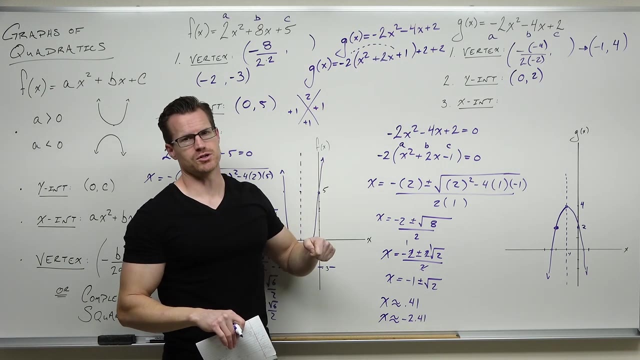 Negative two times. one is negative two. You actually subtracted two from the value of this function. You're going to undo that So, because you added one inside of a parentheses which has this factor in front of it. if you add one here and distribute that two, what you really did is you subtracted two from that function. 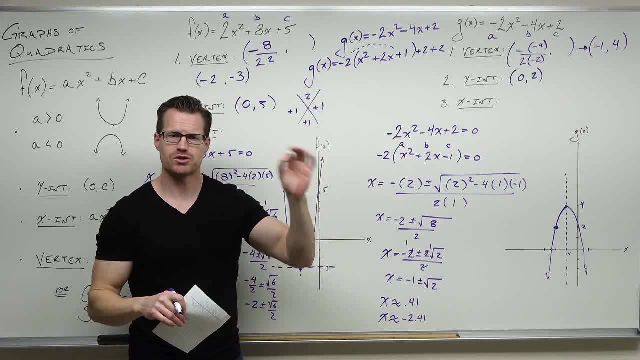 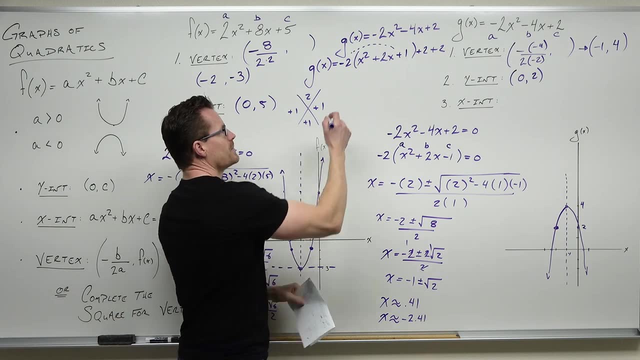 You've got to add two to undo that. So what I tell students is: distribute and then undo whatever that distribution tells you. So this distribution says negative two. We want to add two, We want to undo that. That means that our function is. 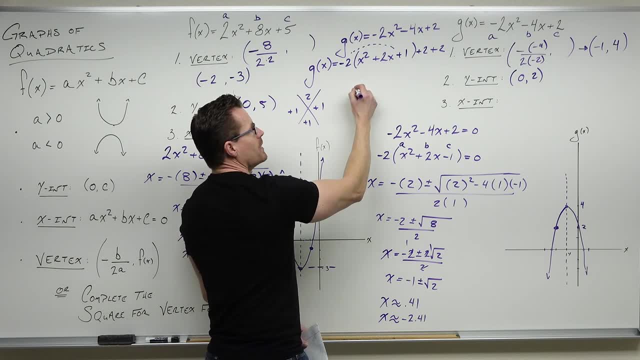 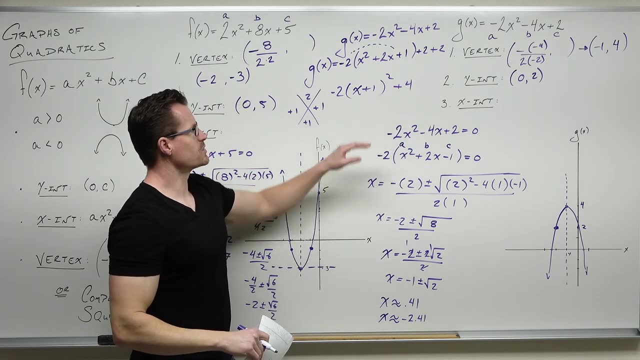 we know that that's going to factor. It's right here. You complete this so that it would factor As x plus one squared. we've got this negative two and then we have this plus four. This says your parabola should be shifted up four. 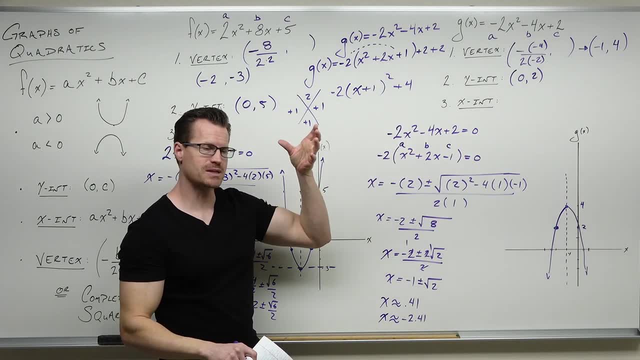 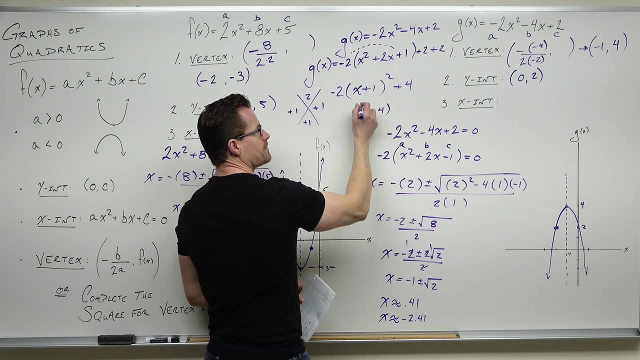 One, two, three, four Should be shifted left one, Remember inside, plus means left, That's where a vertex is. That's why this is called vertex form, because you can easily find your vertex by thinking about the shifting. 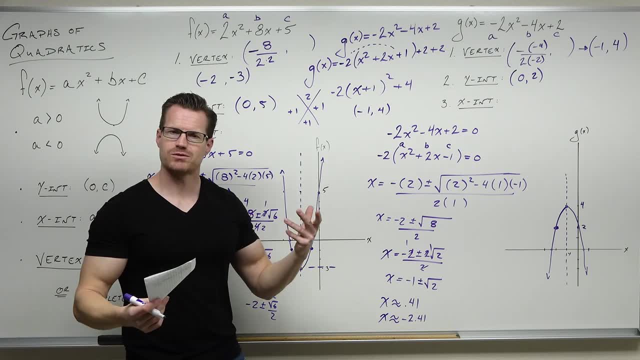 Up: four that's a y value, Left one that's an x value. That's why it's called vertex form. We know it's a parabola. We know it's a downward opening. We could have used key points. 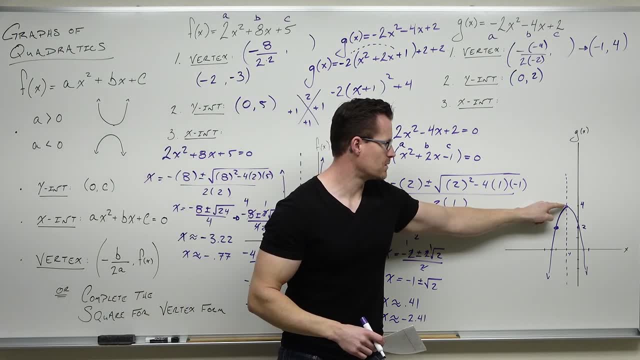 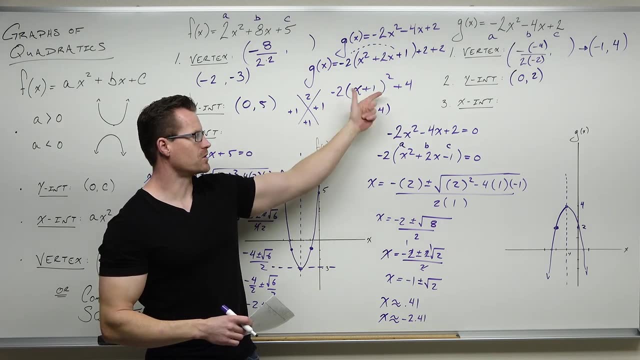 This would be one comma negative two from here. One negative two and one negative one negative two. We get the exact same points as we got before. The drawback is this is a little harder to find x intercepts from. You have to set it equal to zero. 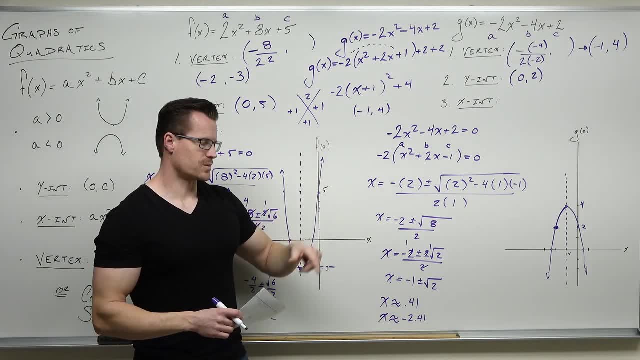 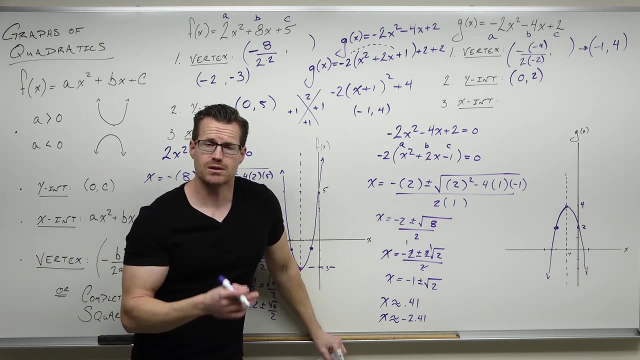 subtract four, divide by negative two, take the square root and then subtract one, You get the same thing. That's the idea behind going through this one of those two ways, Either refining vertex, then y intercept, then x intercepts if necessary. 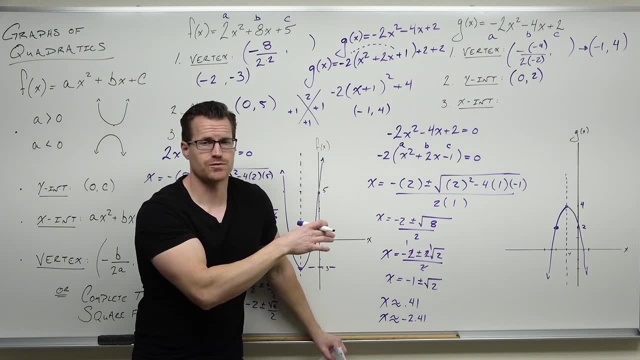 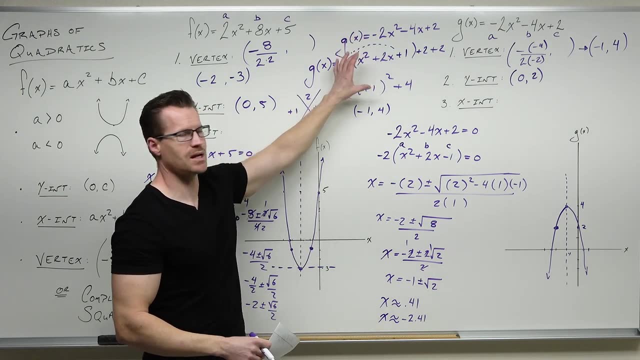 or we're finding the complete the square process with vertex form, Kind of doing the same idea. I hope I've made this make sense. I hope that you see this completing the square as something that's not super duper scary, but something that is giving you the same stuff as this. 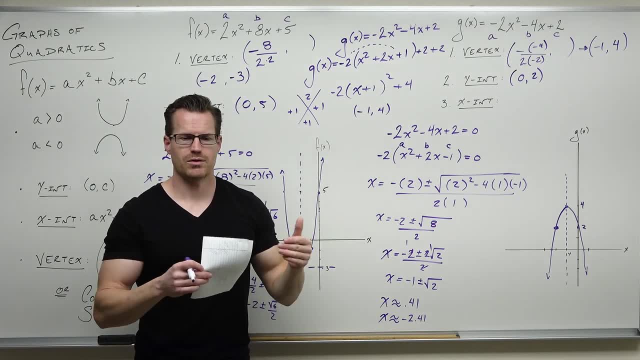 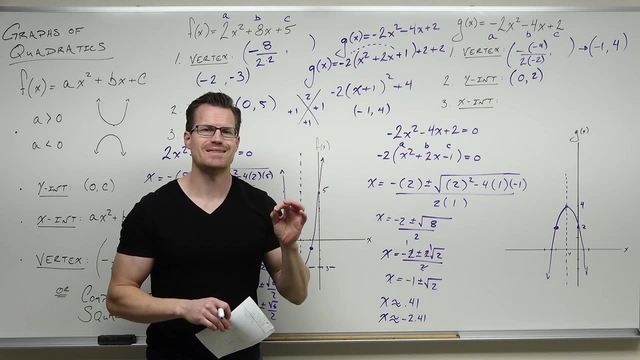 You see, one of the problems in teaching is that we think these are all the same, but we don't know. They're all like, not meshed together. I need you to understand that, whether you're doing this or this, you're finding the same thing. 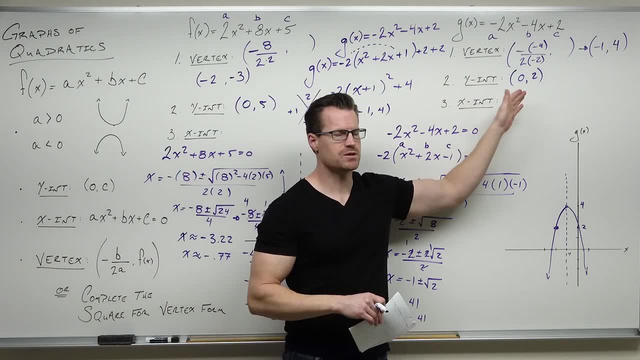 Completing the square gives you the vertex Vertex formula gives you the vertex Y intercept. you can still find it. Plug in zero, you get two. Plug in zero, you get two. Or plug in zero here, you get two. 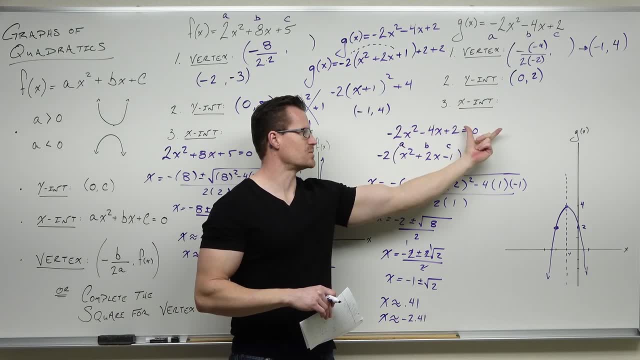 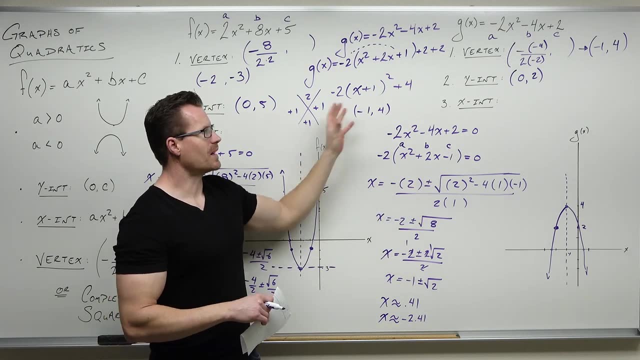 X intercepts. well, I would say that this way is easier, because you have the quadratic formula, or you complete the square, which is where the quadratic formula comes from anyway. So I'm telling you: you're doing the same thing, It's just a different way to get there. 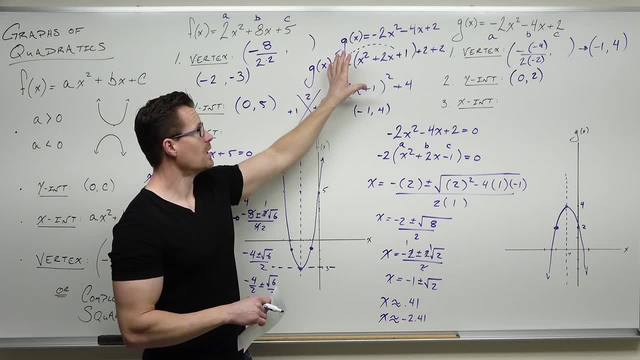 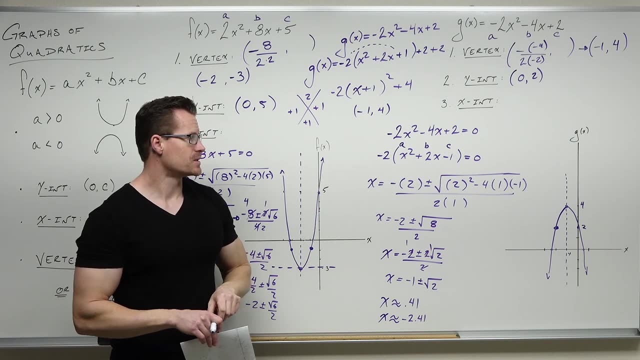 So on the next couple examples, we're not going to go through the whole vertex form. This is only if you need it or if you just really enjoy doing it or want to practice it. So at this point we need to be very comfortable with vertex. 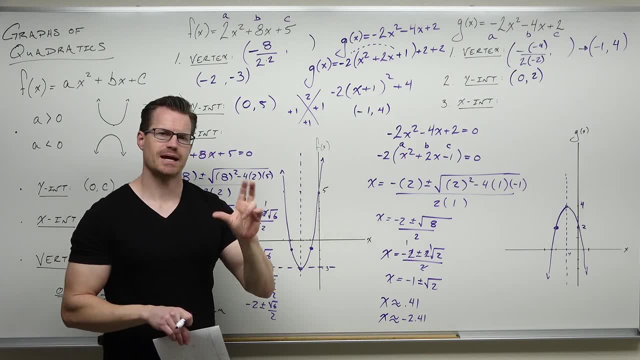 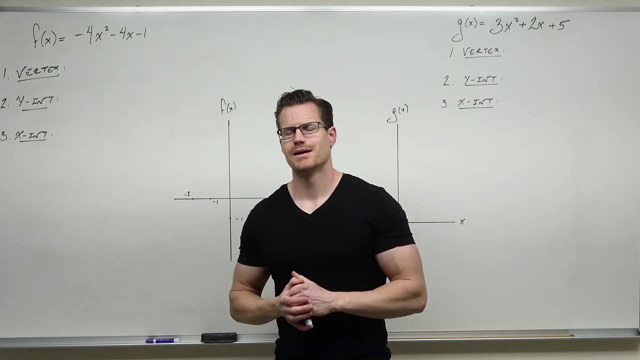 finding that with the y-intercept, using that and then finding x-intercepts of quadratic formula and approximating our calculators. So I'll be right back with a couple more examples. Okay, let's go ahead and finish up our last two examples of graphs. 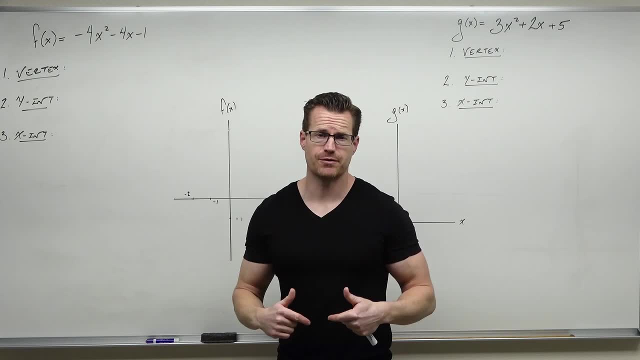 And just to make sure that we understand the process, that we don't always have to find x-intercepts, then I'll show you one way to go backwards. I'll give you a vertex and a y-intercept and show you how to get a function like that from it. 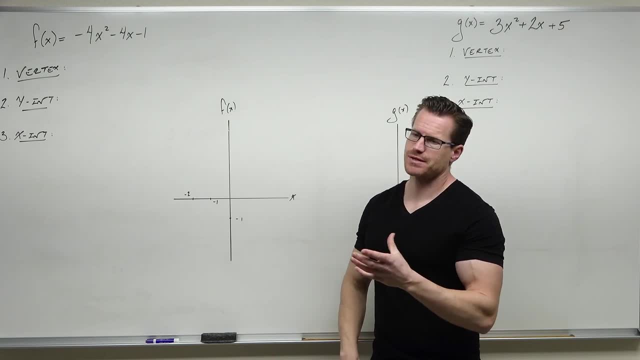 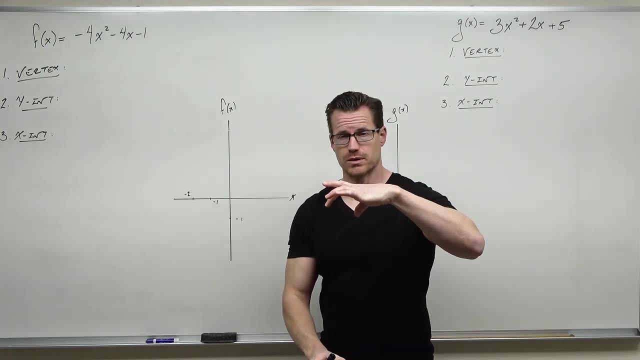 So number one f of x negative 4x squared minus 4x minus 1.. We should all know at this point that that's a parabola and that that is a downward opening and really narrow parabola really. 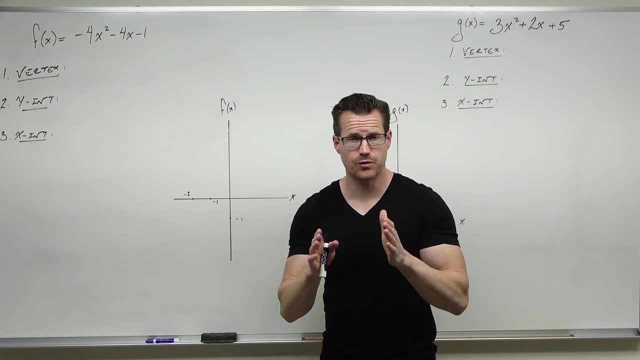 because that negative 4 is going to stretch this thing out. Absolute value of negative 4 is 4.. That's a bigger 1. It's going to be very narrow. Also, what we have is this negative which says that it's downward opening. 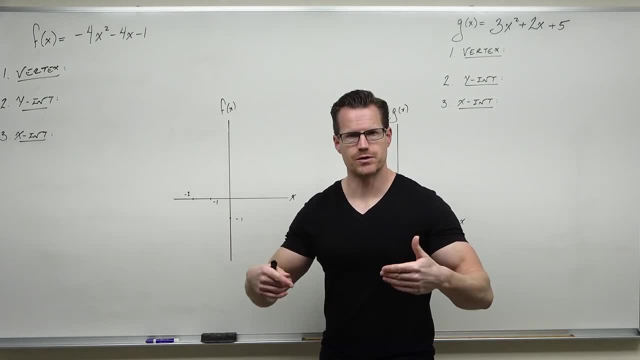 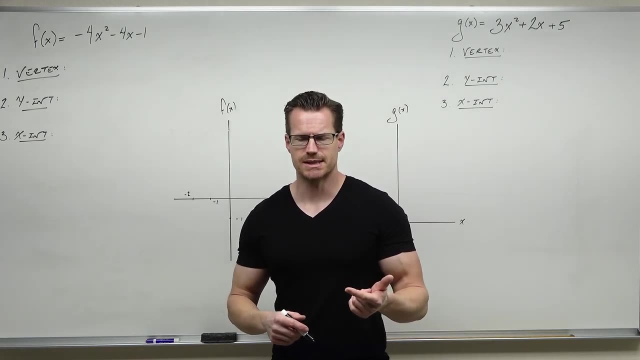 Now we're going to go through. We're not going to complete the square, We're going to do this: the vertex, y-intercept and then maybe x-intercept way, if we can. So with our vertex, we've got to be really good at identifying a, b and c. 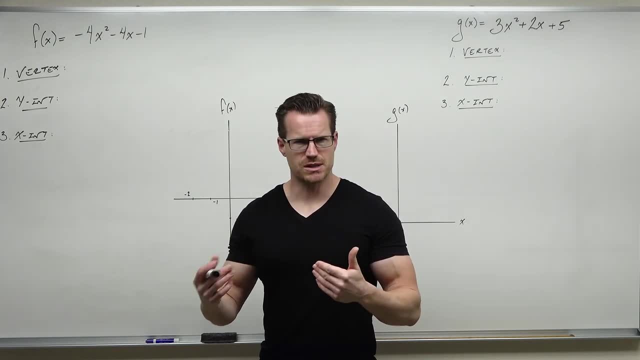 And also I want to make sure that you understand this. You've seen me change some signs from time to time. That only works when you have this set equal to 0 to find x-intercepts. We can't go and change signs now before finding the vertex and y-intercept. 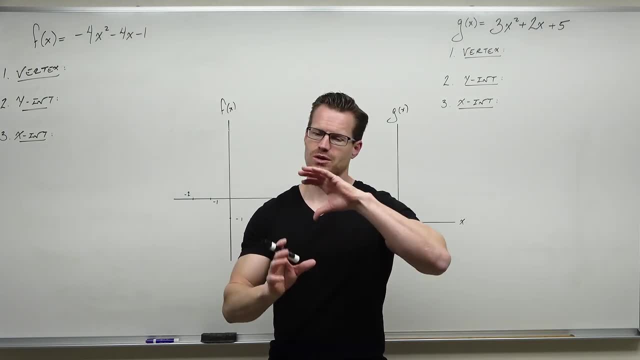 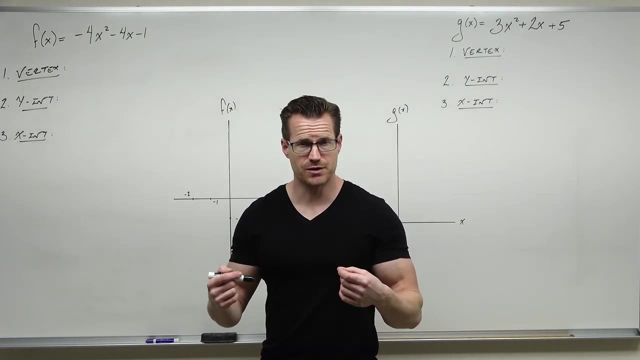 That's why we do the x-intercepts last, Otherwise we start making these signs change and then we have a different opening parabola. That's not OK. The only reason why we can change signs for x-intercepts is if you reflect a function. 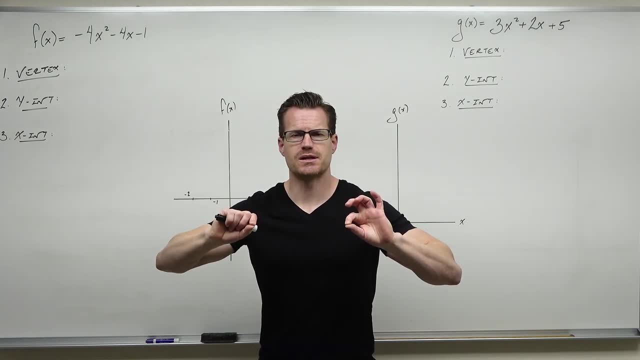 about the x-axis, change the signs. the x-intercepts themselves don't change because they're on the thing that you're reflecting about. They can't change signs because they're signless. That will put a 0 for those x-intercepts. 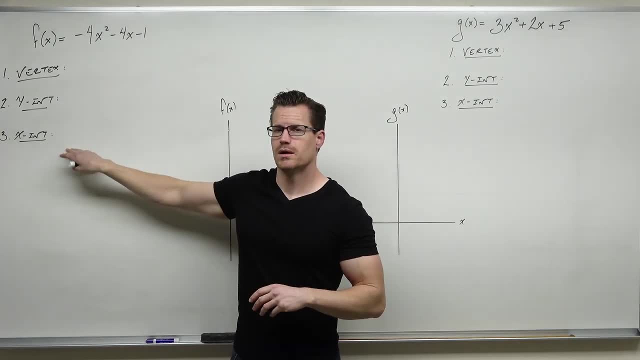 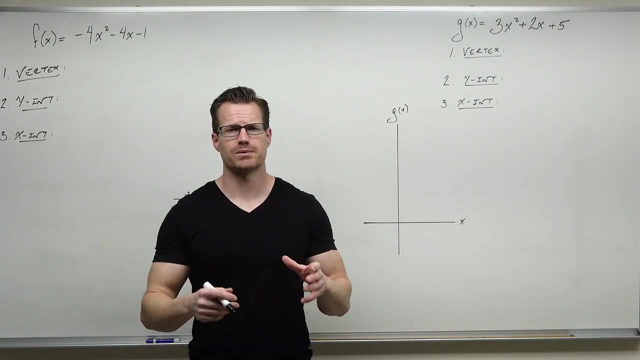 So we don't change signs until we get to here. So for our vertex we all write: our a has to be negative 4, our b is negative 4, and our c is negative 1.. That's the numbers that we got to use to find the vertex. 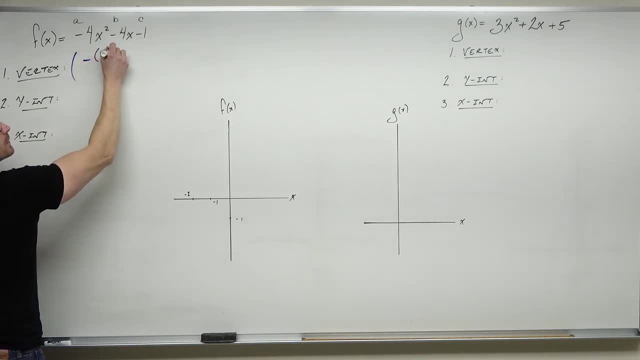 So we're going to do negative, negative 4, 2 times negative 4.. We're going to leave that open for just a second so that we understand. we're going to evaluate our function for that x-value in order to find our output for our y-value. 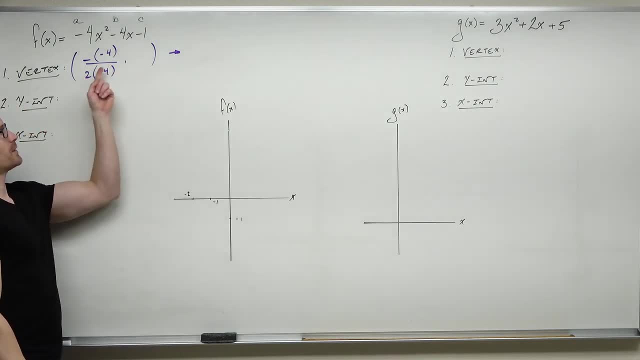 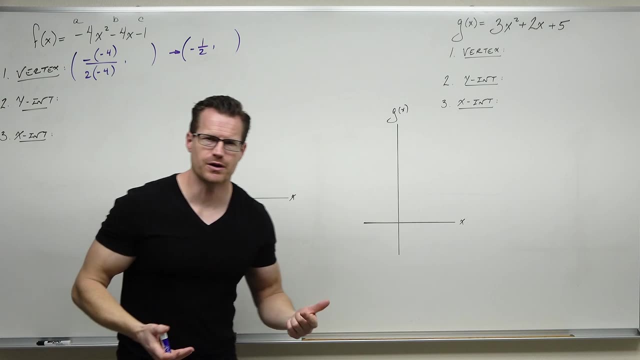 or y-coordinate. So that's positive 4.. That's negative 8. That's negative 1 half, which gets kind of awkward when you start evaluating functions for fractions. I'd recommend your calculator Just take it, Use your fraction button. 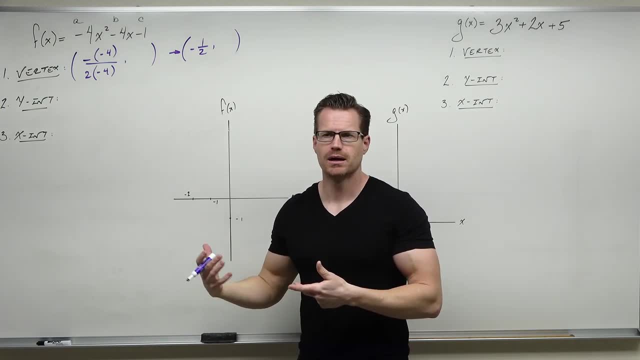 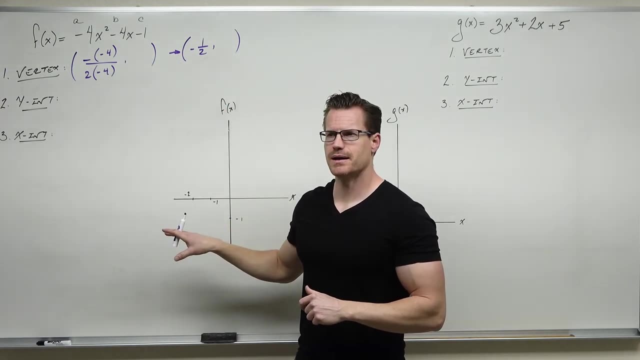 It's helping. we don't make a simple error. You probably can do that in your head, but double-check your work, at least with a calculator, because it's really awkward to put that vertex down here and then use a Wiener step. that's correct. 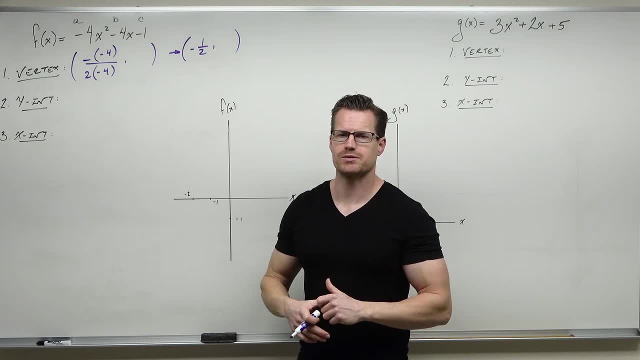 With a vertex. that's not. it's not going to look very good for you, You're not going to get a nice parabola. So with negative 1, half negative 1, half squared is positive 1, fourth times negative, 4.. 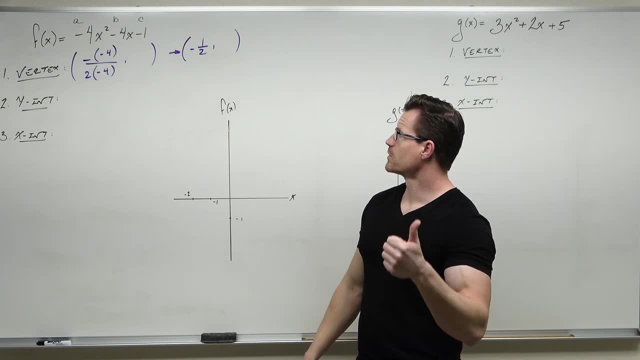 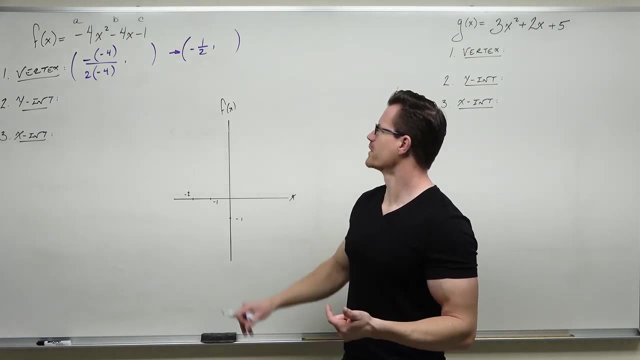 Well, that's negative 1.. And then we have this negative 4 times negative 1 half. Well, that's positive 2.. So negative 1 plus 2 minus 1 is 0. What would 0?? Well, that's weird. 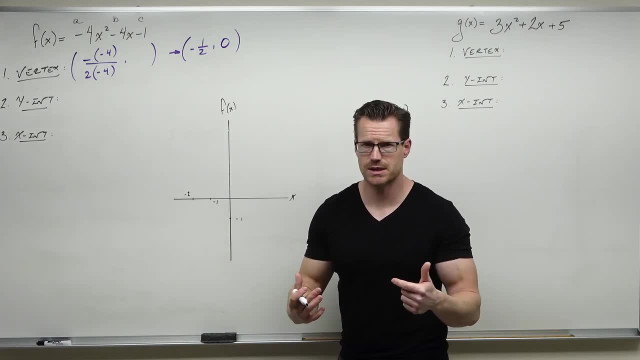 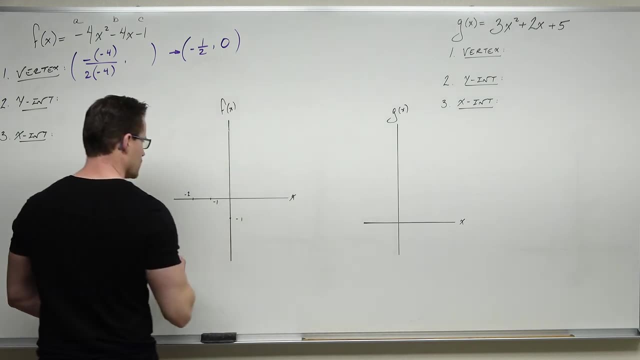 What in the world does that mean? Well, we know that's a vertex and every parabola's got a vertex. Let's plot the vertex. Remember it's a vertex at negative 1 half 0.. Negative 1 half 0 is right there. 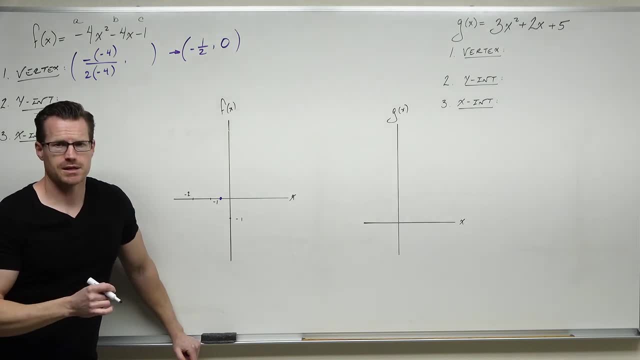 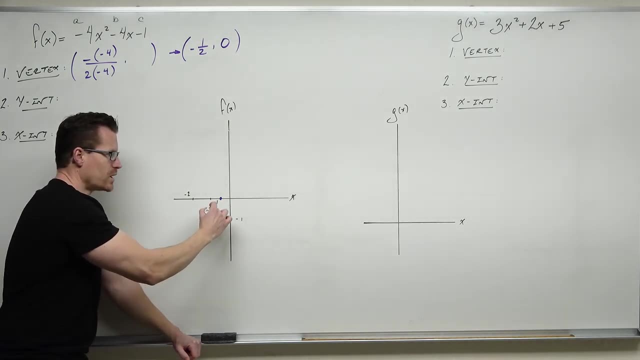 That's negative 1 half comma 0.. Now think about this. This is the vertex, which means it's the highest point of a downward opening parabola. If this is the highest point, can this parabola ever cross the x-axis again? 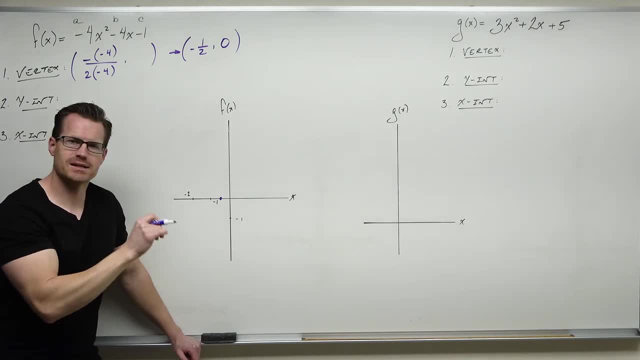 No, it can't. We know this because if you have a vertex that's sitting on that x-axis, you have 5.5.. You have 5.5.. So you have to find the x-intercept. If we had found the only x-intercept, it's a double root. 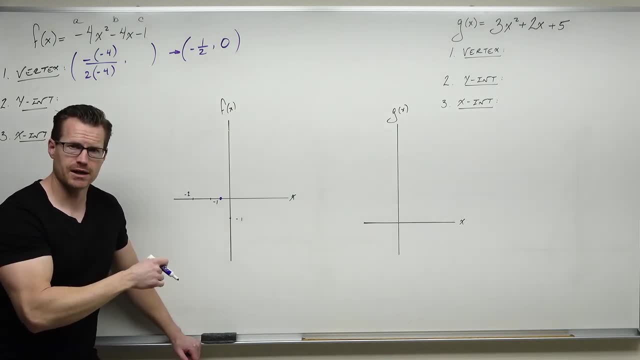 And if we had gone down to x-intercepts and solved this equal to 0, we're going to find negative 1 half twice. If you want to try it, try it, Try factoring it, Try doing whatever you want. It's going to work. 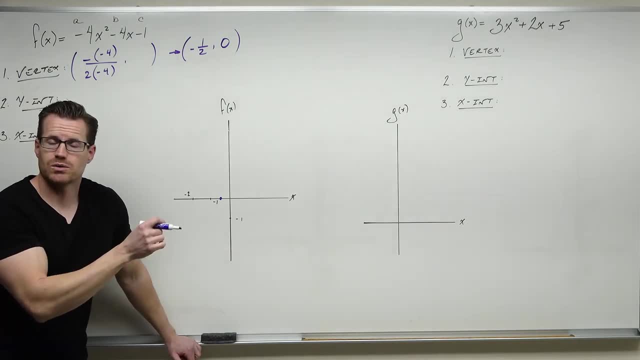 It's going to factor, But you'd get a protein in a minute if you really want. So that right there, that vertex that says you don't have to do x-intercepts right now, You found the only x-intercept that you're ever going to have for this function. 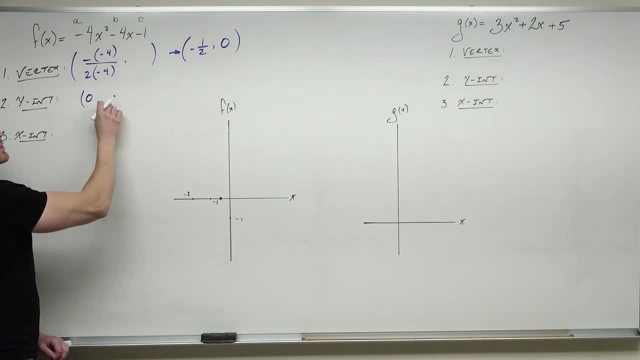 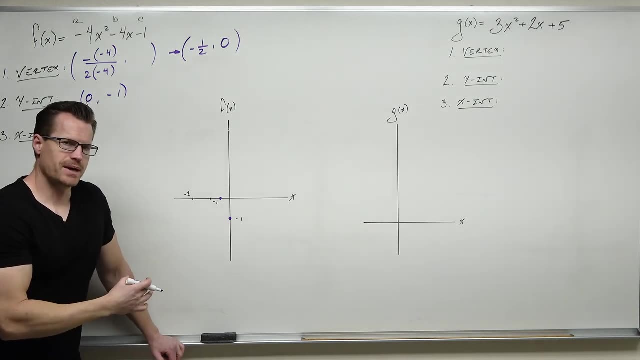 What you do have to do is find your y-intercept 0, we're going to get negative 1.. I know that 0, negative 1 is our y-intercept. Notice how narrow that makes it. If that's our vertex and that's our next point, that's a really, really narrow. 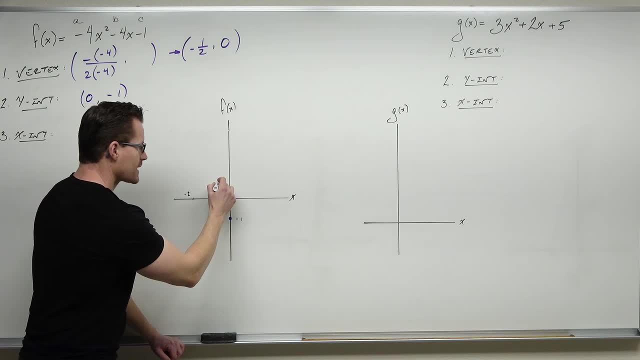 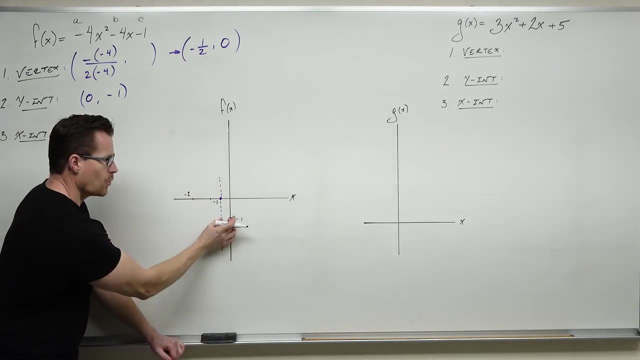 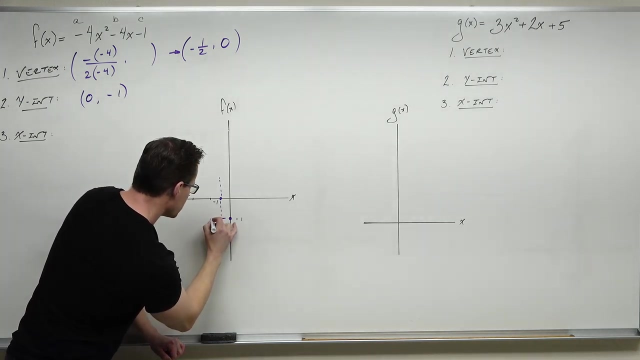 parabola. Now what do we do with it? Well, we know that the axis of symmetry goes right through the vertex. So if I'm a one-half unit away from my axis of symmetry here, I can go one-half unit on the other side and find a symmetrical point. This is what we would. 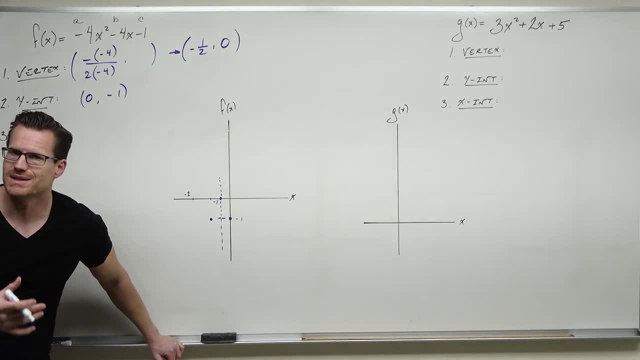 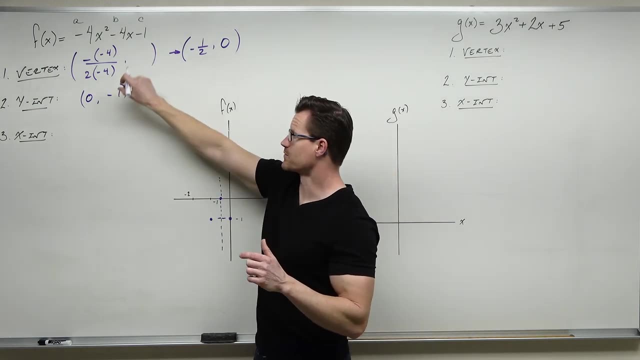 use to graph our parabola. Now, do we have to continue? Do you have to find the x-intercepts? No, it's irrelevant, You've already found it. So that's what we do. is in order. Every parabola has. 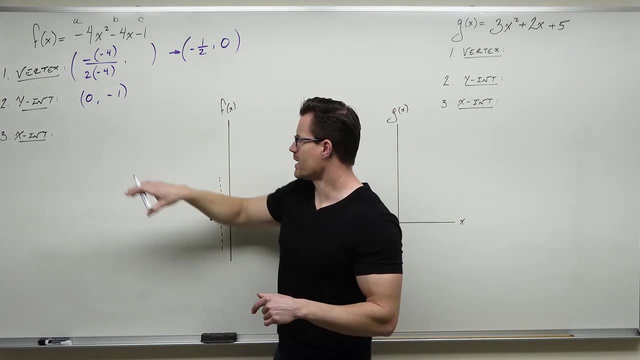 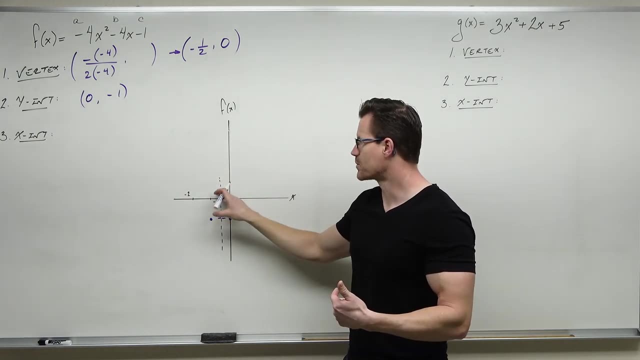 a vertex. Sometimes you're going to find the x-intercept here. Every parabola is going to y-intercept. Use it to find a symmetrical point. But if we understand what this looks like a downward opening parabola, it matches. 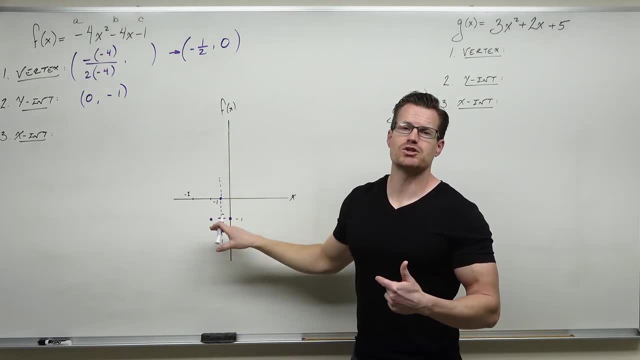 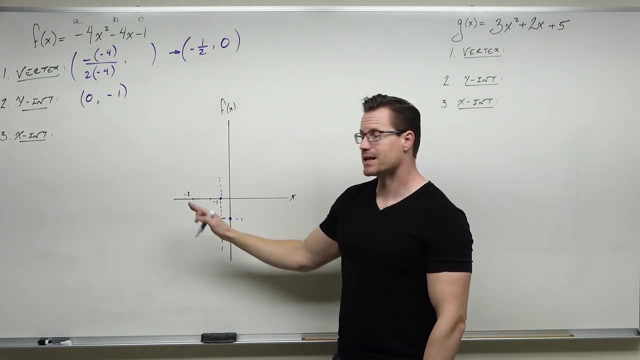 It's narrow, It's downward opening. There's not going to be any additional x-intercepts. Don't waste your time. The only thing that might make this a little better is to go one more unit outside of what you have. What I mean by that is you might want to plug in a value like negative 2. 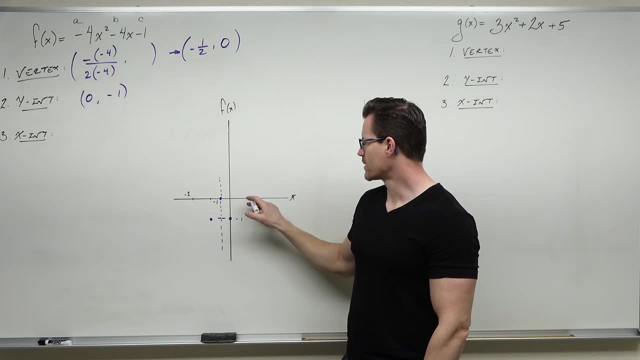 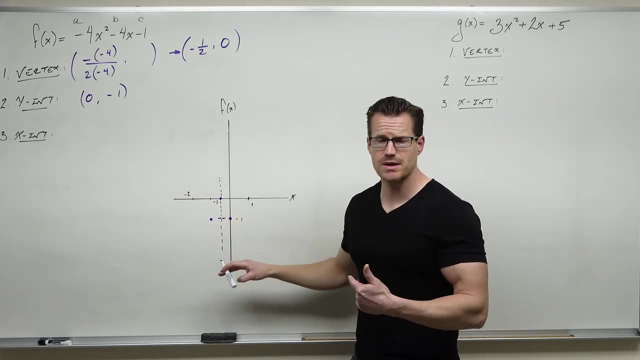 or here's 0, plug in a value like 1.. If I plugged in 1 and I plugged in negative 2, I'd have two additional points that would be symmetrical. Or plug in 1 and use symmetry. That's fine too. 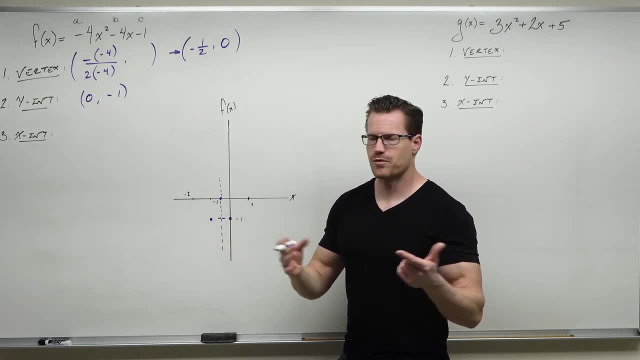 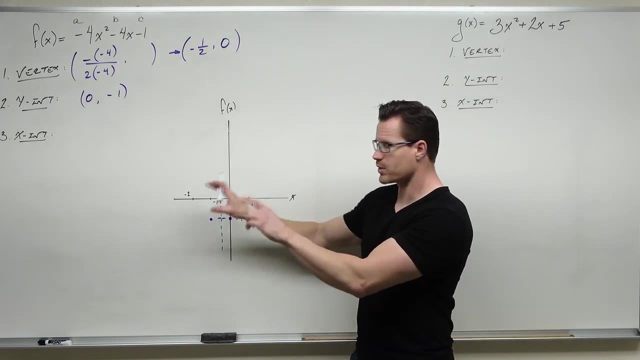 That would give me a better shape of this thing. So I hope that makes sense to you. For me, I mean, this is clear enough that we know that's pretty narrow, but you might want to go ahead and plug in two more points here, or one more point, and use symmetry. 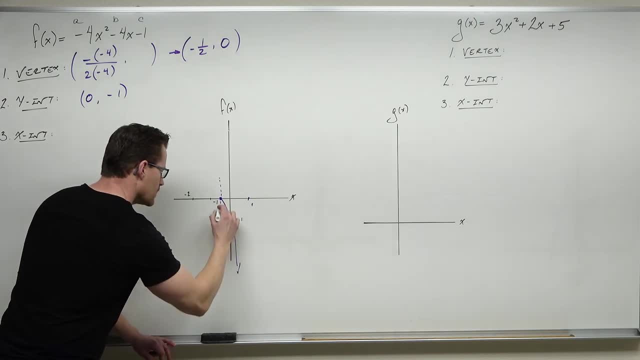 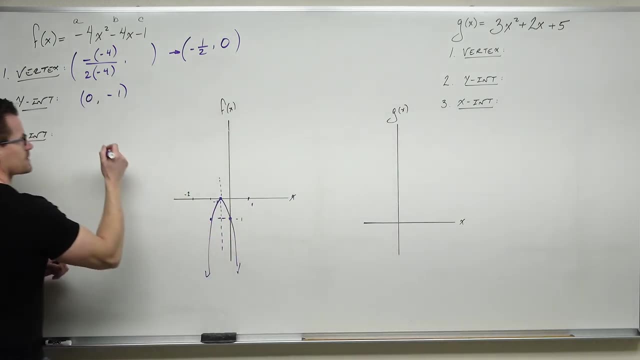 So we're going to do this. Get as good of a parabola as we can out of it. and if you want to see the x-intercepts, if you plug this and our set is equal to 0, and you change. 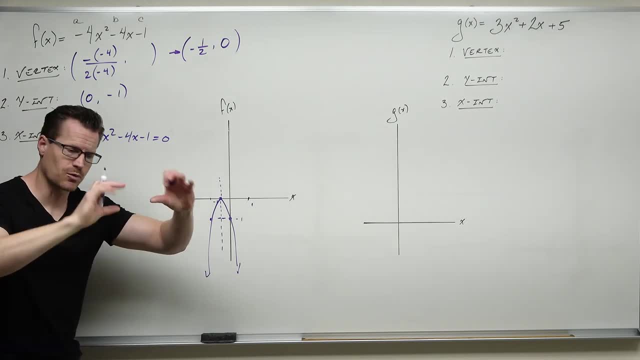 all your signs, Because we can now, because equal to zero doesn't really matter. We're talking about x-intercepts. If you reflect x-intercepts, they don't do anything. They stay the same. We get positive 4x squared. 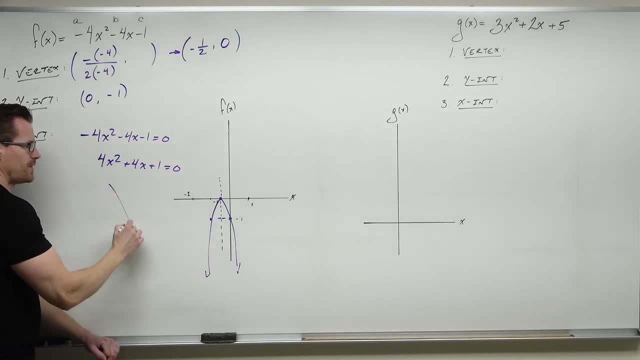 plus 4x plus 1.. This factors actually, but you divide by your a and you'd say, oh, my x-intercepts are. remember this: change your sign: negative 1 half and negative 1 half, You have an x-intercept. 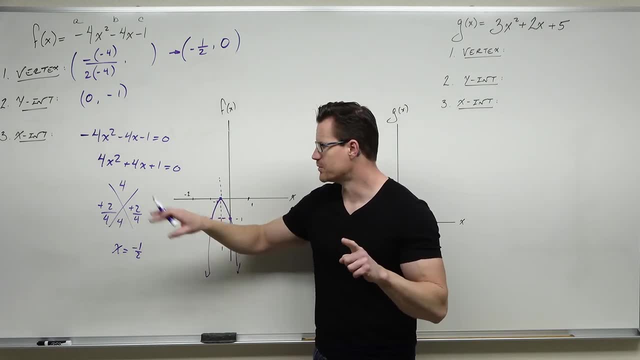 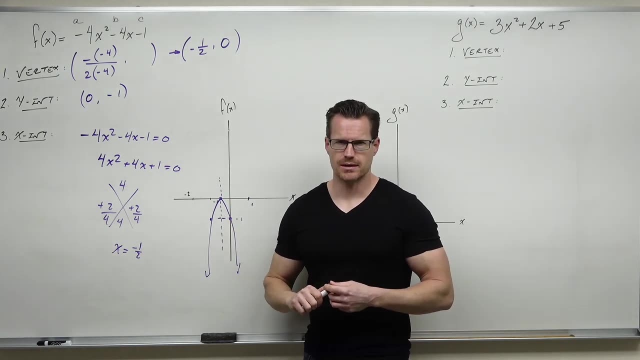 at negative 1 half. That's exactly what we found. and there's only one. It's a repeated root. It's a double root: multiplicity 2.. It says your function is bouncing off the x-axis. That is what I want you to understand. I hope I've explained it well enough that you do understand. 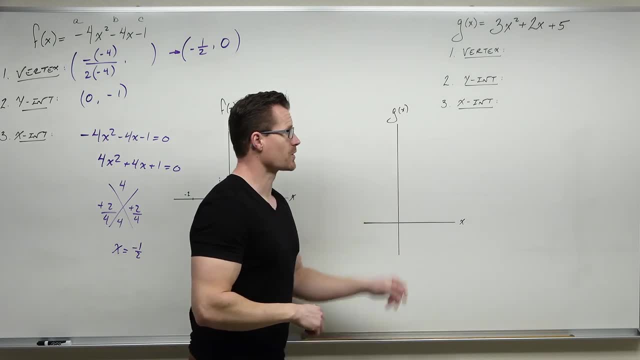 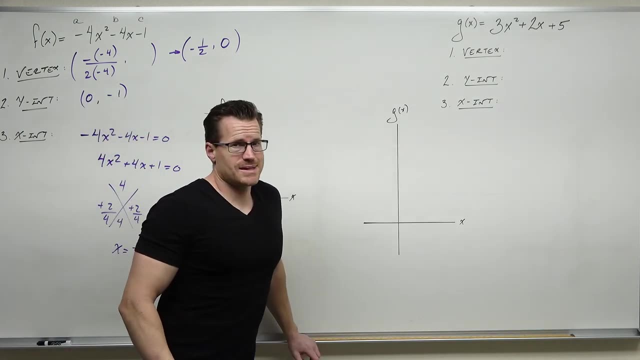 that We're going to go on to the last example. As far as graphing is concerned, it's going to be very quick, and then we'll talk about what I told you going backwards. All right, so let's take a look at g of x. We have 3x squared plus 2x plus 5 in your head right now. I need you to be thinking. 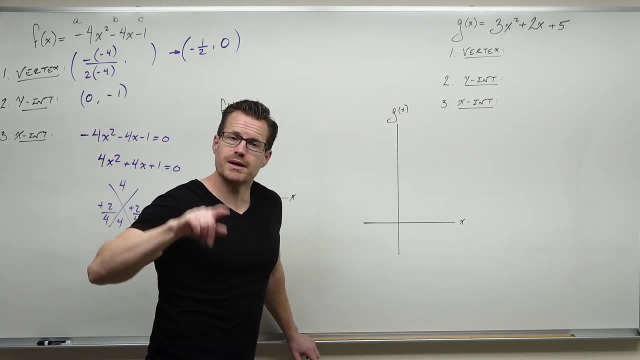 that's a parabola. I need you to understand that it's upward opening, because we have that positive 4x squared plus 2x plus 5 in your head right now. I need you to be thinking: that's a positive 3, and it's fairly narrow, because it's not as narrow as this one was, but it's a little. 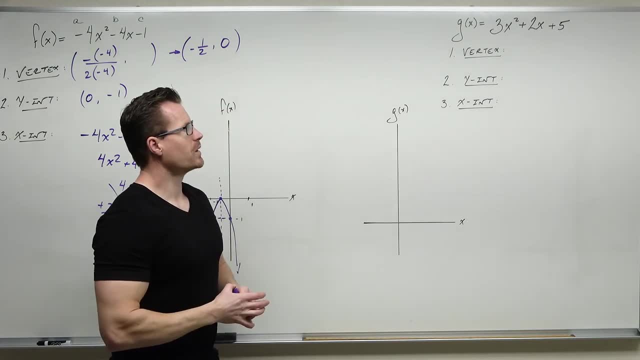 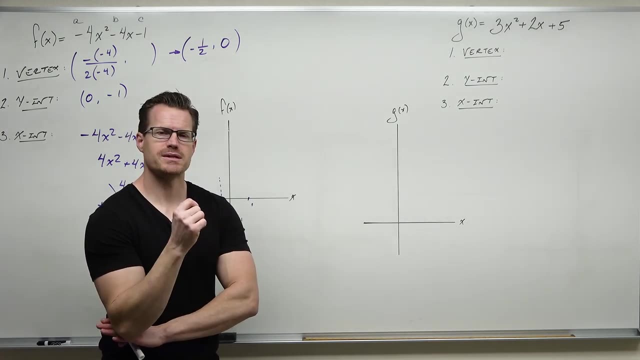 bit more narrow than the 2, a little bit less narrow than the 4.. We're going to go ahead and find the two things that this graph is going to have. It's going to have a vertex, because they all do. It's going to have a y-intercept, because they all do, but this is not going to have any. 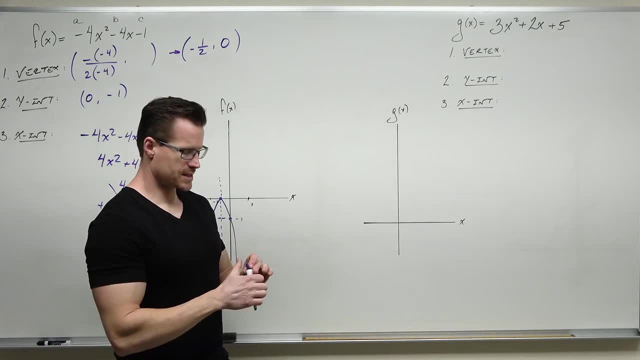 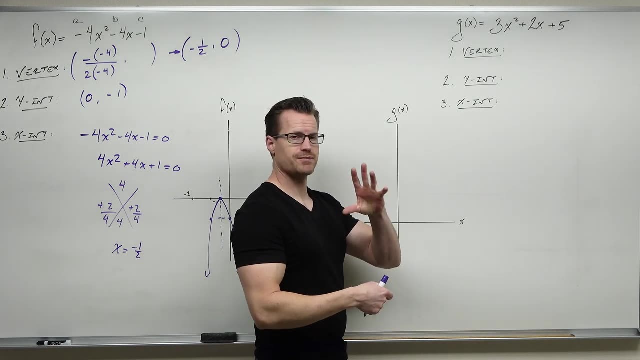 x-intercepts. I want to show you how to deal with it. So, for our vertex, if we identify our a, which you should Maybe try it right now- Our a is 3, and our b is 2, and our c is 5.. 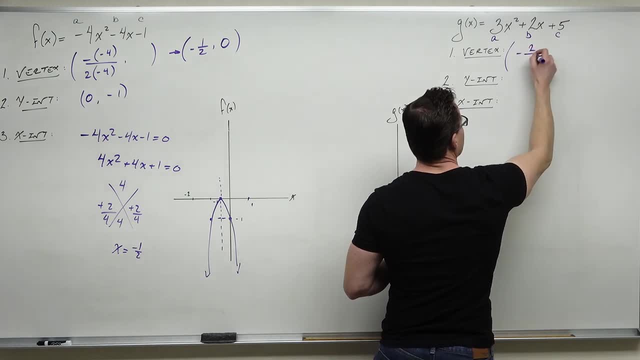 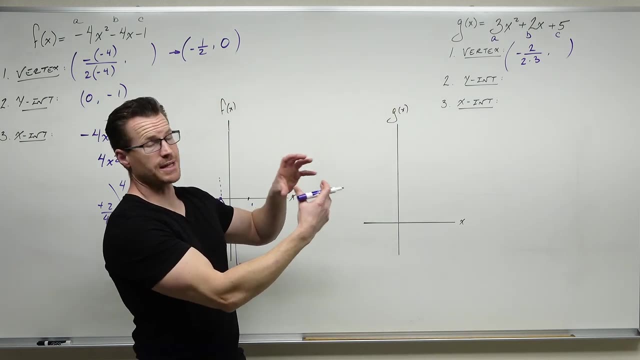 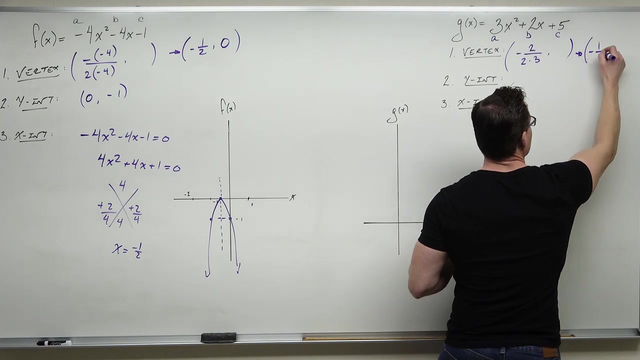 So we put negative b, that's negative 2, all over 2 times a, that's 2 times 3.. That gives us negative 1, third, which is kind of awkward. Now, if we evaluate that, that's the only way we find. 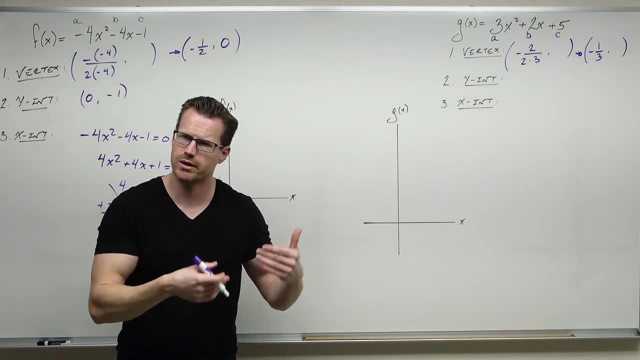 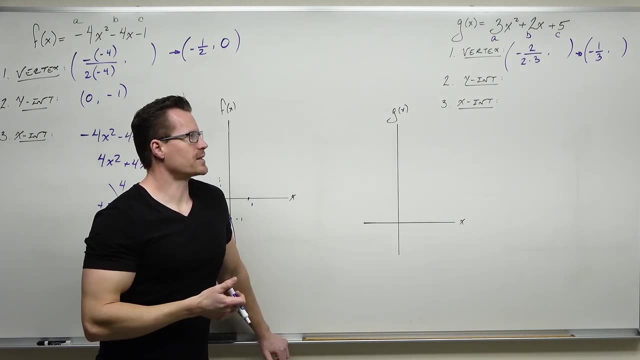 points in functions is to evaluate them or understand the function which we're learning about right now. So if we evaluate for negative 1 third, we're going to have a negative 1 third squared Man. negative 1 third squared, that's 1 ninth and then a third of that, or 3 times that. 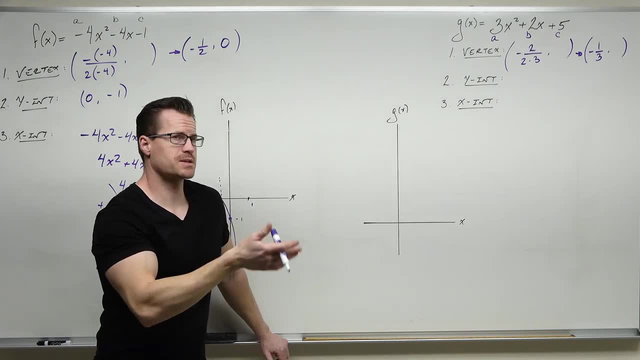 is 1 third again. Okay, well then, 2 times negative. 1 third is negative. 2 thirds: 1 third minus 2 thirds- well, that's negative. 1 third plus 5 is 4 and 2 thirds. And so you do that or you use: 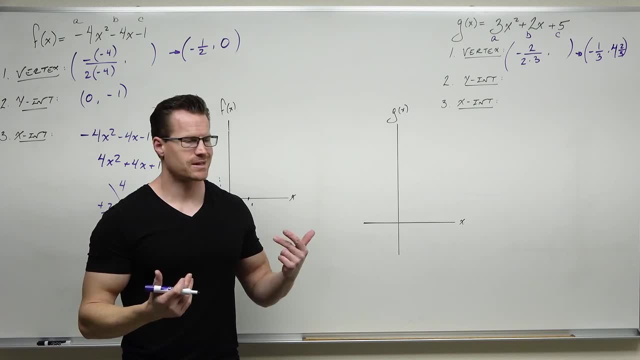 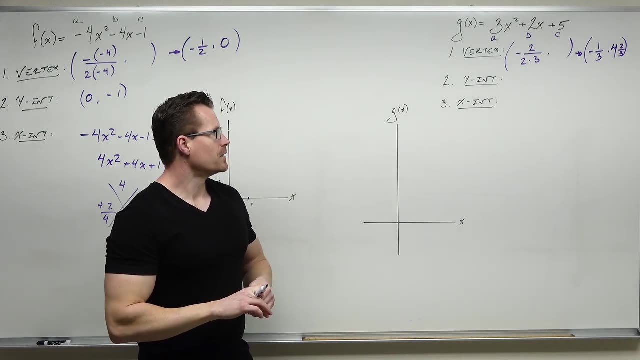 your calculator and you get the same thing. You might get an improper fraction. that's fine too. Let's see: 14 thirds. 14 thirds would be. oh yeah, would be okay. Now can we graph that, Can we plot it? Sure. 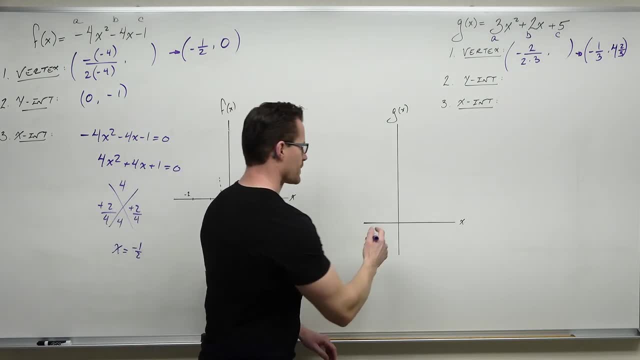 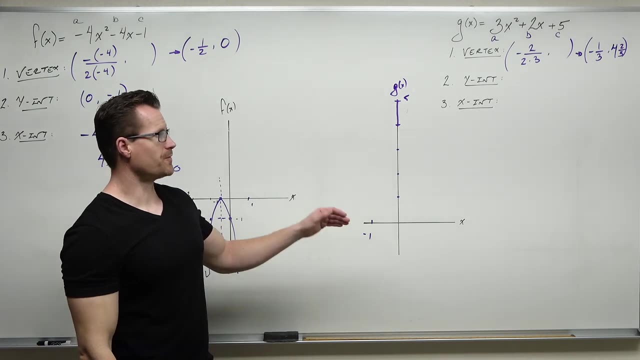 it's a little awkward, but where our vertex occurs is, let's say, this is negative 1, then negative 1. third comma: 4 and 2. thirds 1, 2,, 3, 4, and 2 thirds: negative 1 third. 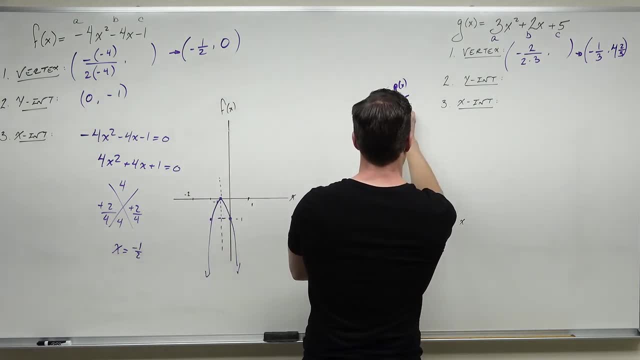 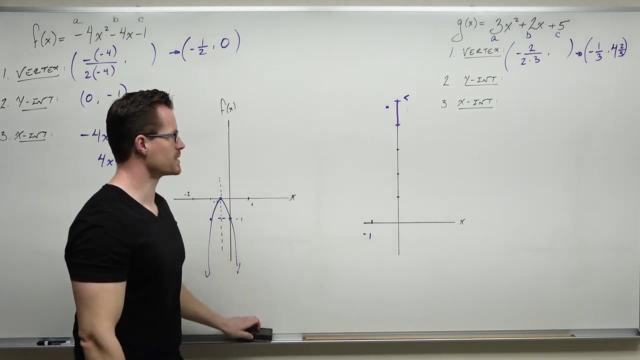 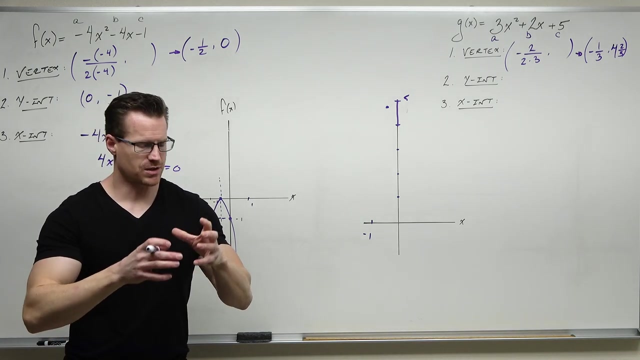 Probably right about there. I'm going to have to adjust my graph a little bit more because of this. Oh, maybe not, It's just going to be kind of awkward. That's where our vertex is Now. think You just you hopefully said in your head that this is upward opening. 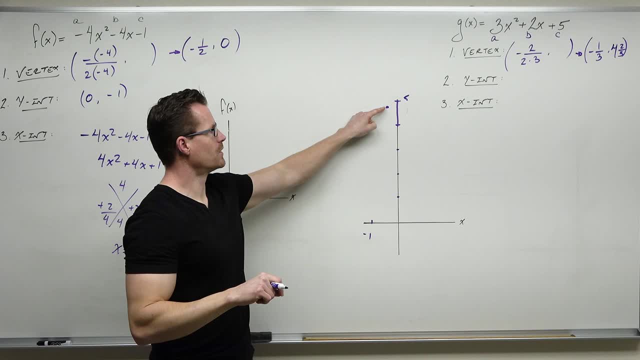 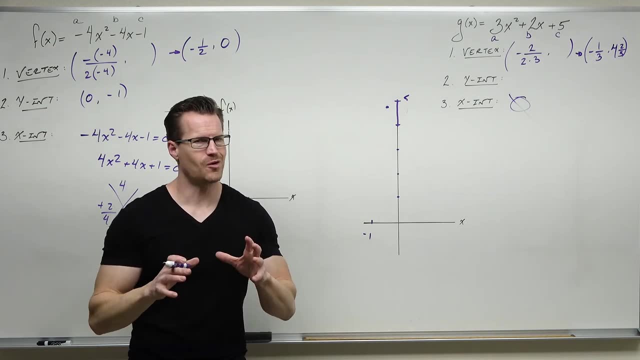 It's upward opening and your vertex is way up here. Is this ever going to cross your x-axis? ever? No, this is there are none. If you want to do quadratic formula, oh man, I hope this makes sense. What's your discriminant going to be? 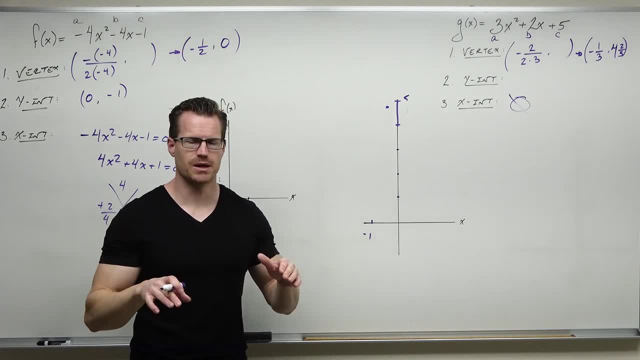 Is it going to be positive, negative or zero? If this doesn't have any x-intercepts, your discriminant would have to be negative. This would give you two complex solutions here, saying you are not crossing the x-axis. That's what's going to happen if you try to find x-intercepts. 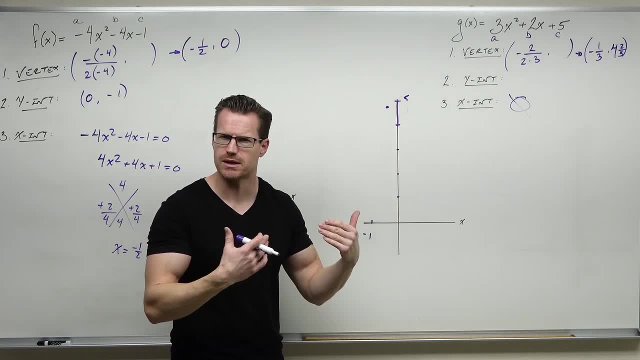 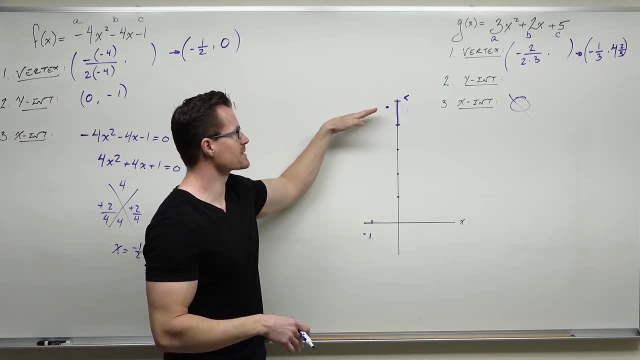 So we're not going to, since we're doing something practical. We're actually graphing this, So we don't, we're not going to have any x-intercepts, We're not going to try to find them because we understand this is upward opening, Vertex is above the x-axis. In fact, our y-intercept- 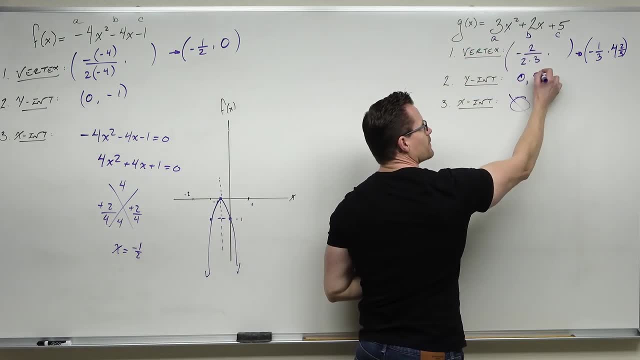 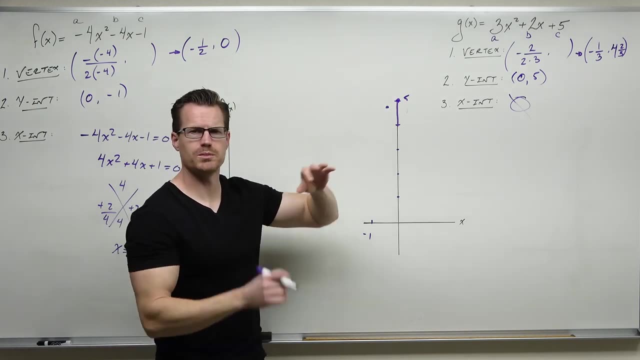 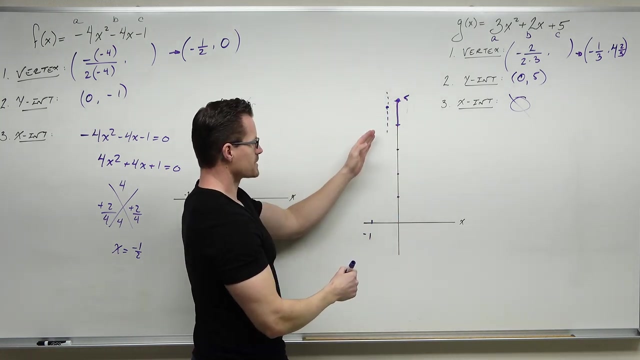 which is zero, zero, zero. comma five is right here. Now this is kind of awkward because we don't have a lot of room to notice the curve of this graph. So if you were used to act as a symmetry, which is fine, this is a third of a unit from remember. this is negative one-third. 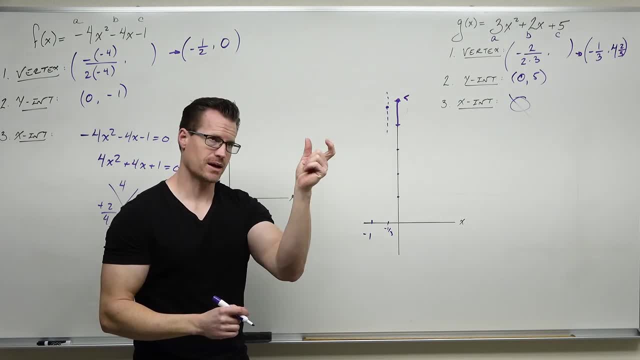 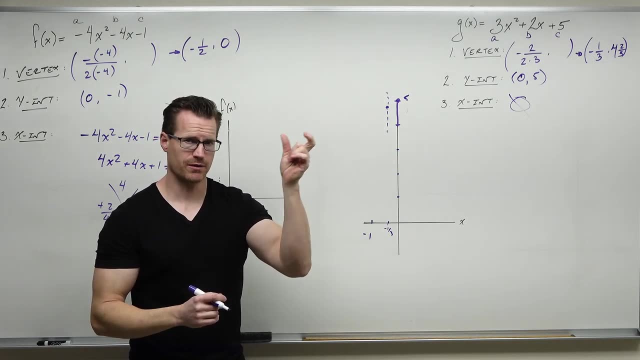 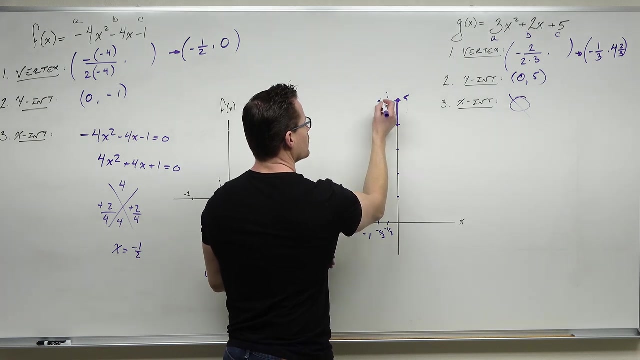 That's a third of a unit away from the y-axis. the y-axis is a third of the way where that that y-intercept is is a third of a unit away from the axis of symmetry. If we go another third of a unit, so like negative two-thirds, we plot another point, Use our symmetry and 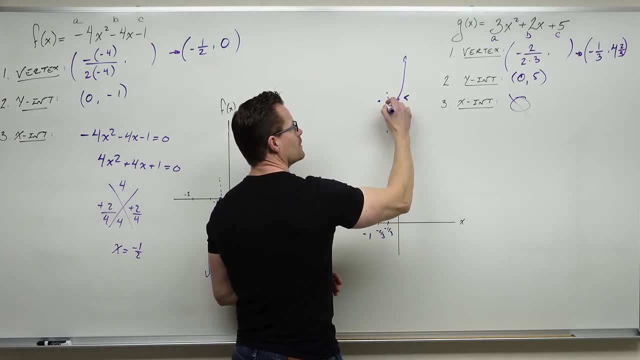 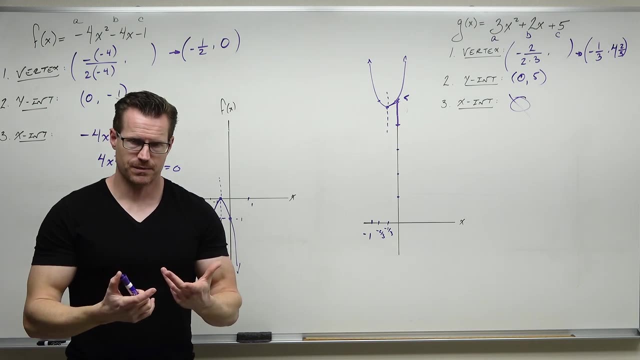 use our knowledge of the fact that this is going to be quite narrow to give ourselves that upward opening problem we know we're going to get. What would make this better is to use some values outside of your y-intercept. So I would use something like: 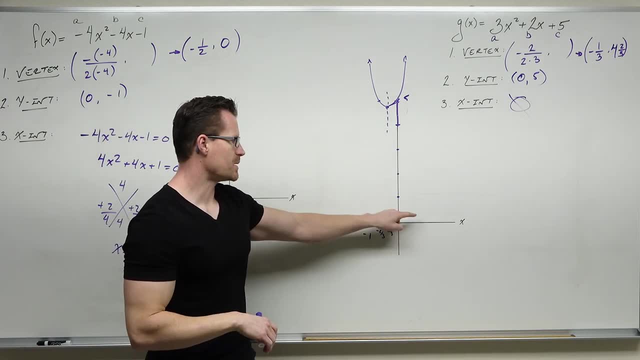 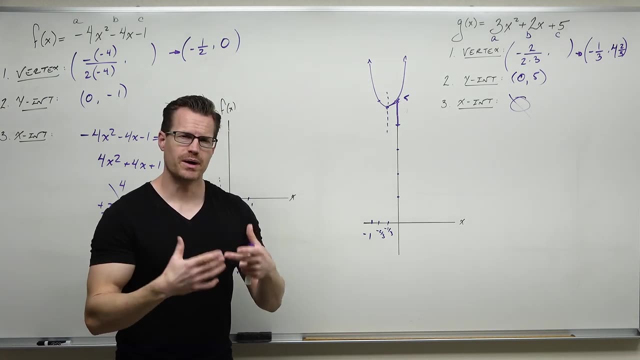 negative one and maybe positive one. They're not going to give you symmetrical points here because they're not spread evenly from that negative two-third, negative one-third. but it would be a little bit better than nothing. So plug in a couple points here to get that that nice. 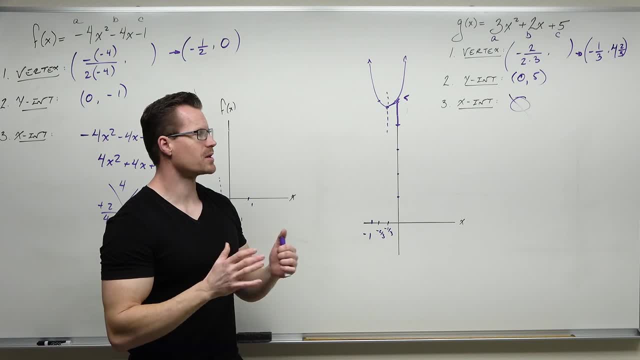 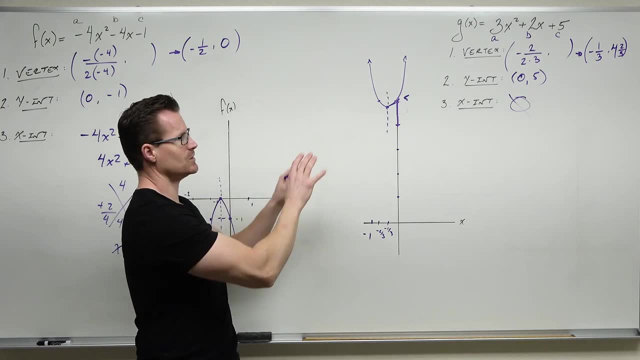 look to your graph. That's where I'm going to leave you. I'm going to leave you just with the understanding of what the vertex does, that you need at first y-intercept second, and then you might not even have to do x-intercepts and how to deal with that. So I hope that that's made sense. 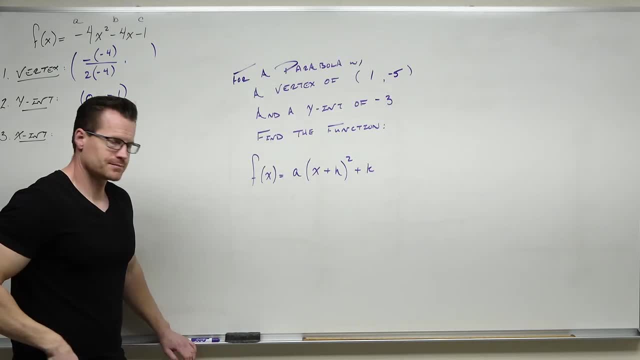 I'll come back with one more very quick example, So I'm going to give you a little bit of time to think about this example. Okay, so sometimes you're asked to find a function given some information, like in this case: you got a vertex and you have a y-intercept and it says: find a. 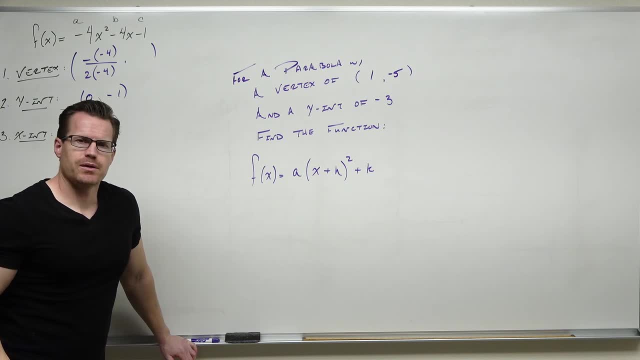 function. How in the world do I do that Really? by understanding how your functions work in what's called vertex form, which I've talked a lot about in this video in the first two examples. So what we're going to do here is two-fold, Because we have one, two, three missing parts, three missing. 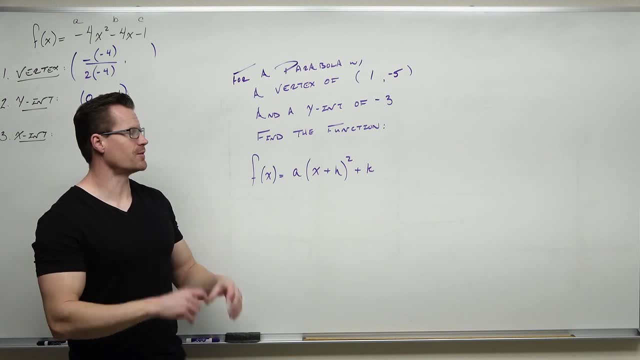 values and one, two, three missing or three given values. we're going to have to find a function. We're going to use those to fill this function out. Here's the way that we do it. Number one: take your vertex and fill out what your vertex would do as far as your shifting is. 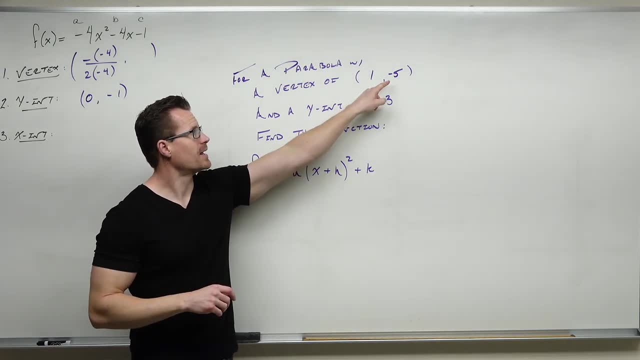 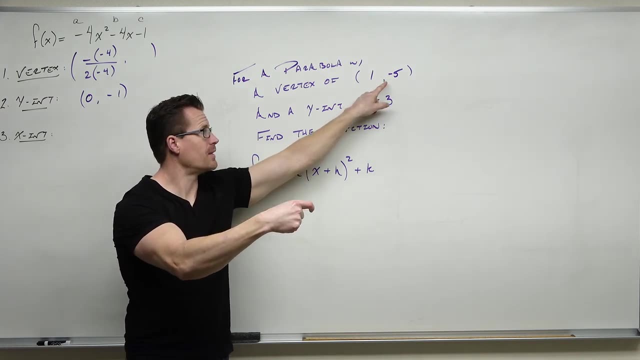 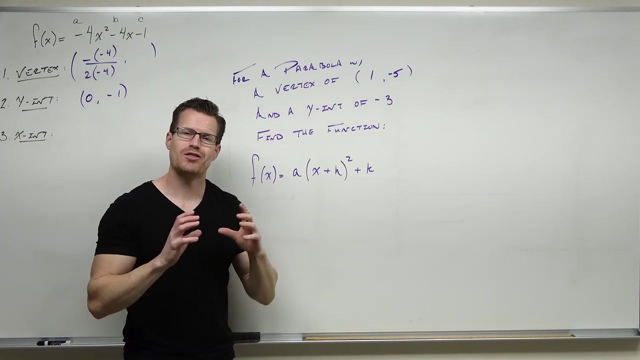 concerned. Think shifting, think transformations. Think that if I have a x-coordinate of one that's a shift right one, and this minus five would be a shift down five. This is a shift right one down five. Represent that first. Then what we do is use the fact that we have a function that's 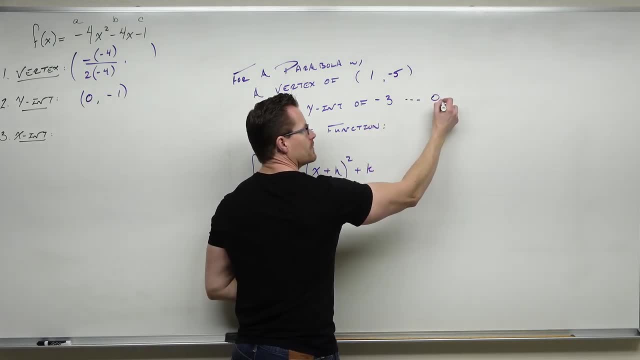 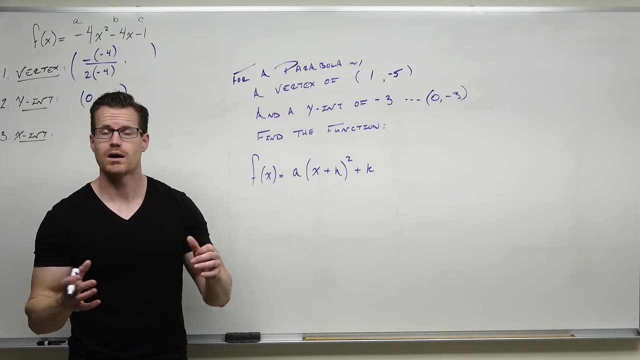 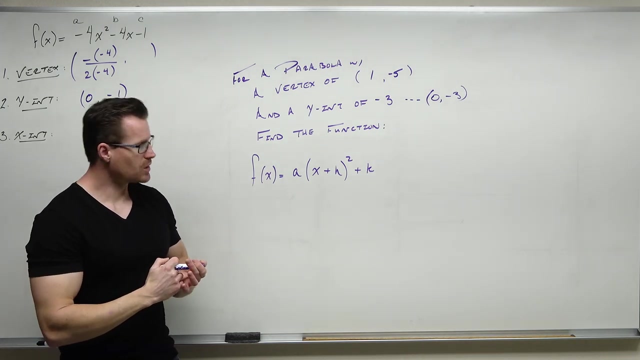 a y-intercept of negative three is zero comma negative three. That's a point. That's got to be a point. That's why we used points in everything we've done so far. Use that point to fill out what your a is going to be, And so I'm going to show you how to do that right now. So, if you have, 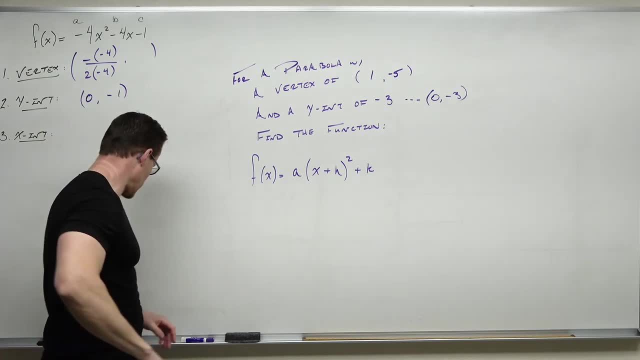 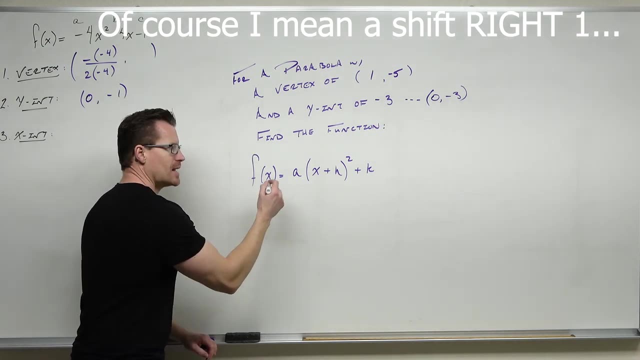 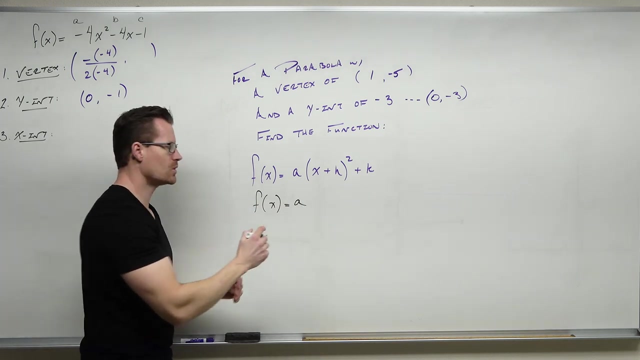 a vertex of one negative five and you go: well, listen, that one. that really means that we have a shift left one and we have a shift down five. Then, instead of having x plus h and this plus k, I know that this function is going to be something like this: A, I don't know. 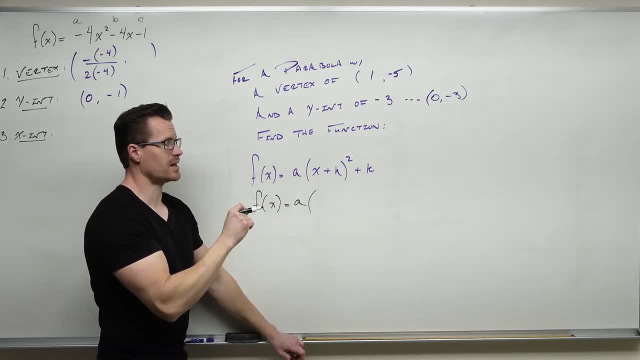 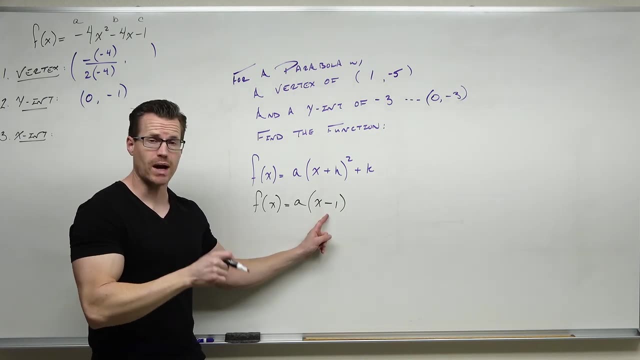 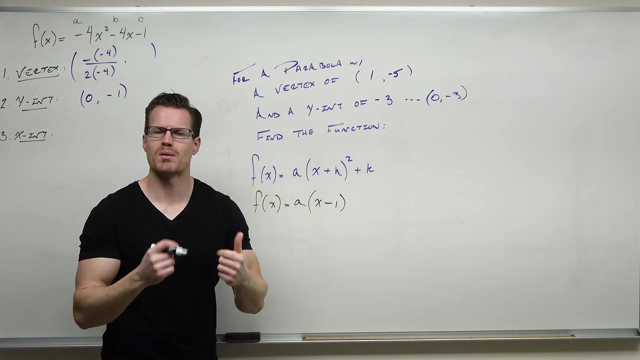 yet. but I know a shift left- I'm sorry, a shift right, I said left- A shift right one is x minus one. That represents a shift to the right of one unit. Since this vertex says: I shift right one and down five, that right one is a minus one. Do you remember that? Do you remember that everything? 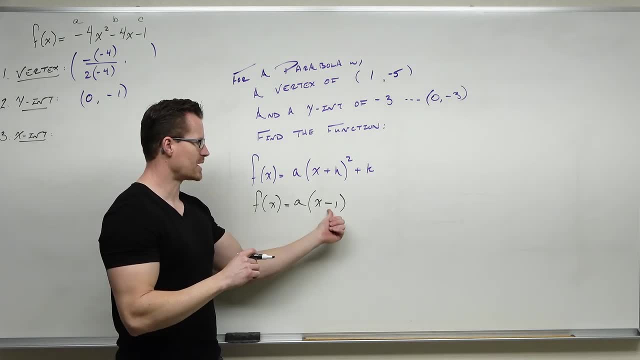 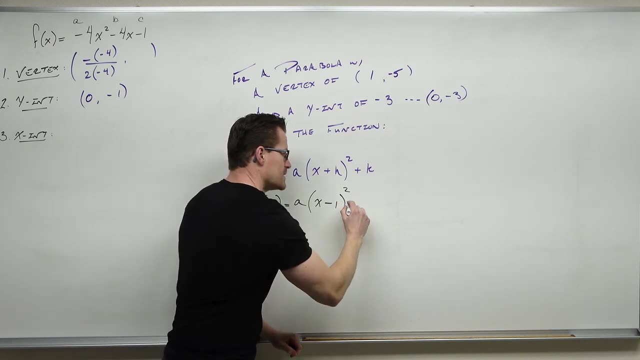 inside the parentheses is opposite of what you see. So if this is a minus one, this would be a shift to the right one. So if this is a minus one, this would be a shift to the right one, Representing that that value A shift. down five is a down five. We know that this would be a shift. 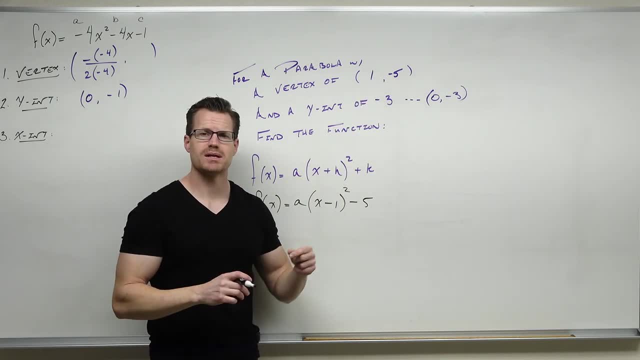 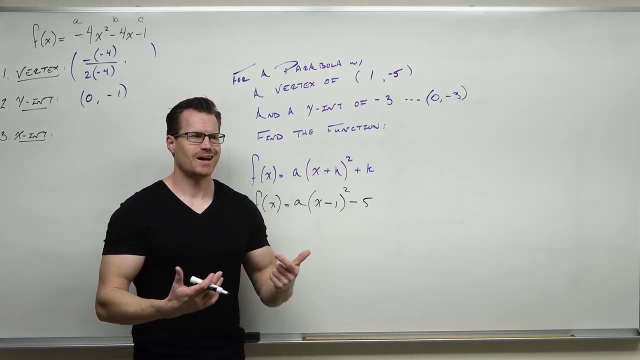 down five. Okay, that's what that means. This would be a shift right one. Okay, that's what that means. This is why this is called vertex form, because it models your vertex perfectly in your transformations. Of course, the issue is that I need to find what that A is. Well, your first step is: 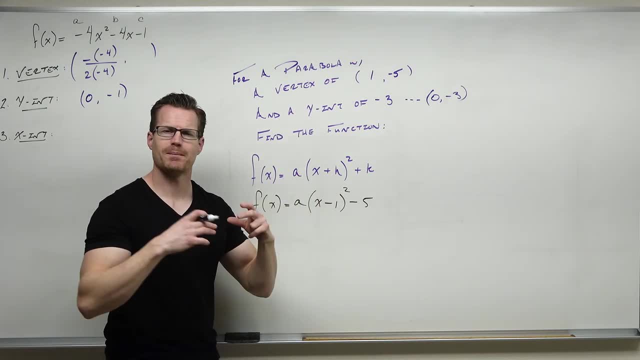 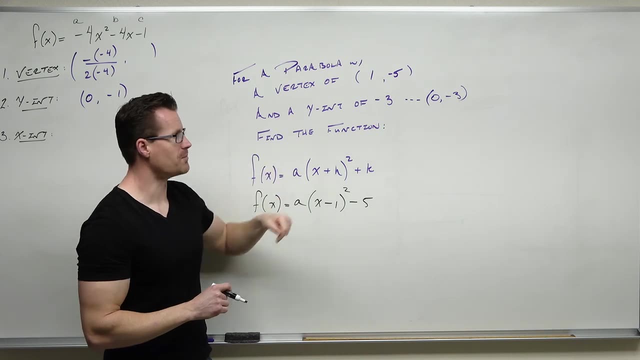 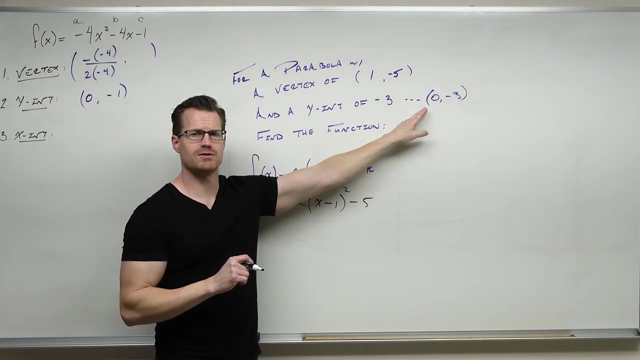 done. Your first step is use your vertex to fill out what you can, by understanding the transformations that are taking place, to get to obtain that vertex. Shift right minus one, Shift down minus five. Now we use this point that's given to you. Here's what this says: Your input is zero and it gives you. 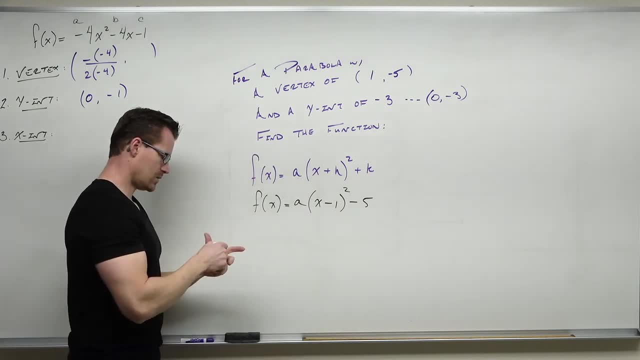 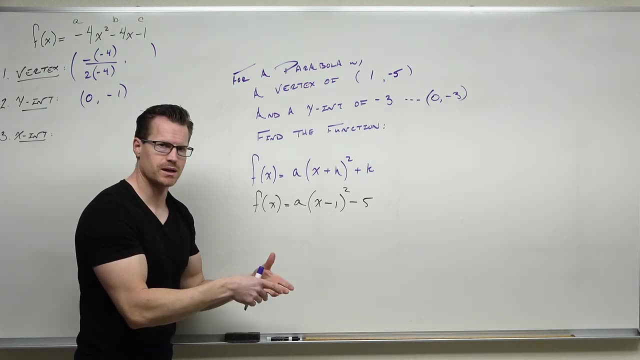 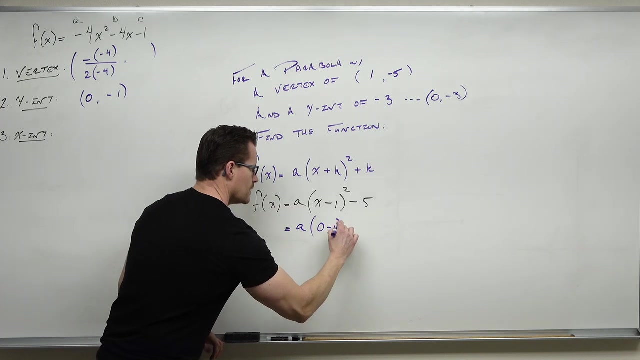 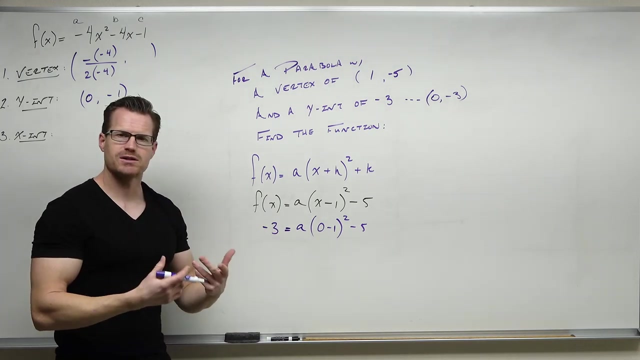 an output of negative three. Well, since your variable for your inputs is x and your variable for your outputs is f of x, plug in your point. Don't plug in for A. This says your input is zero. so replace the x with zero. Your output is negative three. Replace the f of x with negative. 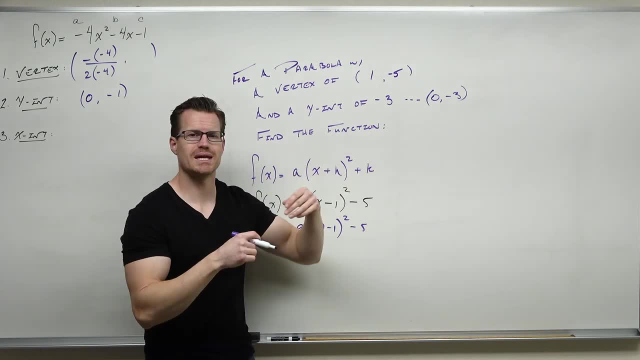 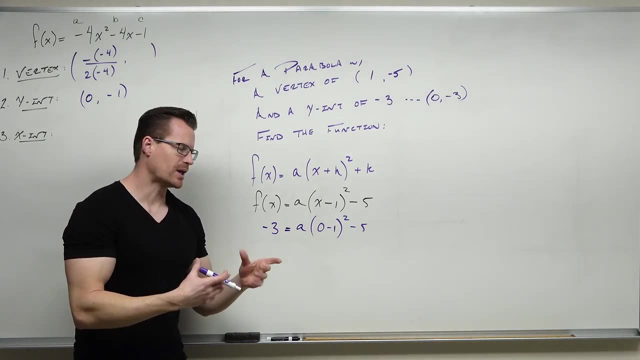 three. This is what this is saying to you. It's saying: if you plug in zero, you should get out an output of negative three. Hey, I plugged in zero, I should get an output of negative three. And now that we have that filled out, there's only one thing that we can do. We can solve for your A. 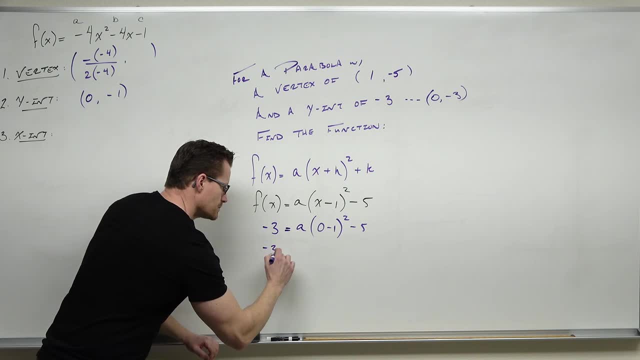 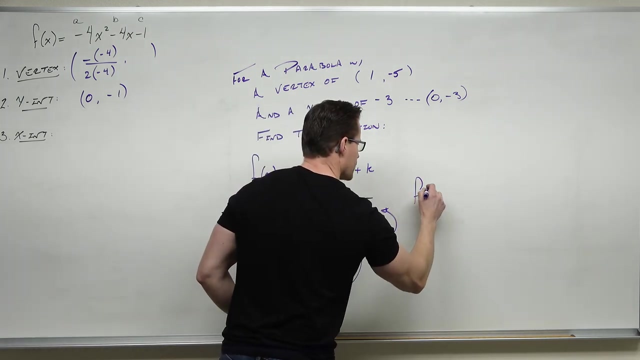 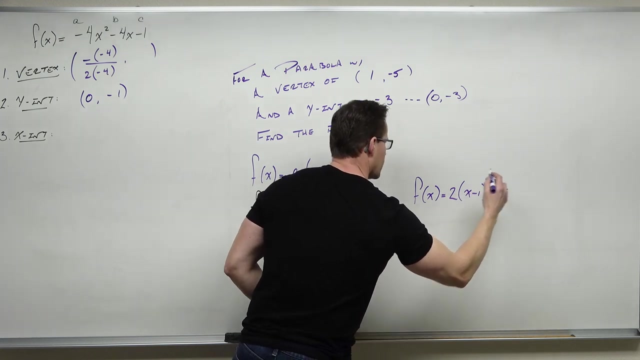 So by doing that, negative one squared is one. One times A is A. If I add five, then A is two. Come right back up here and just put that A in there and you've completed your function. That still has a vertex of: let's see right, one down five, That's here. This would still. 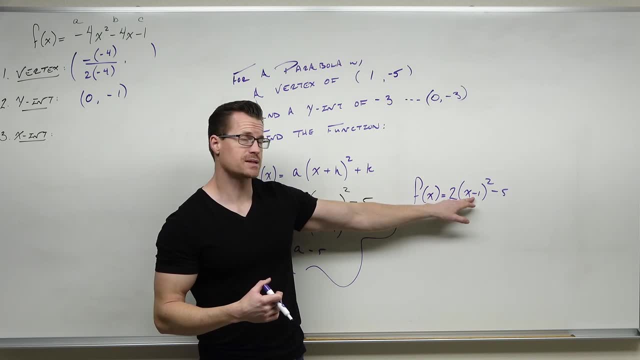 have a y intercept of zero three. Plug in zero if you want to. Zero minus one, That's negative one. squared is one. One times two is two Minus five is negative three. So I know that we're going to have a y intercept of zero three. So I know that actually works with the information. 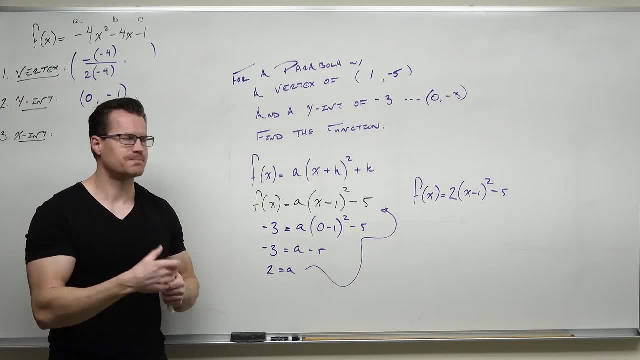 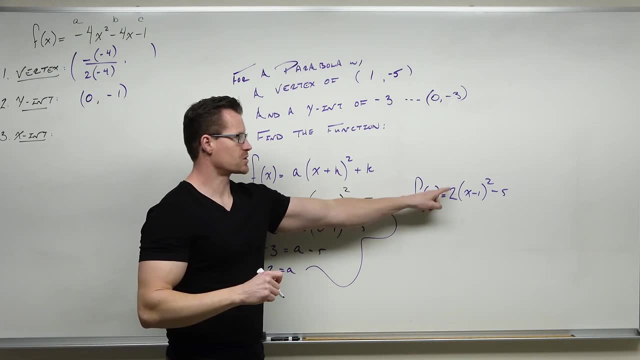 that's given to me And that's how to go from giving a point like a vertex and a y intercept, how to find a function from it. If you need to distribute it, you can certainly do that. So you distribute this x minus one squared first.